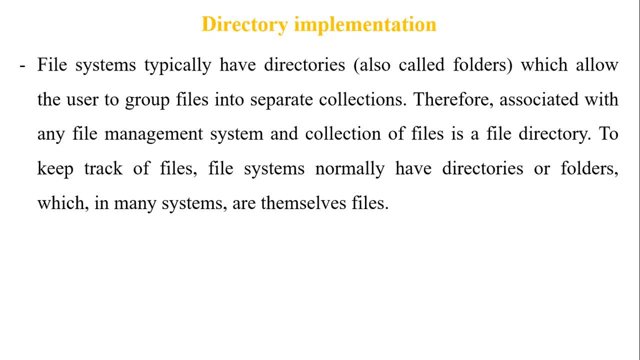 File systems typically have directories, also called folders, which allow the user to group files into separate collections. Therefore, associated with any file management system and the collection of files is a file directory To keep track of files. file systems normally have directories or folders, which, in many systems, are themselves files. 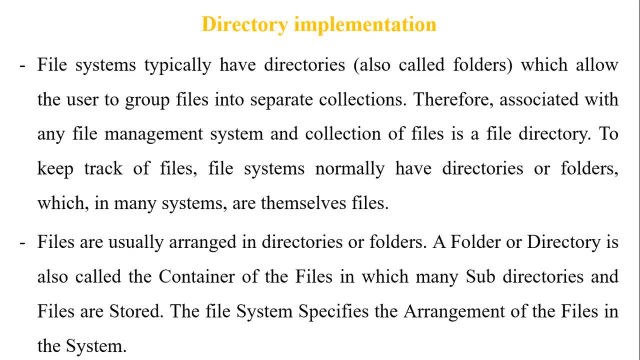 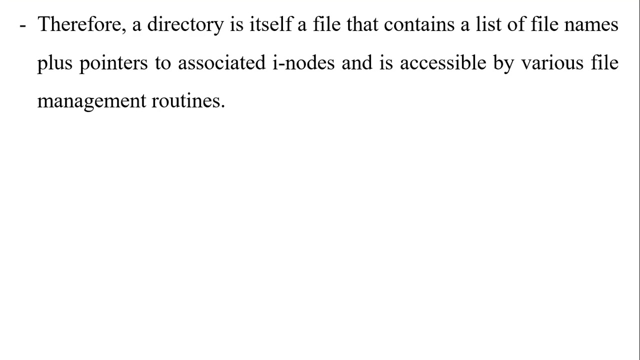 Files are usually arranged in directories or folders. A folder or a directory is also called the container of the files, in which many subdirectories and files are stored. The file system specifies the arrangement of the files in the system. Therefore, a directory is itself a file that contains a list of filenames plus pointers to associated items. 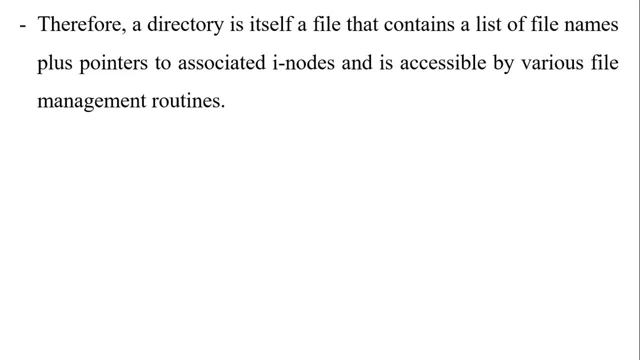 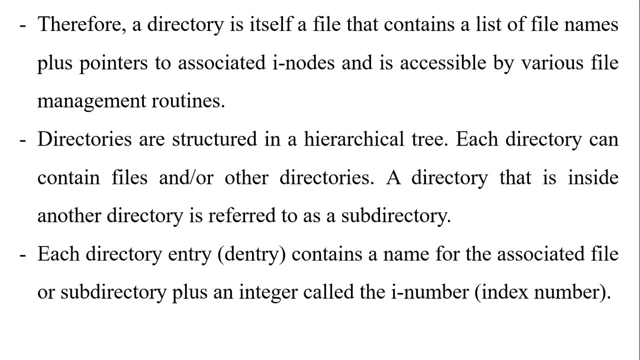 and is accessible by various file management routines. Directories are structured in a hierarchical tree. Each directory can contain files and or other directories. A directory that is inside another directory is called a subdirectory. Each directory ends up in a directory called a sub directory. 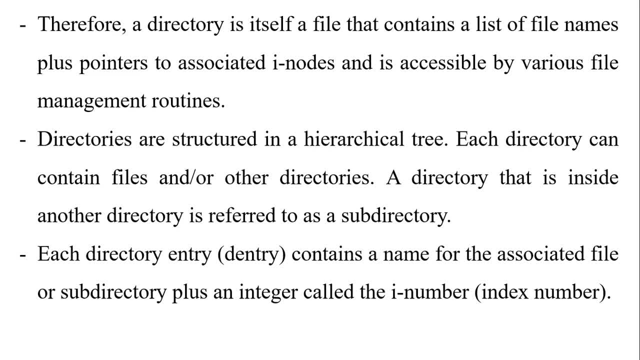 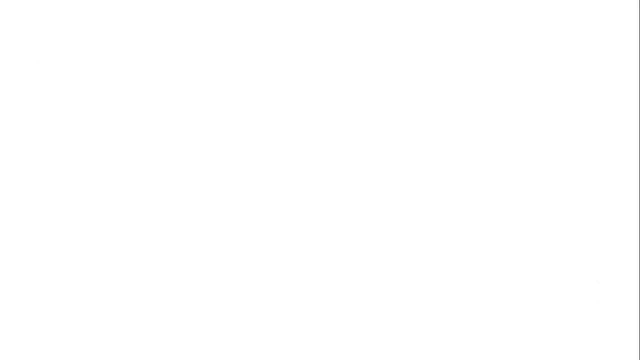 The sub-directory or the entry contains a name of the associated file or a subdirectory plus an integer that is called the INUMBER or INDEX NUMBER. When the file or a directory is accessed, its INUMBER is used as an INDEX into the INODE table. 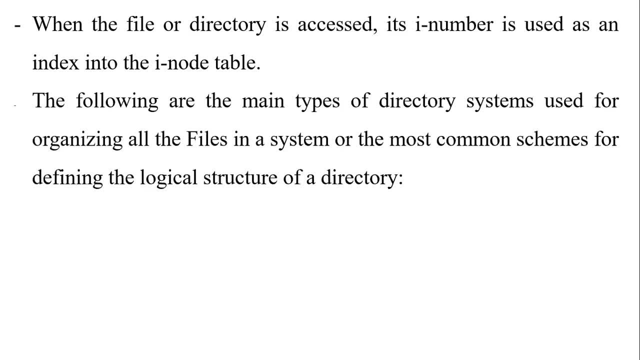 The following is an example of an INDEX INTO the INODE table. The following are the main types of directory systems that are used for organizing all the files in a system, or the most common schemes for defining the logical structure of a directory. Number one is what we call the single-level directory systems. 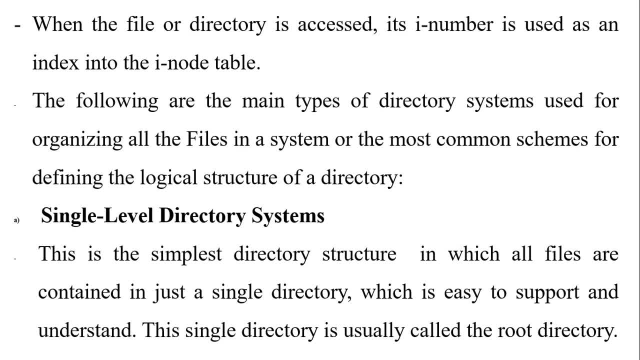 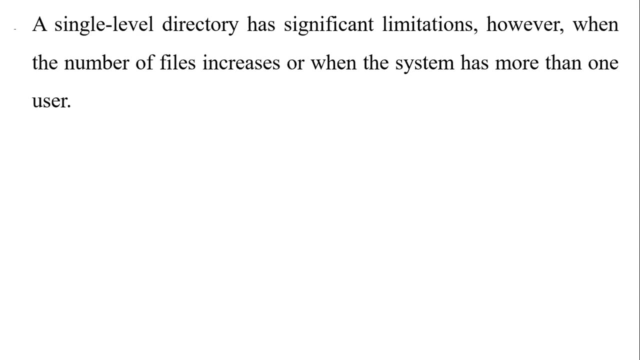 This is the simplest directory structure, in which all the files are contained in just a single directory, which is easy to support and understand. This single directory is usually called the root directory. A single-level directory has significant limitations, However, when the number of files is less than or equal to the number of files in the directory. 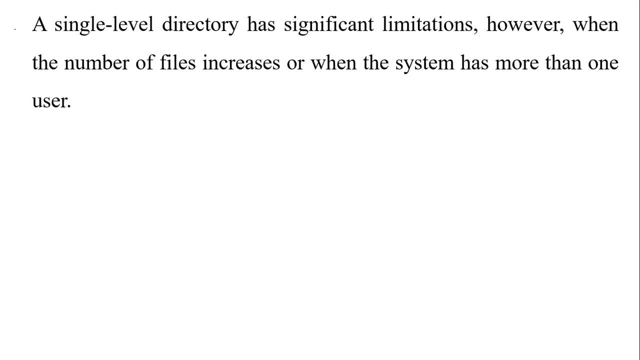 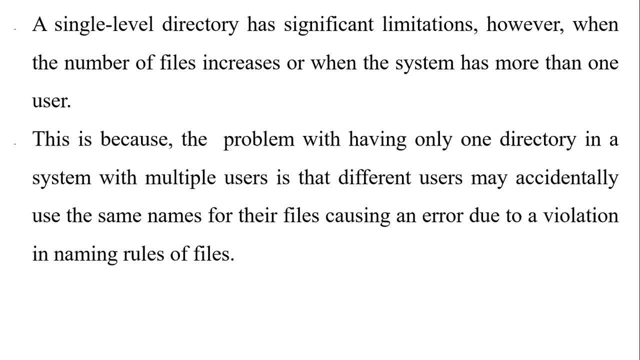 the number of files increases or when the system has more than one user. This is because the problem with having only one directory in a system with multiple users is that different users may accidentally use the same names for their files, thus causing an error due to evaluation. 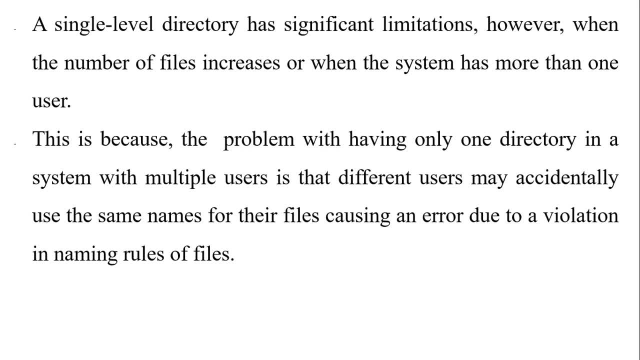 This is usually occurred only in一點. Indeed, the ng directories have a lot of markings in theirhd давай, horses, a variety of rounded flows with their libraries, But this noise or sound quality is not central to the use of thebsek. 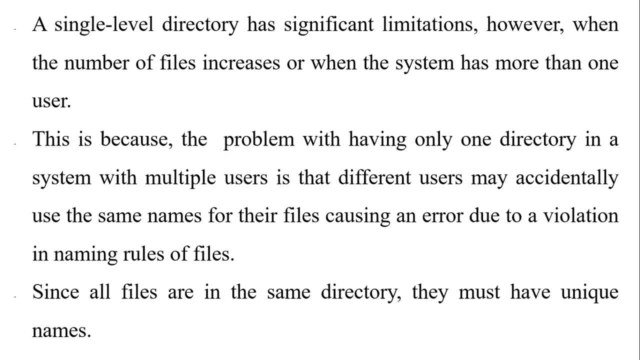 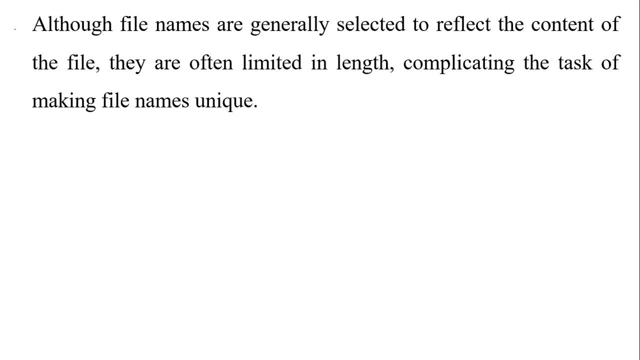 Itny name will non shouldn't affect theual typeface. Note that the true name is weak. Since all files are in the same directory, they must have unique names. Although file names are generally selected to reflect the content of the file, they are. 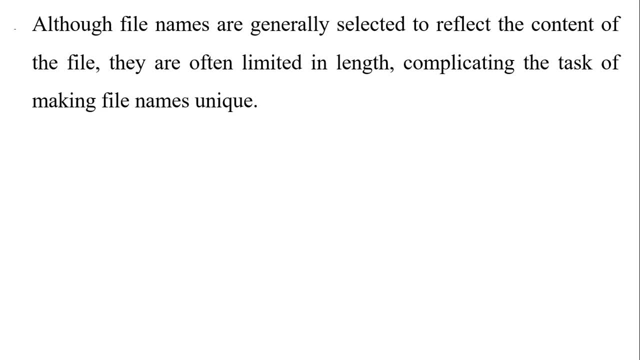 often limited in length, complicating the task of making file names unique. Regression data- Jewish trip in the want. Even a single user on a single level directory may find it difficult to remember the names of all the files as the number of files increase. 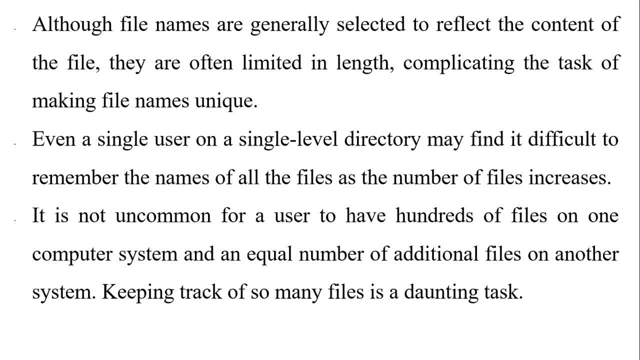 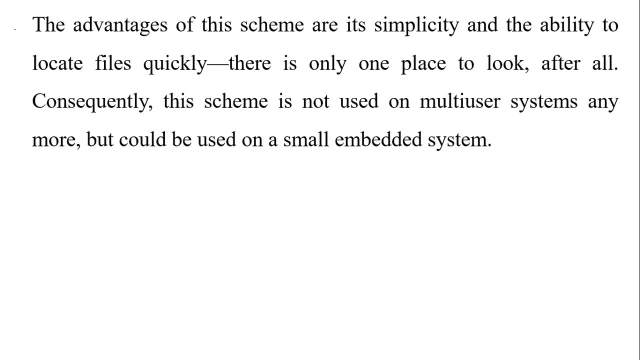 It is not uncommon for a user to have hundreds of files on one computer system and an equal number of additional files on another system. Therefore, keeping track of so many files is a daunting task. The advantages of this scheme are its simplicity and the ability to locate the files quickly. 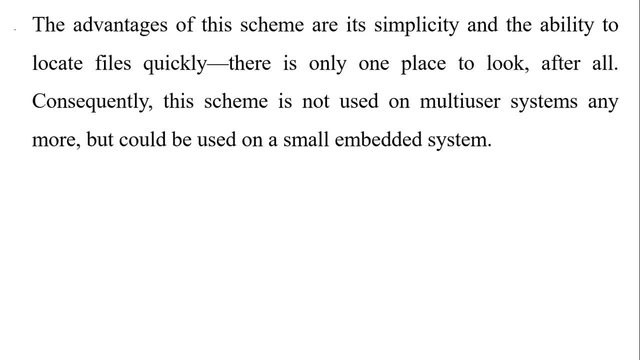 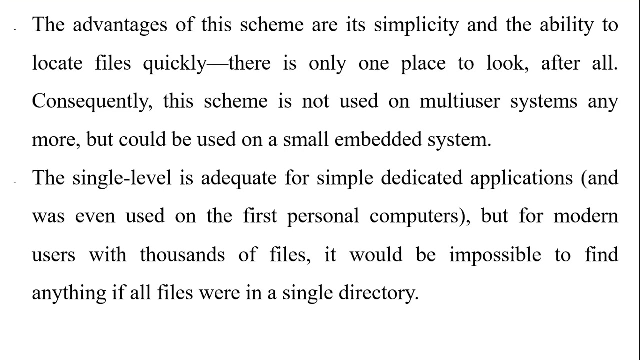 There is only one place to look after all. Consequently, this scheme is not used on multi-user systems anymore, But it could be used on a small abandoned system. The single level is adequate for simple dedicated applications and was even used on the first personal computers. 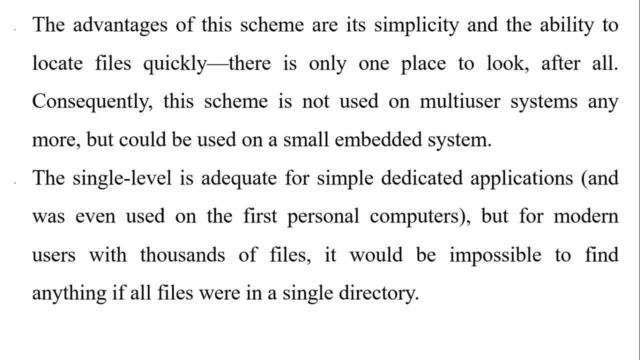 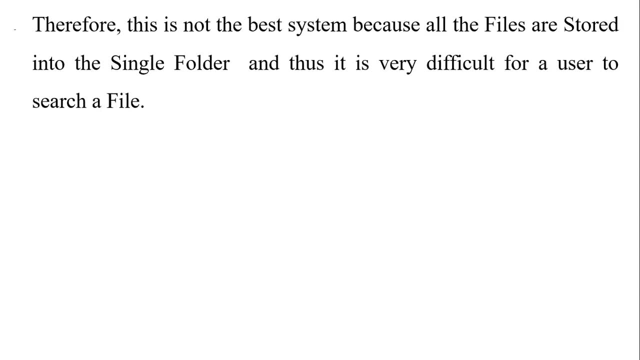 But for modern users without a sense of files, it would be impossible to find anything if all files were in a single directory. Thank you. Therefore, this is not the best system, because all the files are stored into a single folder, and thus it is very difficult for a user to search a file. 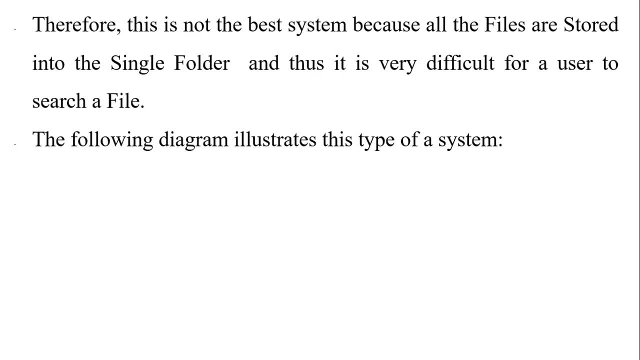 The following diagram illustrates this type of a system. From this diagram, My dear students and the rest of the learners, you can see that we have a root directory. A root directory is normally the storage location or the storage medium in which the files are. 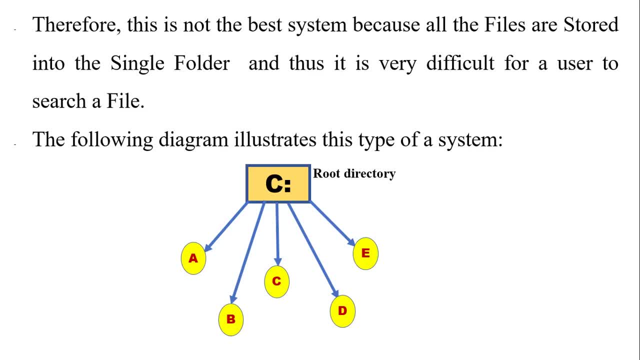 stored. For example, in this case our root directory is the hard disk, which is abbreviated in operating systems as C colon. If this computer contains a single hard disk or simply a single partition, Then inside that root directory or inside that storage medium we don't have any subdirectories. 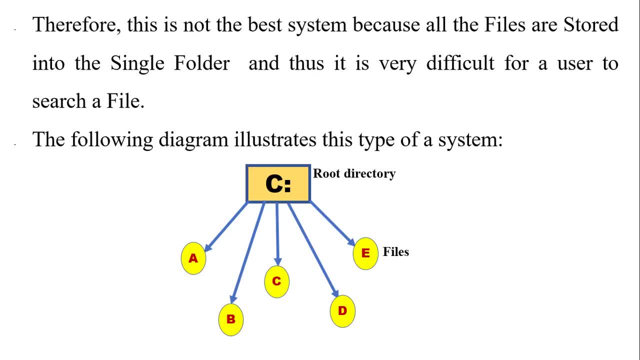 What we just have are files that are directly stored in the storage medium, And in this case we have files A and B. Now can we do this properly: B, C, D and E directly stored in a storage medium, without it being organized into folders or subdirectories? 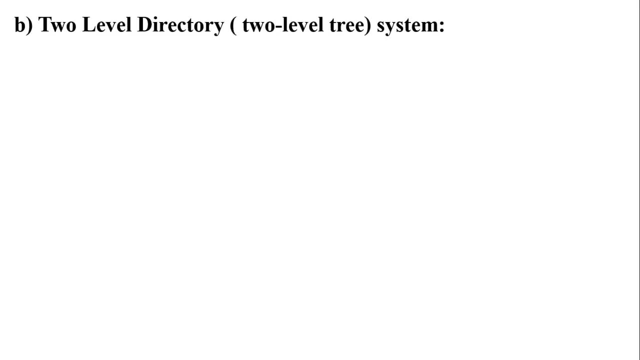 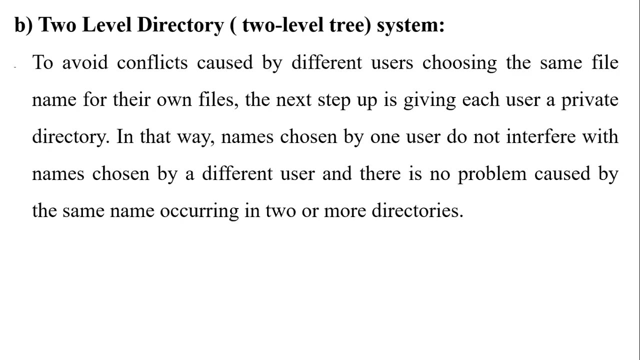 The second is what we call the two-level directory or two-level tree system, To avoid conflicts that are caused by different users choosing the same file name for their own files. the next step is to step up this method of storing by giving each user a private directory or a personal directory. 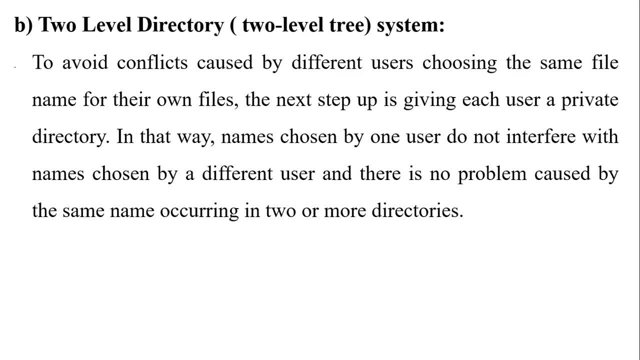 In that way, names chosen by one user do not interfere with the names chosen by another user And there is no problem caused by the same name occurring in two or more directories. Therefore, in order to avoid confusion of file names in a storage medium among different users, the standard solution is to create a separate directory for each user. 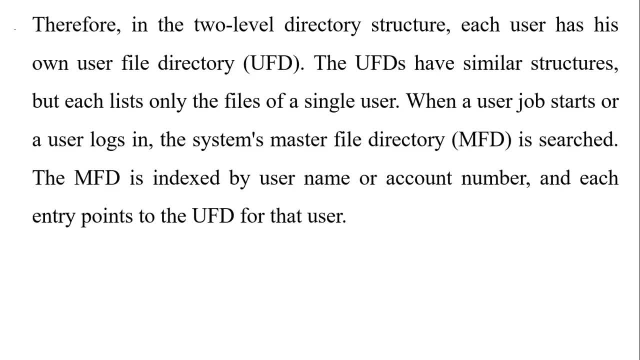 Therefore, in the two-level directory structure, each user has his or her own user directory, which we abbreviate as UFD, that is, User File Directory. The UFDs have similar structures, but each lists only the files of a single user. 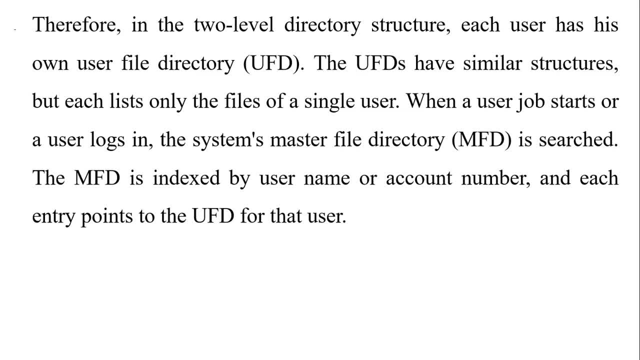 When a user's job starts or a user logs in, the system's master file directory, MFD, is searched. The MFD is indexed by username or account number and each entry points to the UFD for that user. When a user refers to a particular user, the MFD is indexed. 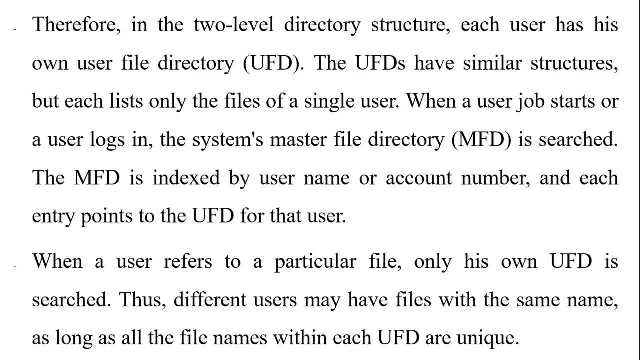 The MFD is indexed by username or account number, and each entry points to the UFD for that user. The MFD is indexed by username or account number. When a user finds a particular file, only his or her own UFD is searched. 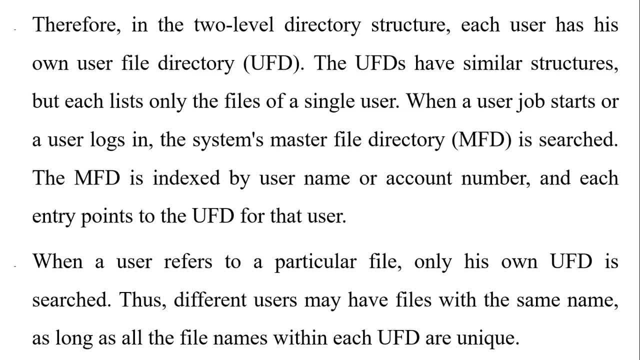 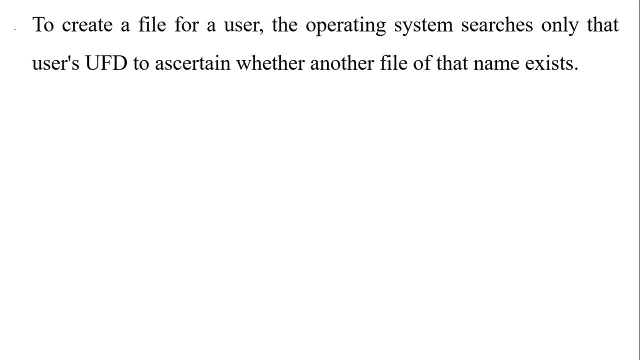 Thus different users may have files with the same name. as long as all the file names within each UFD are unique. To create a file for a user, the operating system searches only that file, Only that user's UFD, to ascertain whether another file of that name exists. 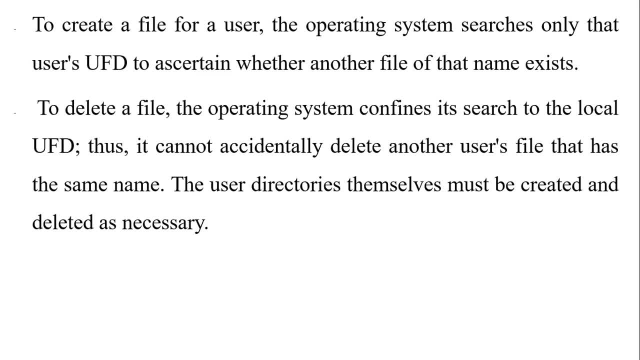 To delete a file. the operating system confines its search to the local UFD. Thus it cannot accidentally delete another user's file that has the same name. The user directories themselves must be created and deleted as necessary. The user directories themselves must be created and deleted as necessary. 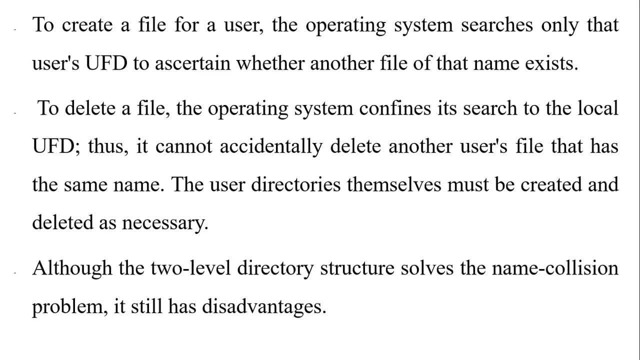 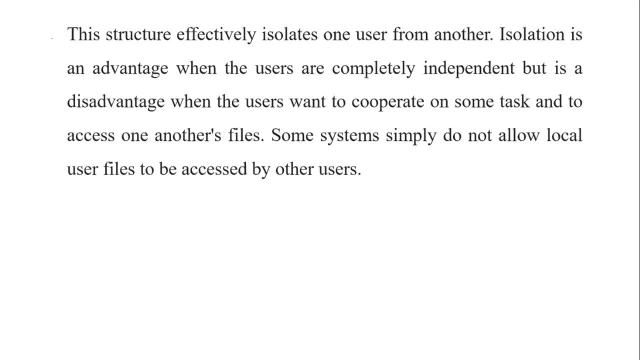 Although the two-level directory structure solves the name collation problem, it still has disadvantages. Although the two-level directory structure solves the name collation problem, it still has disadvantages. This structure effectively isolates one user from another. This structure effectively isolates one user from another. 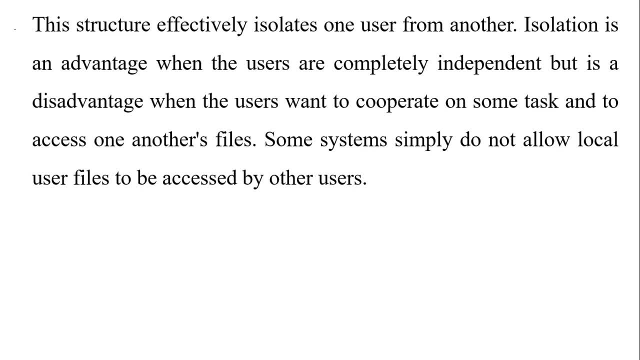 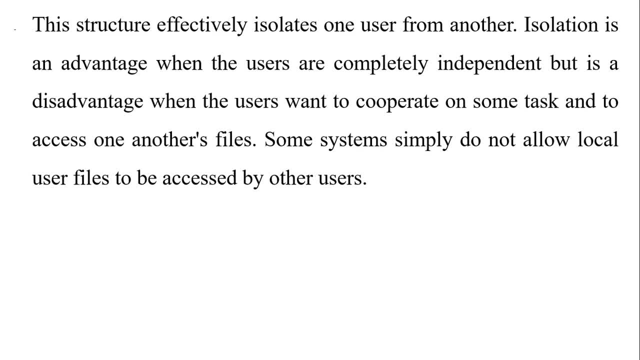 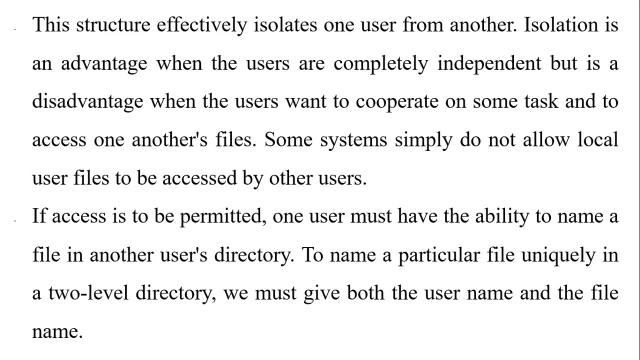 when the users want to cooperate on some task and to access one another's files. Some systems simply do not allow local user files to be accessed by other users. If access is to be permitted, one user must have the ability to name a file in another. 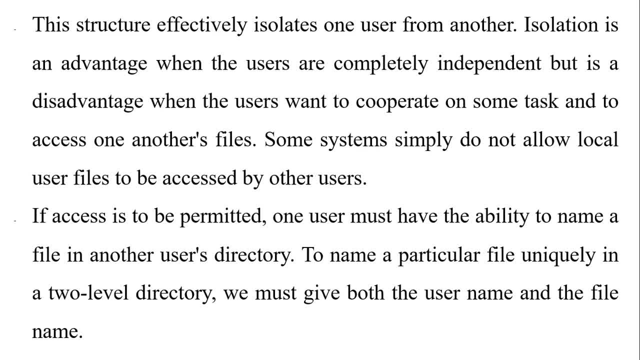 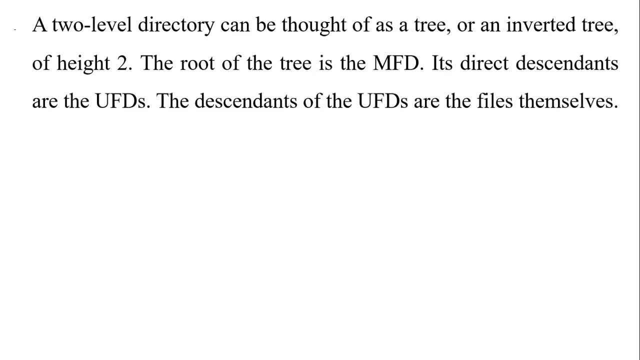 user's directory. To name a particular file uniquely. in a two-level directory we must give both the username and the filename. A two-level directory can be thought of as a tree or an inverted tree of height 2.. The root of the tree is the MFD. 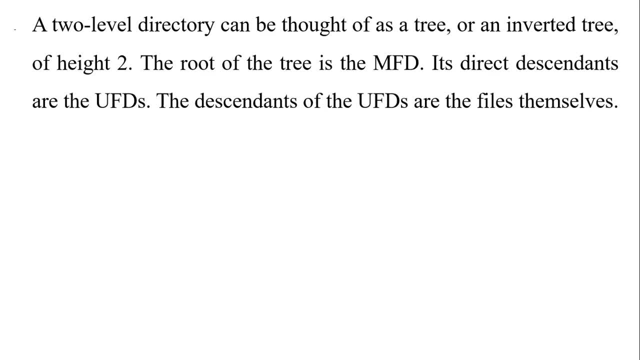 Its direct descendants are the UFDs. The descendants of the UFDs are the files themselves. MFD stands for master file directory, which we also call the root directory, And, just as I have said, it is usually the storage media or a partition that contains. 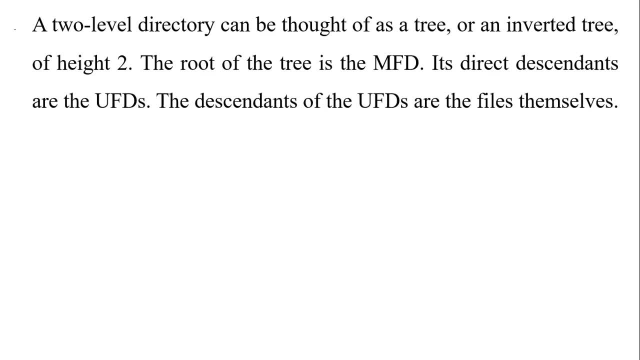 the directories, subdirectories or files, While the UFD stands for the user file directories, which can also be defined, too, as the user's subdirectories. The descendants of the UFDs are therefore the files themselves. This is because a user stores his or her files within his or her own directory. 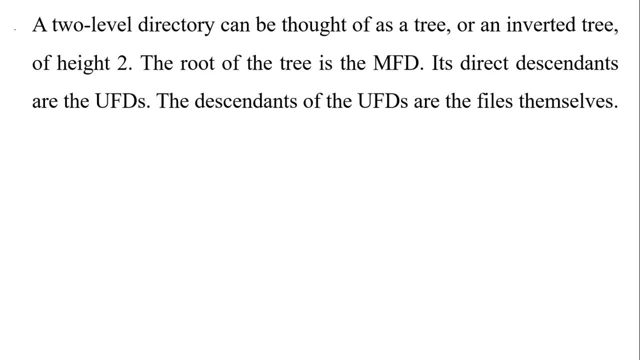 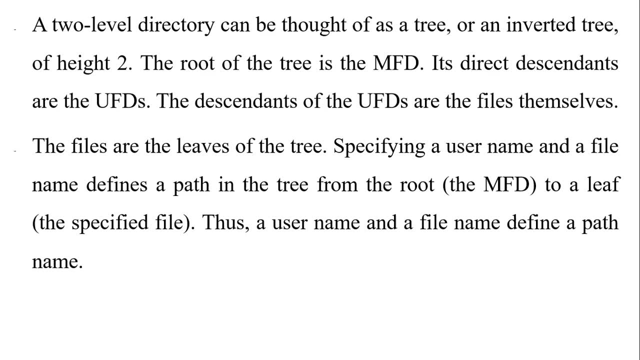 User file directory, or what we can call a sub-directory. The files are the leaves of the tree Specifying a username, and a filename defines a path in the tree from the root, that is the MFD, to a leaf that is the specified file. 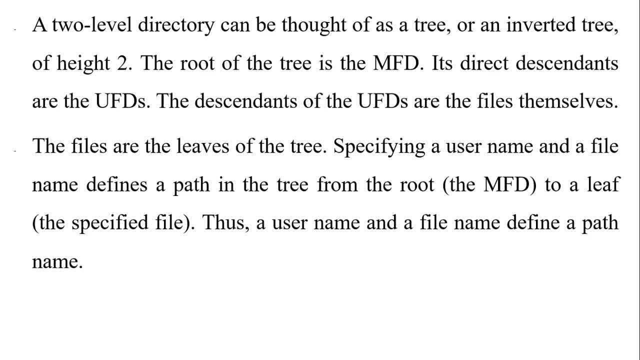 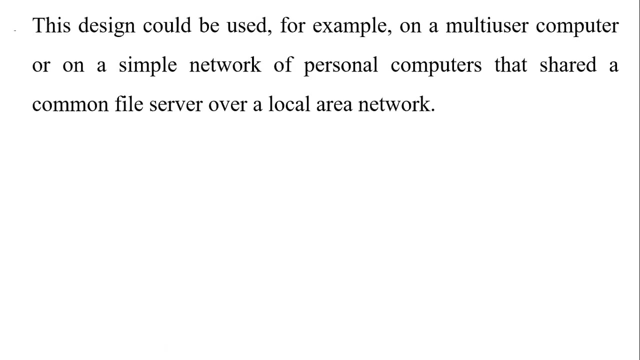 Therefore, a username and a filename define a path name. This is called the MFD. Every file in the system has a path name. To name a file uniquely, a user must know the path name of the file designed. This design could be used, for example, on a multi-user computer or a simple network. 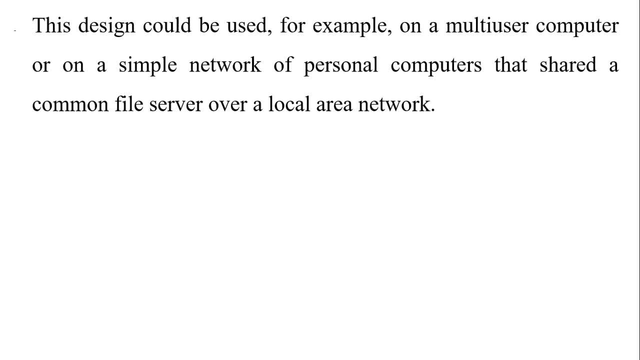 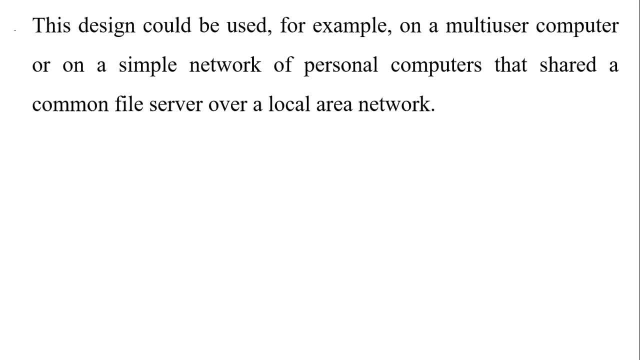 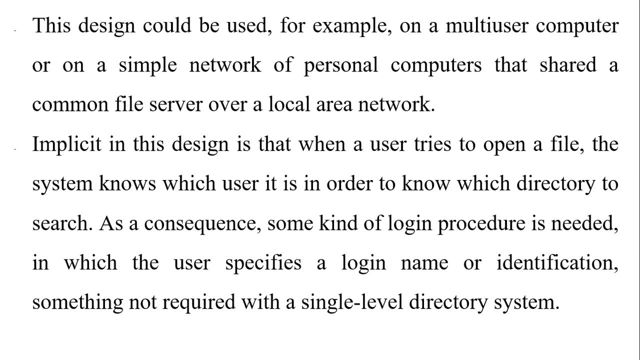 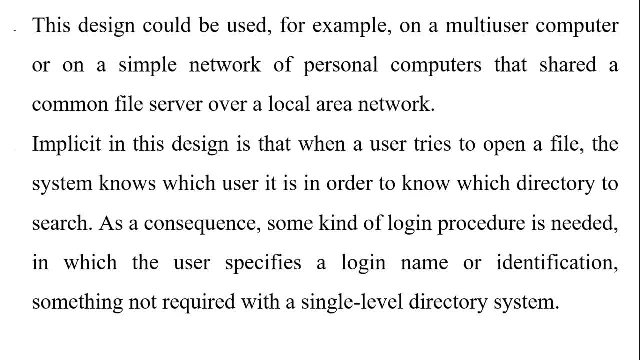 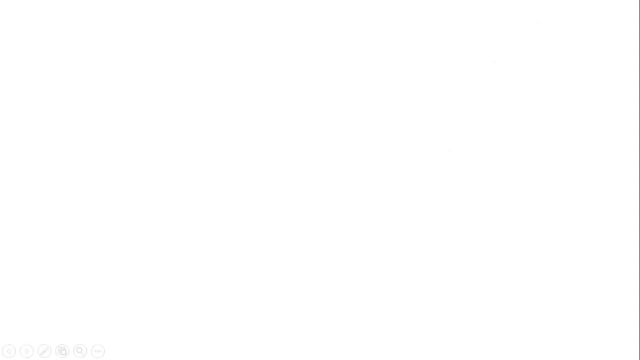 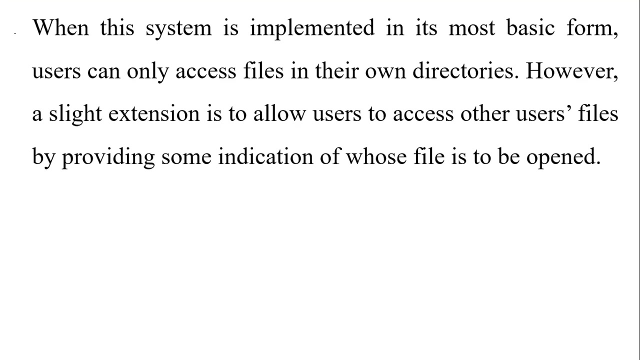 As a consequence, some kind of login procedure is needed in which the user specifies a login name or identification, something that is not required within a single level directory system. When this system is implemented in its most basic form, users can only access files in their own. 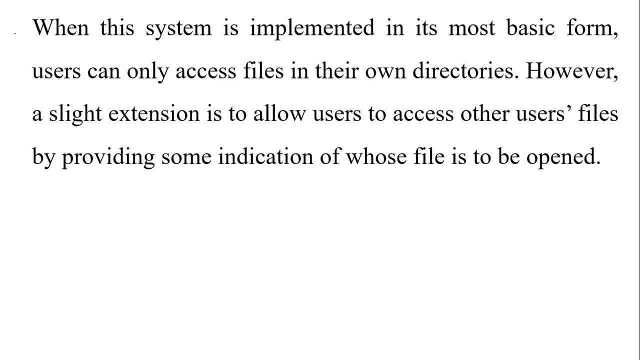 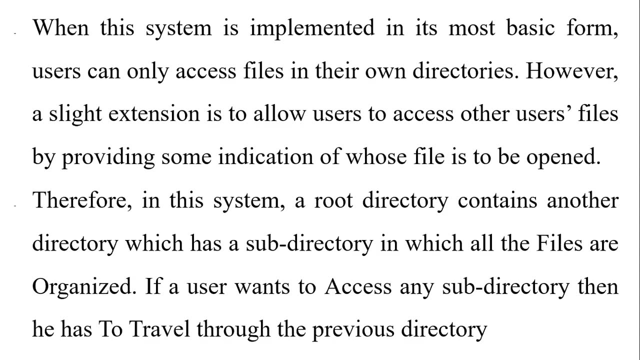 directories. However, a slight extension is to allow users to access other users' files by providing some indication of whose file is to be opened. Therefore, in this system, a root directory contains another directory which has a subdirectory in which all the files are organized, If a user wants to access. 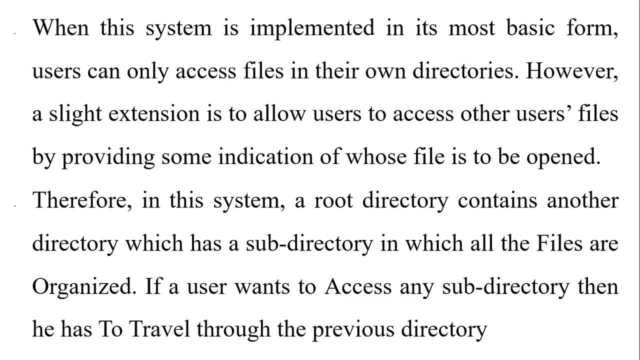 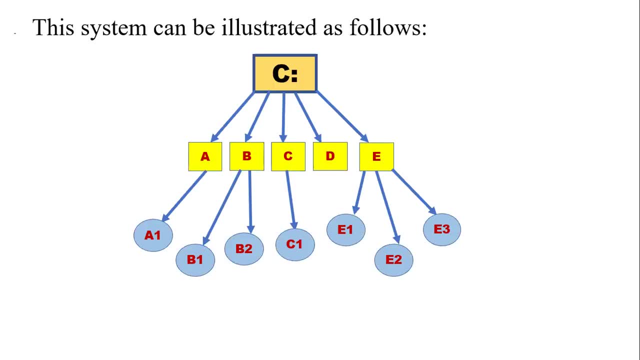 any subdirectory, then he or she has to travel through the previous directory. This system can be illustrated as follows: So in this case we have a root directory, which we also call the master file directory, And then in this root directory we have different directories for each user. 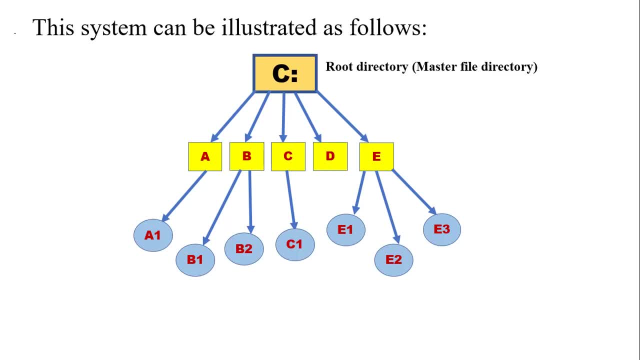 that are mostly accessible by the owners only, And this we call them the user file directories, And each individual user, for example user A, stores his or her own files within his or her own user file directory. These user file directories can even be called. 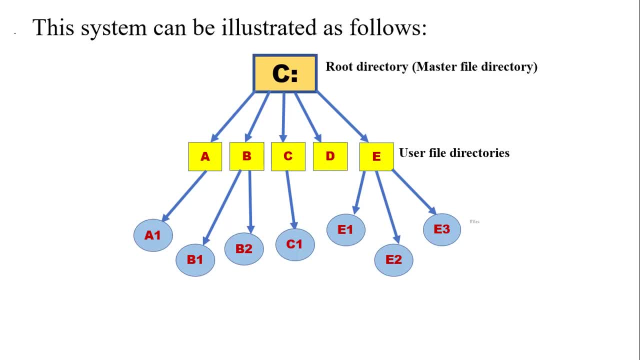 subdirectories in this context And therefore we have files. For example, in this situation or in this case, we have one single root directory, which we call the master file directory. that I have already said. it represents the storage media area for the files, And then we have several users, that is user A to user E. User A has a single file. 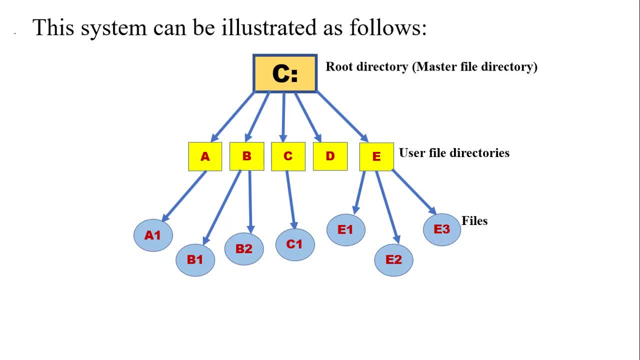 that is called A1.. User B has two files, in this case B1 and B2.. User C has a single file- C1,, while user D has a directory but which has no files, While user E has three files in his or her directory or subdirectory, which are file E1, E2, and E3. 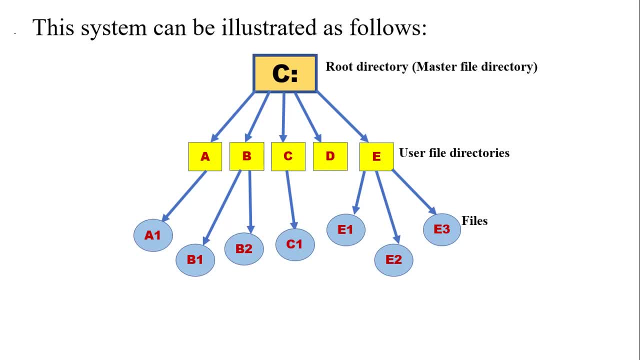 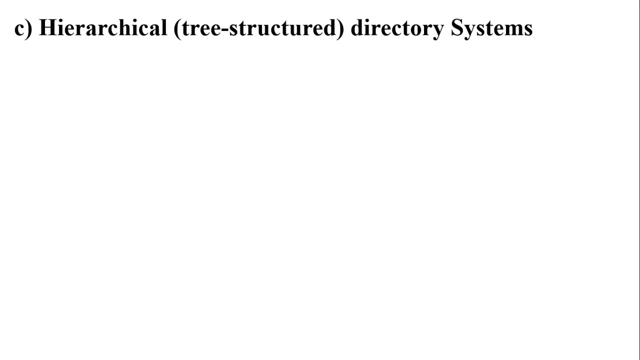 In this case, a user is only able to access or access his or her files only because he or she is only able to access his or her user file directory. The valid type of directory system is what we call the hierarchical or subdirectory. This is usually an extension of the two-level directory to a tree of arbitrary height. 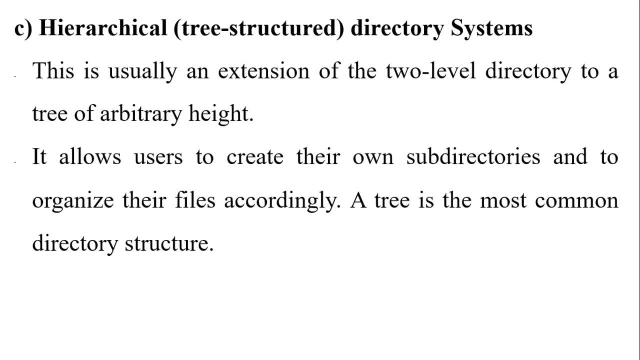 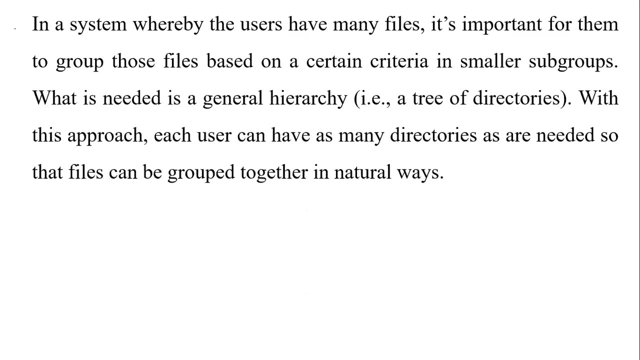 It allows users to create their own subdirectories and organize their files accordingly. A tree is the most common directory structure. The tree has a root directory And every file in the system has a unique path name. In a system whereby the users have many files, it is important for them to group those files, based on a certain criteria, in small subgroups. 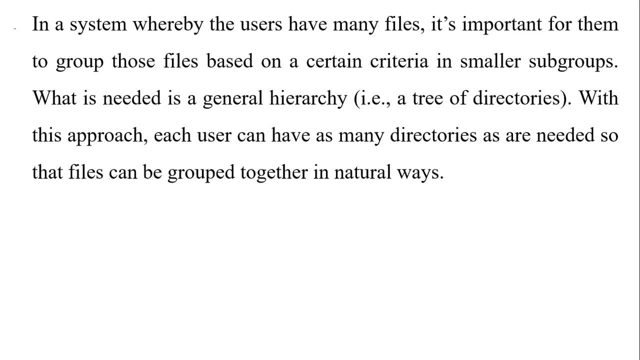 What is needed is a general hierarchy, That is what we call a tree of directories. With this, we can create a tree of subdirectories. With this approach, each user can have as many directories as are needed, so that the files can be grouped together in natural ways. 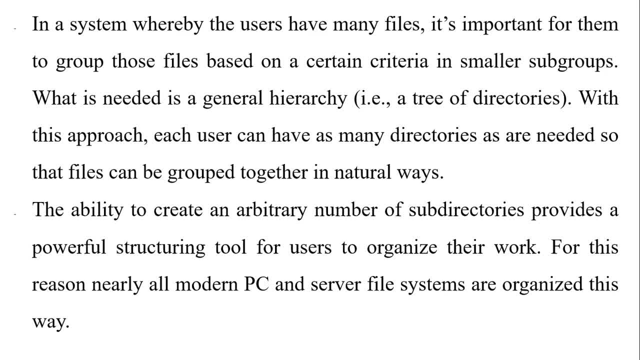 The ability to create an arbitrary number of subdirectories provides a powerful structuring tool for users to organize their work. For this reason, nearly all modern PCs and server file systems are built on a tree of directories. It is important to know that they are organized in this manner. 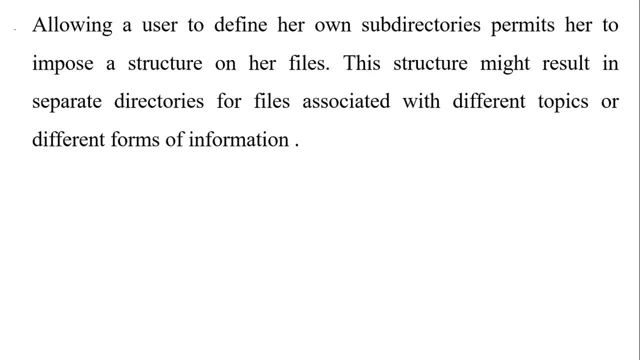 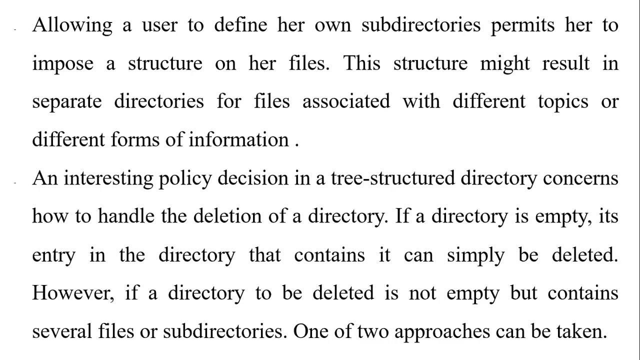 Allowing a user to define her own or his own directories or subdirectories permits him or her to impose a structure on his or her files. This structure might result in separate directories for files associated with different topics or different forms of information. An interesting policy decision in a tree structure directory concerns how to handle the deletion. 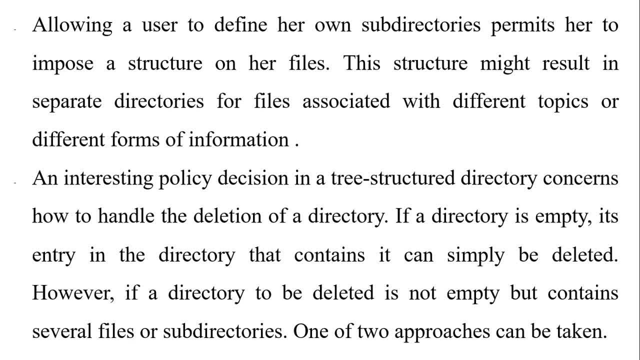 of a directory. If a directory is empty, its entry in the directory that contains it can simply be deleted. However, if a directory to be deleted is not empty but it contains several files or subdirectories, one or two approaches can be taken. 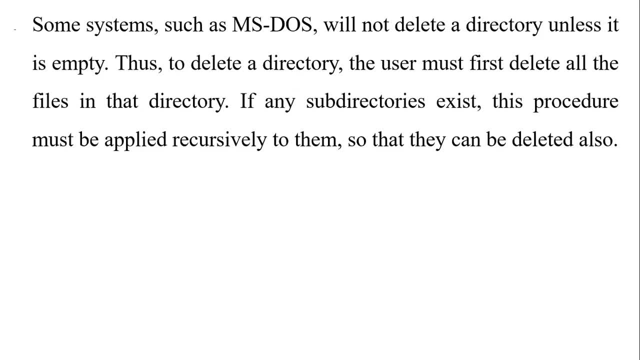 Some systems, such as MS-DOS, will not delete a directory unless it is empty, and therefore to delete such a directory, the user must first delete all the files in that directory. If any subdirectories exist, this procedure must be applied recursively. 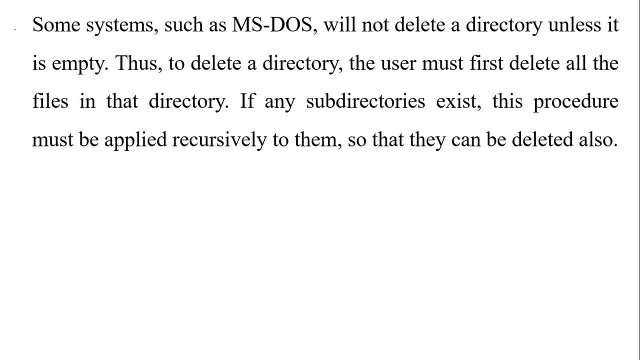 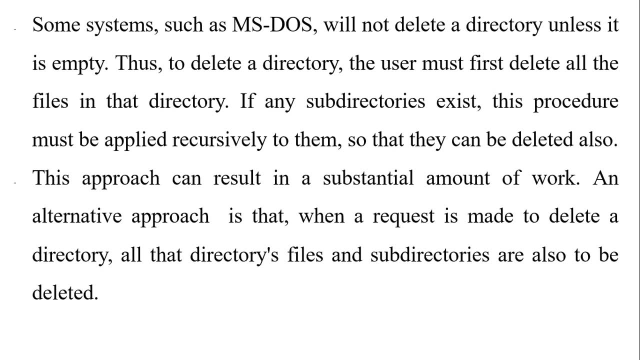 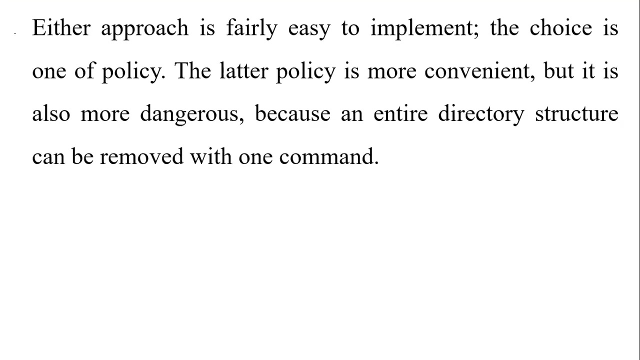 This approach can result in a substantial amount of work. An alternative approach is that when a request is made to delete a directory, all that directory's files and subdirectories are also to be deleted. Aether approach is fairly easy to implement. The choice is one of policy. 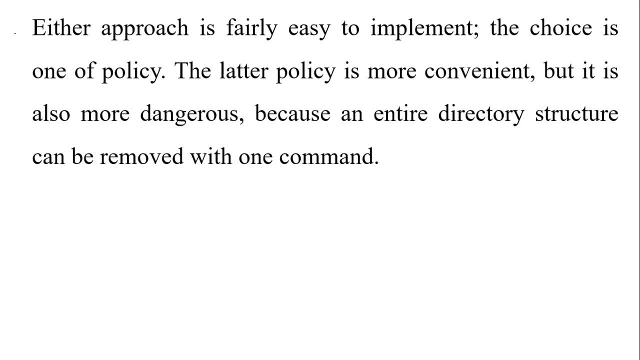 The latter policy is more convenient, but it is also more dangerous, because an entire directory structure can be removed with one command. If that command is issued in error, a large number of files and directories will need to be reset, And if a request is turned on, the user must return the file to the directory. assuming 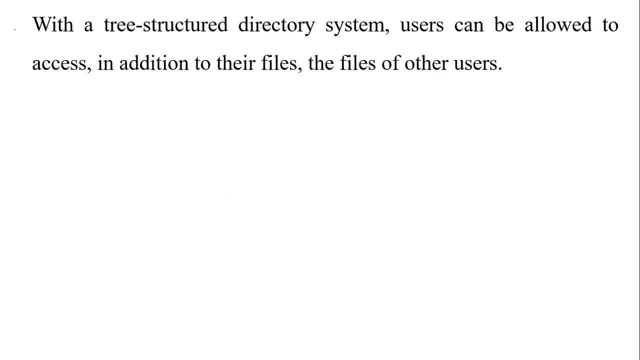 a backup exists. With a tree structure directory, system users can be allowed to access, in addition to their files, the files of other users. A path to a file in a tree structure directory can be longer than a path in a 2-level directory. 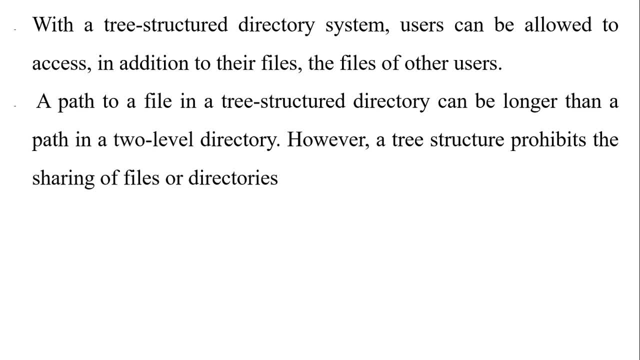 3.. However, a tree structure prohibits the sharing of files or directories. Therefore, in this system, all the files are organized in the form of parent and child relationship. This means that there is a parent directory which contains all the subdirectories. 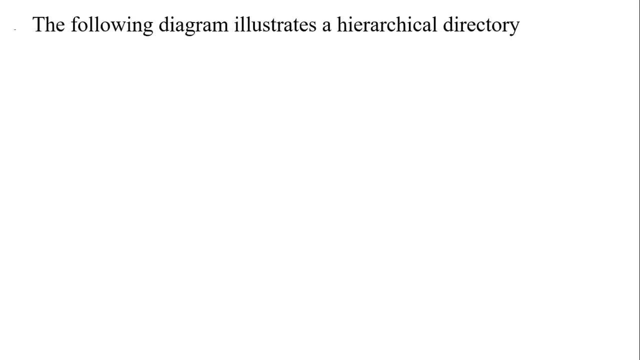 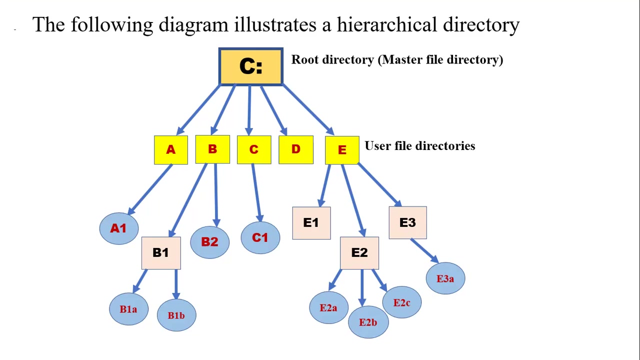 The following diagram illustrates a hierarchical directory, Just as it is in the other hierarchies or directory systems that we have looked at. in this system we also have a root directory, which we also call the master file directory, And then we have the user file directories, whereby each directory or subdirectory has its own directory. 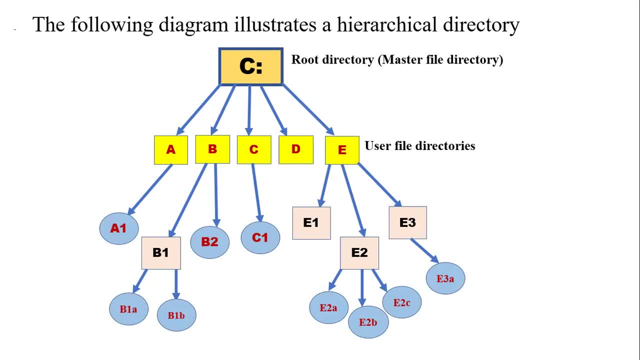 Each directory contains a single user's files Under the directory or under each user directory. we can have a file, like it is for a user, with having the user file directory A and C. In this case, A and C contains a single file each. 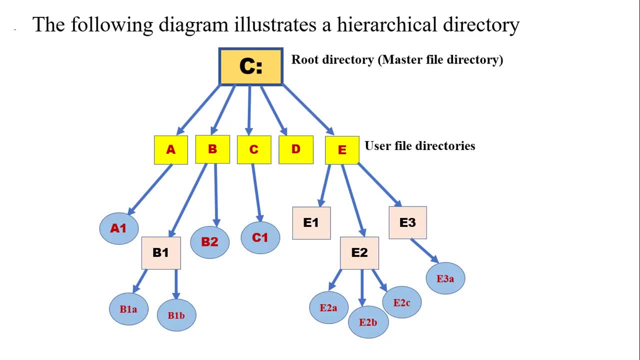 while D has a directory that does not contain any content. However, the user file directory for user B also contains another subdirectory, which is B1. And therefore, in this case, under this subdirectory B1, we have two files: file B1A and B1B. 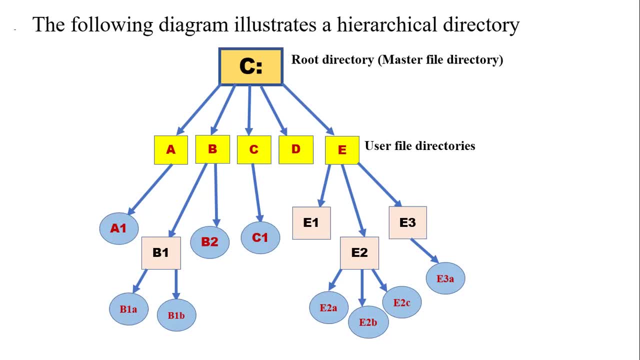 While at the same level we have another file, B2, which does not belong in a subdirectory, but it is directly placed under the user file directory. On the other hand, the user file directory E contains three further subdirectories, which are E1, E2, and E3. 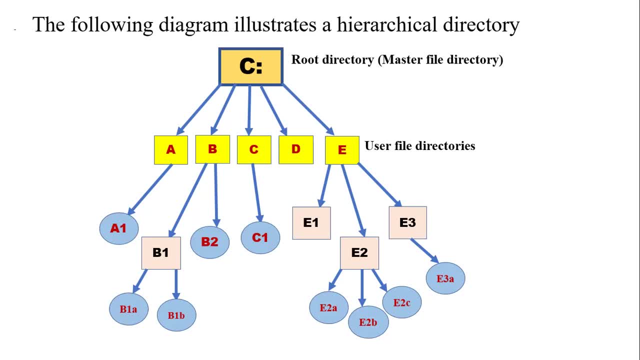 The E1 subdirectory does not contain any files, but E2 contains three files, while E3 contains a single file, And therefore this organization indicates an inverted tree where the root directory is the storage media, in this case is the hand disk. 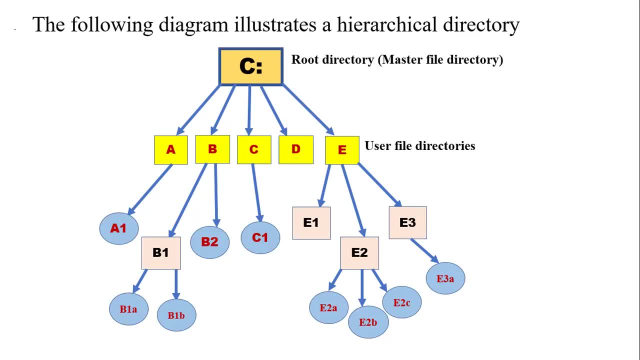 And then we have user directories or user file directories, under which we can have additional subdirectories, with each subdirectory being organized to contain a certain type of files. So that is the hierarchy directory, or hierarchical directory, where on topmost we have the root directory or the master file directory. 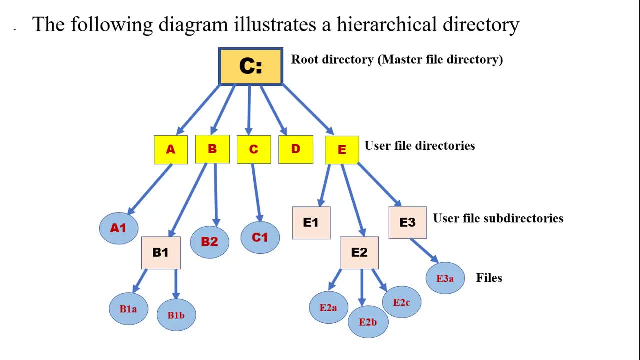 below which we have, or in which we have, five user file directories, And under these user file directories we have users creating subdirectories, And in this case we can see that user B has one subdirectory, while user E has three subdirectories. 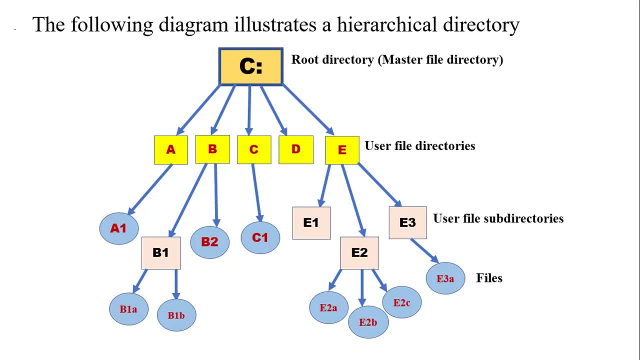 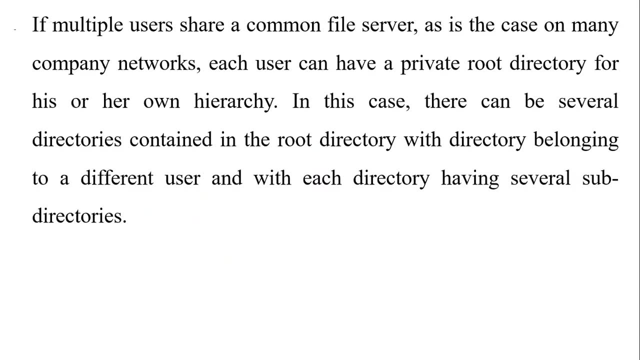 which we also call the user file subdirectories, And then under each of them we can have files. If multiple users share a common file server, as is in the case on many company networks, each user can have a private root directory for his or her own hierarchy. 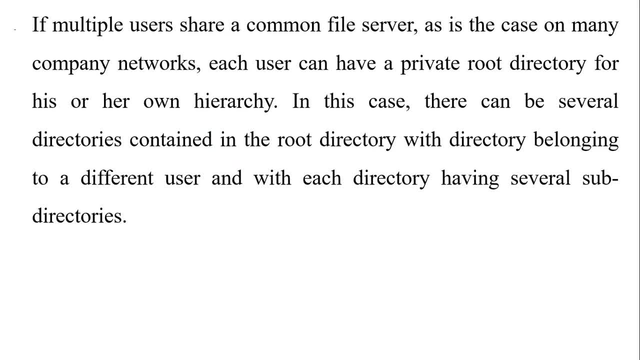 In this case, there can be several directories contained in the root directory, with the directory belonging to a different user and with each directory having several subdirectories. When the file system is organized as a directory tree, some way is needed for specifying the file names. 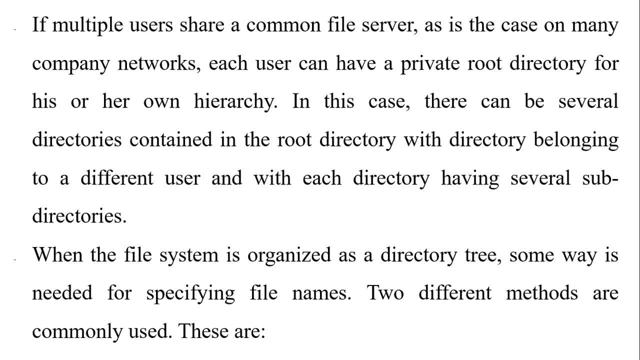 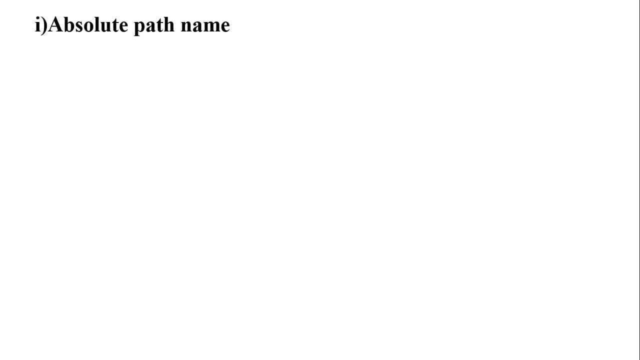 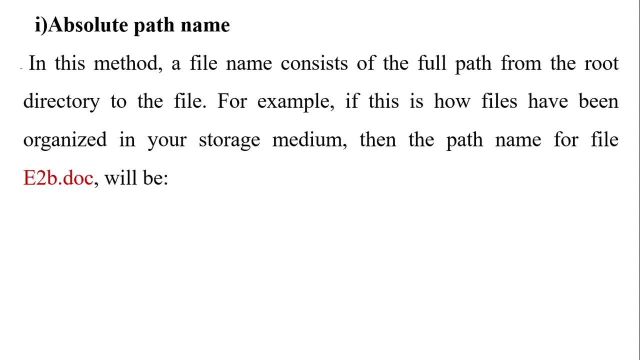 The two different methods that are commonly used are. Number one is what we call the absolute path name. In this method, a file name consists of the full path from the root directory to the file. For example, if this is how files have been organized in your storage medium: 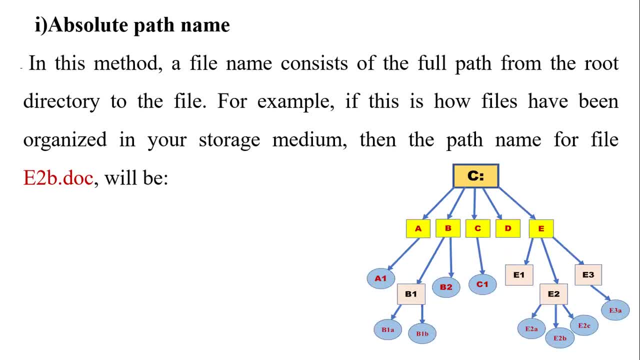 then the path name for file e2bdoc will be C colon, backslash e, backslash e2, backslash e2bdoc. in Windows operating systems, While it will be for one slash e, for one slash e2, for one slash e2bdoc. 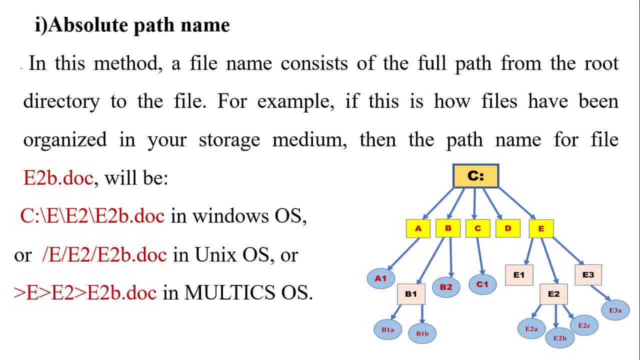 in Unix operating systems, or greater than sign e, greater than sign e2, greater than sign e2bdoc in Multics operating systems. My dear students and the rest of the learners, what you need to note is that when we are referring to a file based on absolute path name, 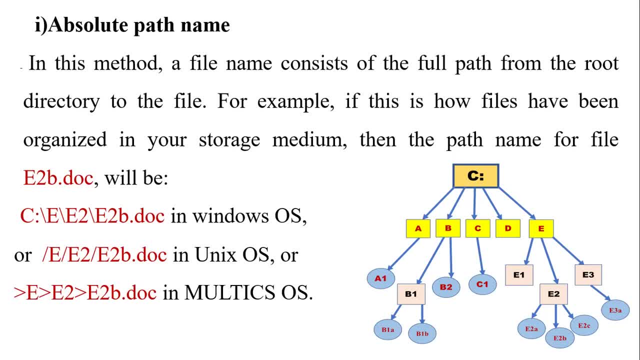 we give the entire path from the root to the file. As you can see in these examples, like in Windows, we have C colon, which is the root directory, And then we have e, which is the first user file directory, And e we have. 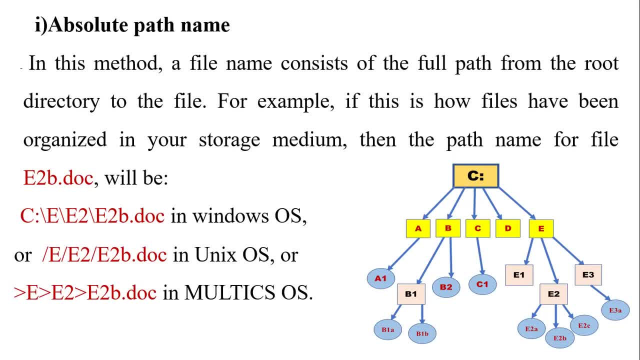 three subdirectories And in this case the subdirectory that contains our file is e2.. So we have e2 user subdirectory And under e2 user subdirectory we have the file that we are referring to, which is a documented file- e2b. 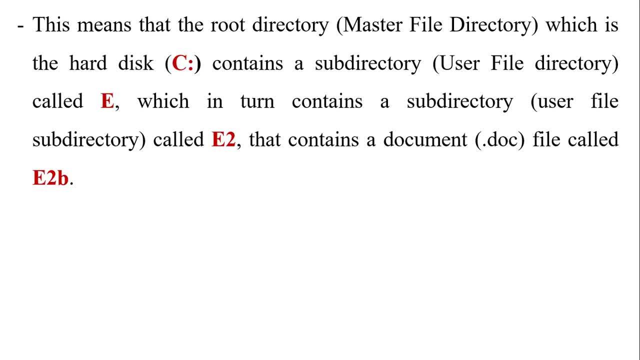 This means that, just as I have explained that the root directory or master file directory, which is the hand disk C colon, contains a subdirectory or user file directory called e, which in turn contains a subdirectory or a user file subdirectory. 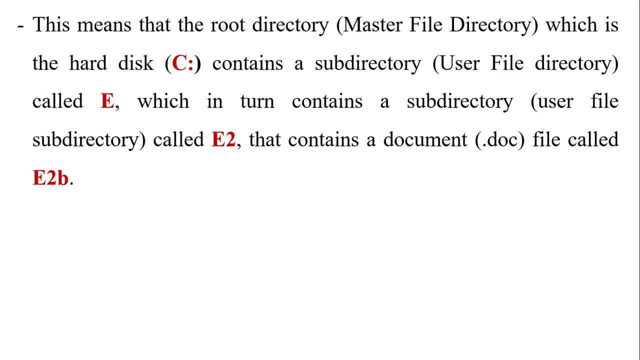 that is called e2, which contains a documented file by the name e2b. e2bdoc simply means that e2b is a documented file. To learn more about these extensions like e2bdoc, e2btxt and others. 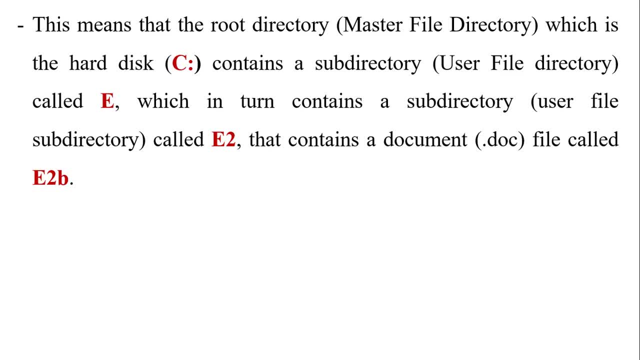 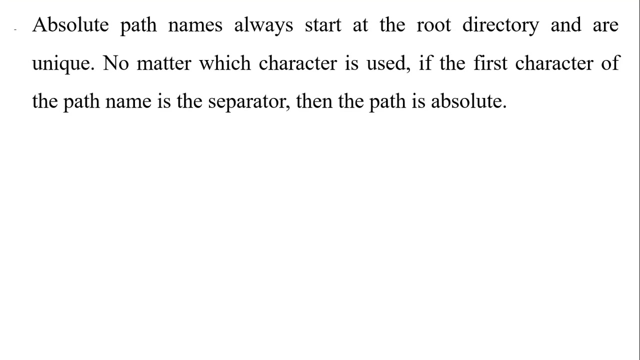 kindly search for and listen to the part one series and the part two series of these presentations on file management as posted in MLSwap YouTube channel, That is, MLSwap ICT YouTube channel. Absolute path names always start at the root directory and are unique No matter which character is used. 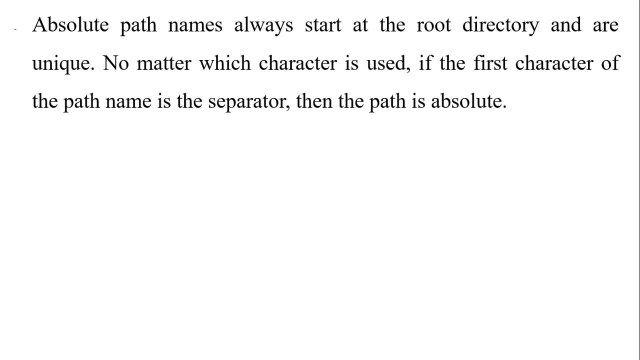 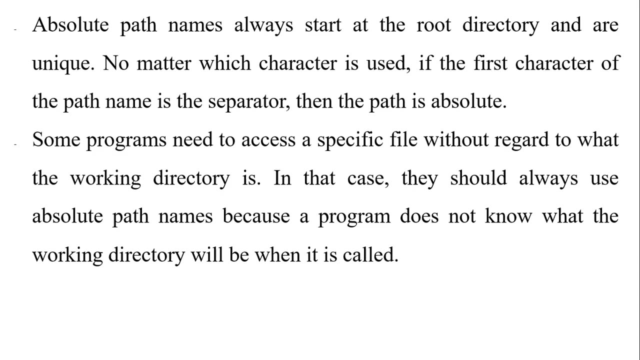 if the first character of the path name is the separator, then the path is absolute. Some programs need to access a specific file without regard to what the working directory is. In that case, they should always use absolute path names, because a program does not know. 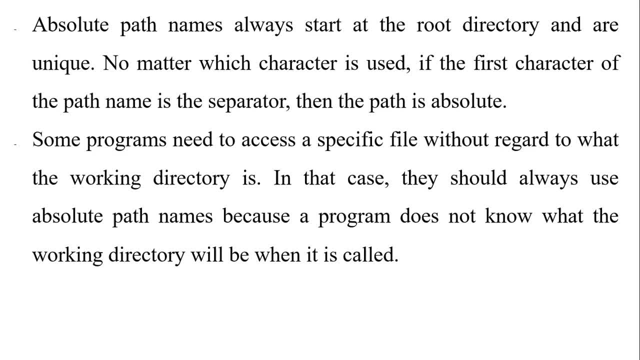 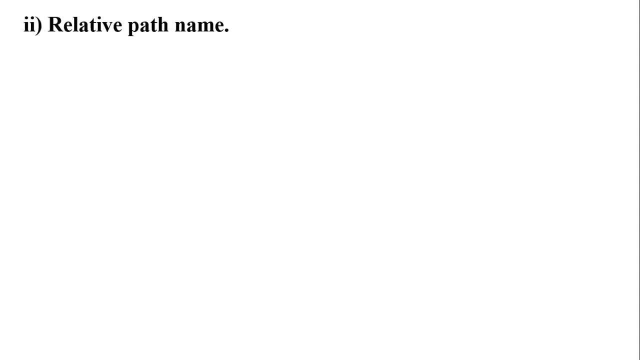 what the working directory will be when it is called. The absolute path name will always work, no matter what the working directory is. The second type of file naming is what we call the relative path name. This is used in conjunction with the concept of the working directory. 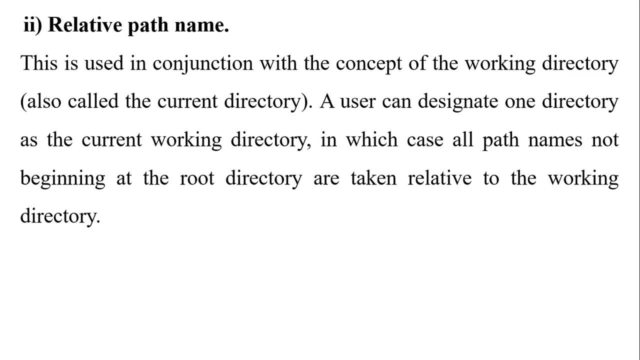 which is also called the current directory. A user can designate one directory as the current working directory, in which case all path names not beginning at the root directory are taken relative to the working directory. For example, if the current working directory is E2. 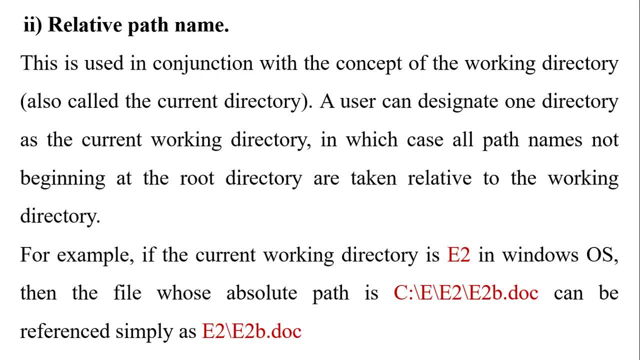 in Windows operating systems, then the file name whose absolute path we have seen as C colon backslash E backslash E2 backslash E2B dot doc can be referenced simply as E2 backslash E2B dot doc, where E2 is the current working directory. 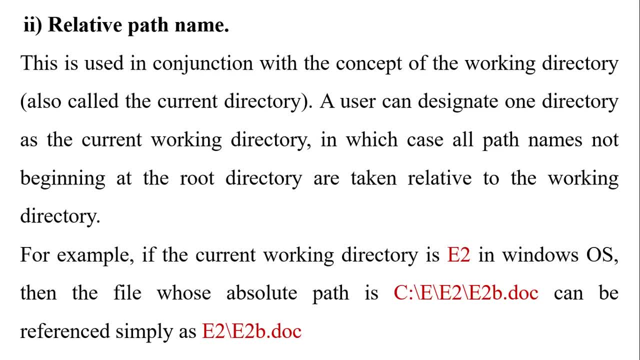 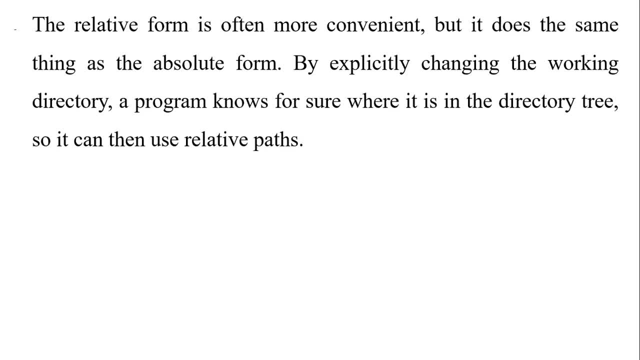 and E2B is the documented file that we are referring to. The relative form is often more convenient, but it does the same thing as the absolute form. By explicitly changing the relative form, by explicitly changing the working directory, a program knows for sure where it is in the directory tree. 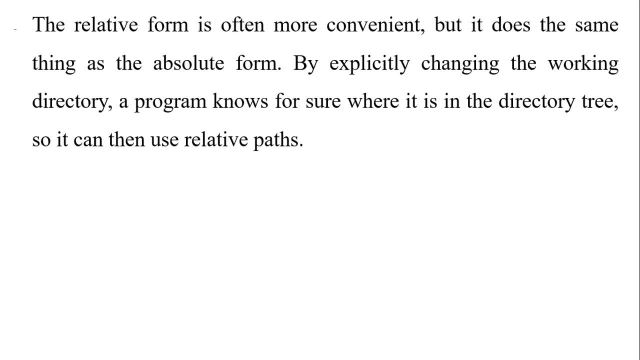 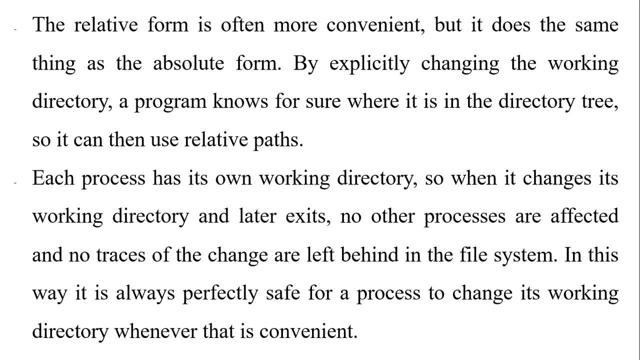 so that it can then use relative paths. Each process has its own working directory, so when it changes its working directory and later exits or exists, no other processes are affected and no traces of the change are left behind in the file system In this way. 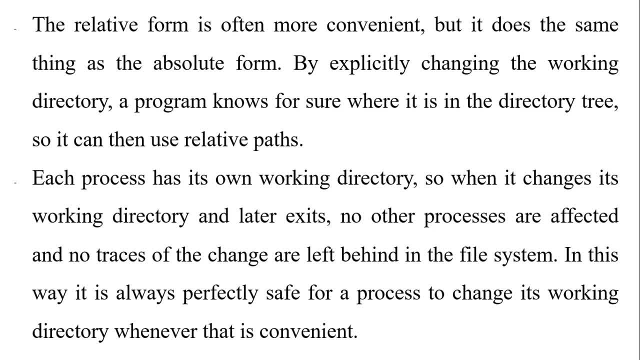 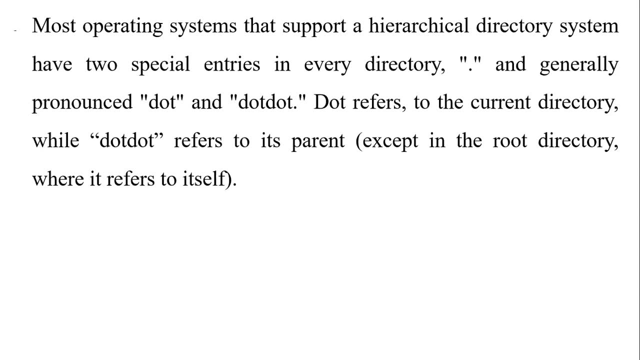 it is always perfectly safe for a process to change its working directory whenever that is convenient. Most operating systems that support a hierarchical directory system have two special entries in every directory, That is, dot, which is generally pronounced as dot, and dot dot. Dot refers to the current directory. 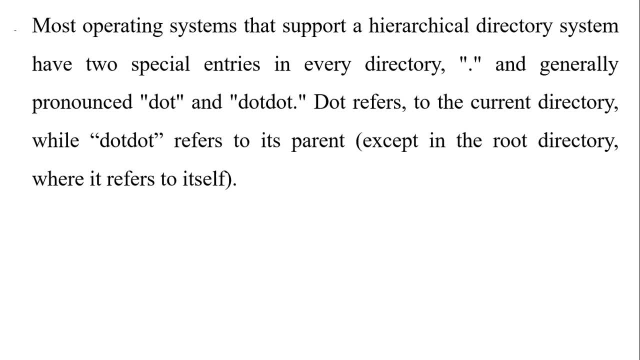 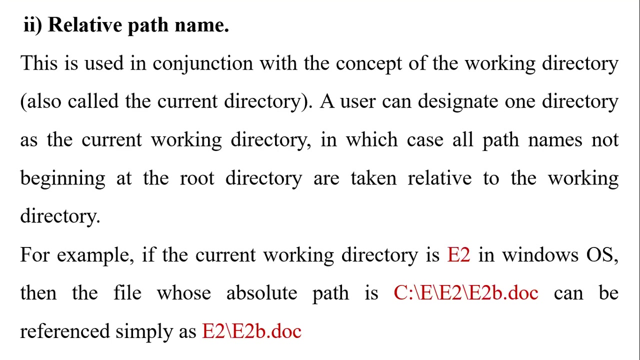 while dot dot refers to its parent, except in the root directory where it refers to itself. What I mean, my dear students and the rest of the learners, is that if, for example, I have a file like c, colon, backslash e, backslash e2, 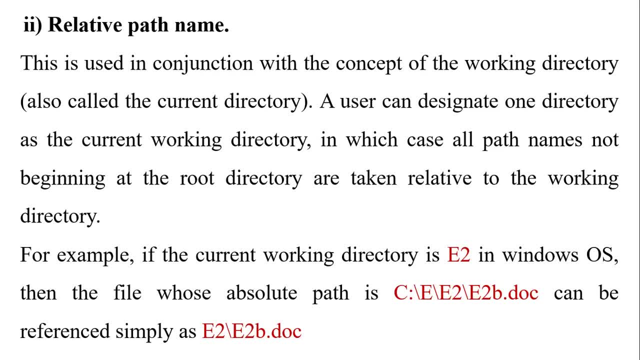 backslash: e2b dot doc. if I write it as e2 dot- e2b dot doc, it simply means that e2b is inside the subdirectory e2.. If I write it as e2 dot doc, it simply means that. 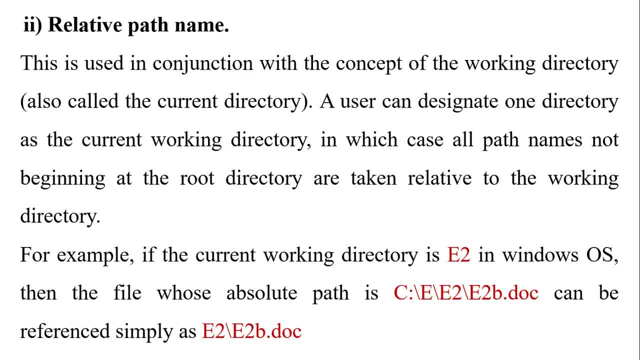 I am going towards the root, e2 dot will skip e2, dot dot. the second dot will skip the e, And then we shall of course be referring to c colon. So if I was to type c colon backslash e, backslash e2,. 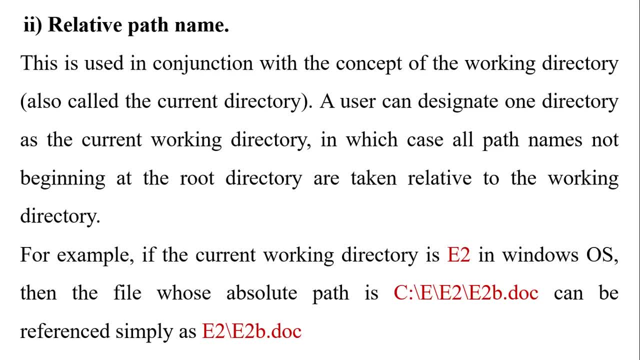 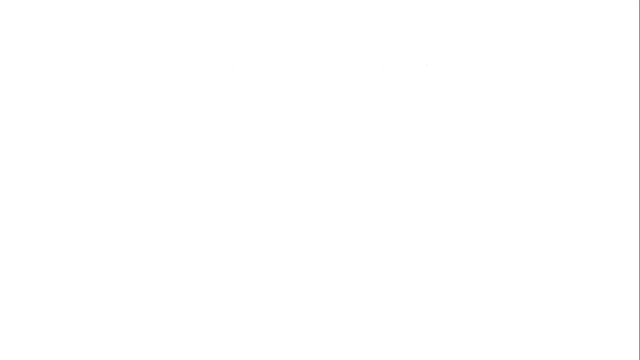 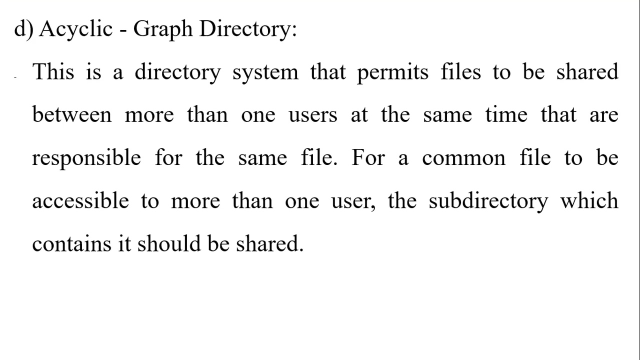 and then I type e2, dot, dot. I'll simply be referring to my root directory. The fourth type of directory system is what we call a cyclic graph directory. This is a directory system that pertains or permits files to be shared between more than one users. 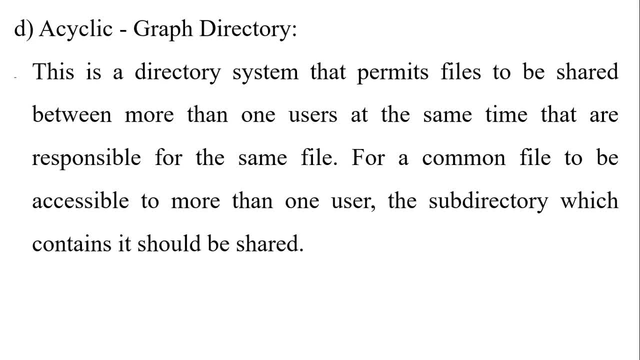 at the same time that are responsible for the same file. For a common file to be accessible to more than one user, the subdirectory which contains it should be shared. A shared directory or file will exist in the file system in two or more places at once. 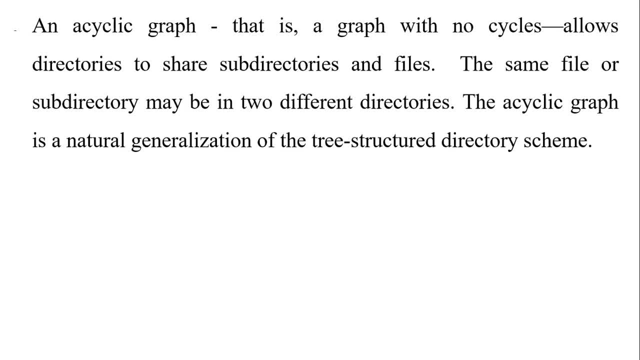 A cyclic or a cyclic graph- that is, a graph with no cycles- allows directories to share subdirectories and files. The same file or subdirectory may be in two different directories. The acyclic graph is a natural generalization of the tree structure directory. 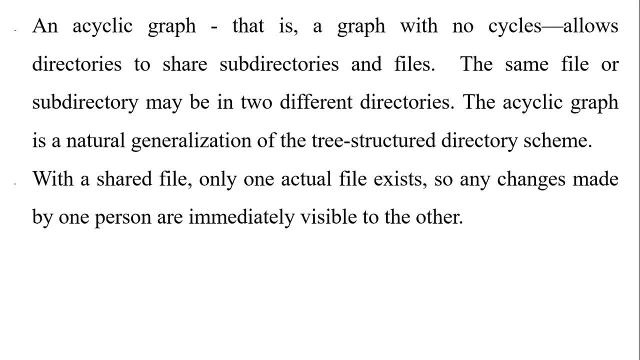 or sub directory scheme. With a shared file, only one actual file exists, so any changes made by one person are immediately visible to the other. Sharing is particularly important for subdirectories. A new file created by one person will automatically appear in all the shared subdirectories. 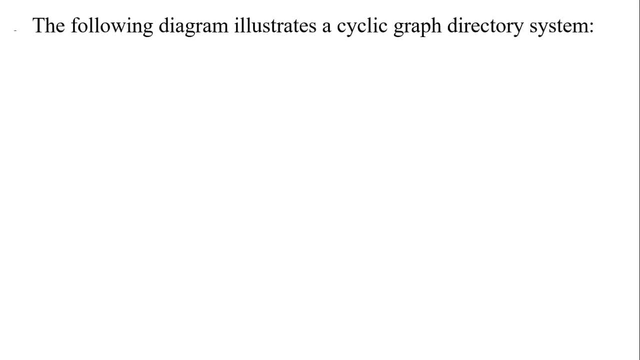 The following diagram illustrates a cyclic graph directory system. So in this diagram, my dear students and the rest of the learners, we can see that we have the root directory, which is C colon, or which, in this case, is the hard disk storage medium. 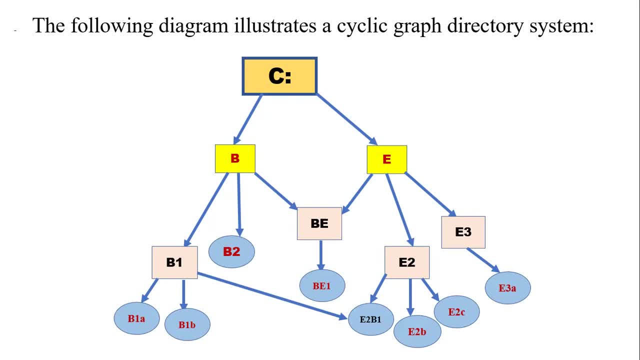 And this storage media. we have two user file directories, which are B and E, And then we have a subdirectory called B- E, which has been shared and is accessible through the user file directory B and the user file directory E. This simply means. 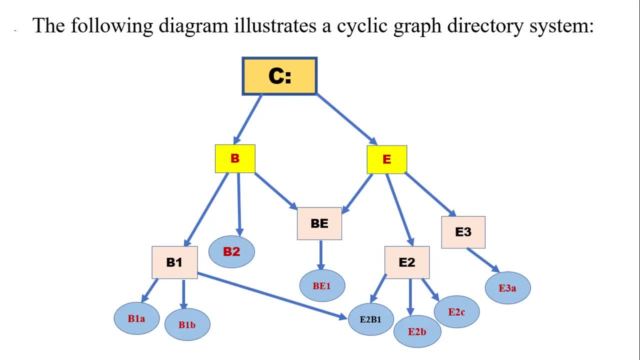 that when the user B is inside his or her user file directory B, he or she will be able to see two directories, that is, B1 as well as B? E, While on the side of the user E, he or she will be able to see 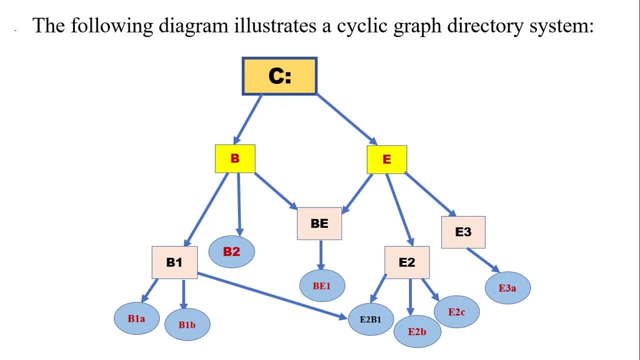 three directories or three user file directories, which will be B E, E2, and E3. And therefore, in this case, the subdirectory B? E has been shared between the user B and the user E And therefore B? E will appear as a user file subdirectory. 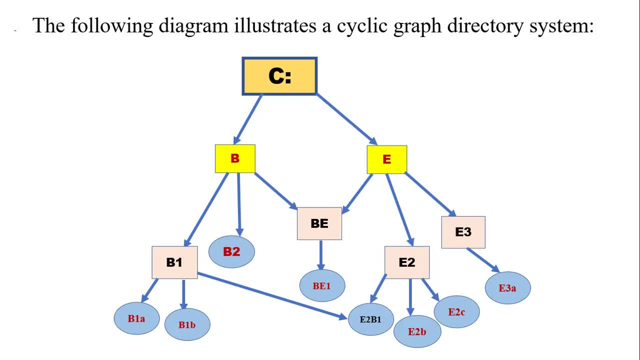 for user E and for user B. We also have, therefore, another file. We also have another file that has been shared amongst two users. This file is file B is file E2 B1.. E2 B1 has been shared between. 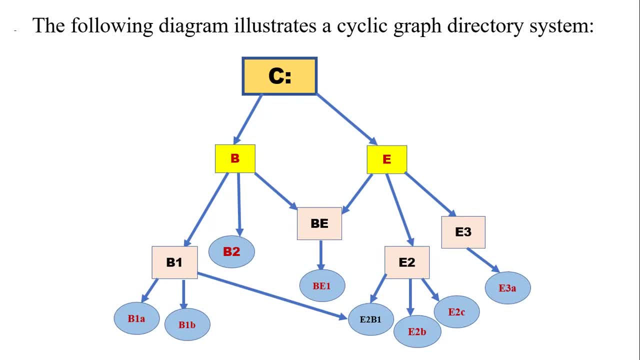 the user for user file subdirectory B1 and the user file subdirectory E2.. Therefore, the user file subdirectory E2 or a user who accesses the subdirectory or the user file subdirectory E2 will be able to see file E2- B1. 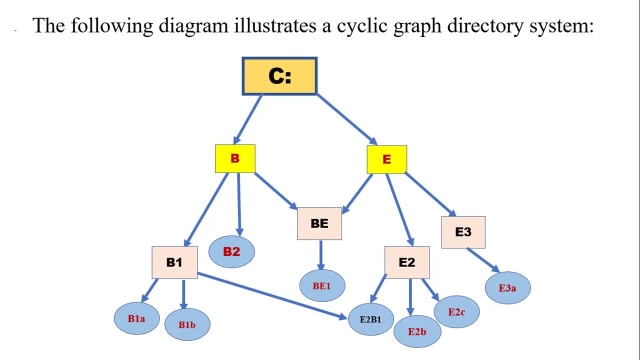 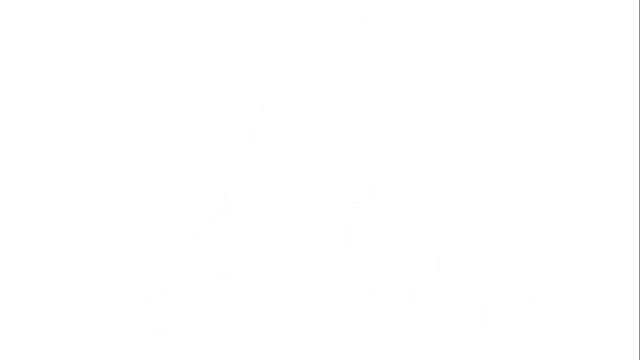 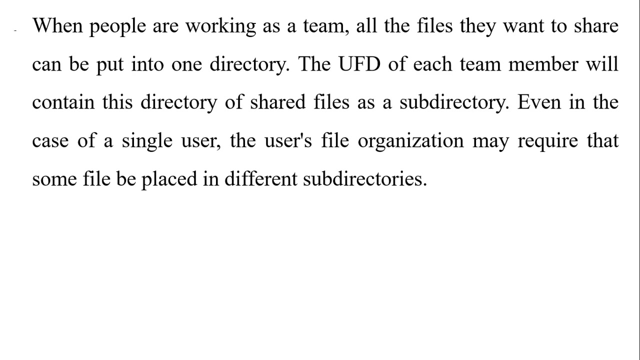 in his or her folder or her directory, while B1 will also be able to see the shared file E2 B1 in his or her directory, which is directory B1.. When the people are working as a team or other files they want to share. 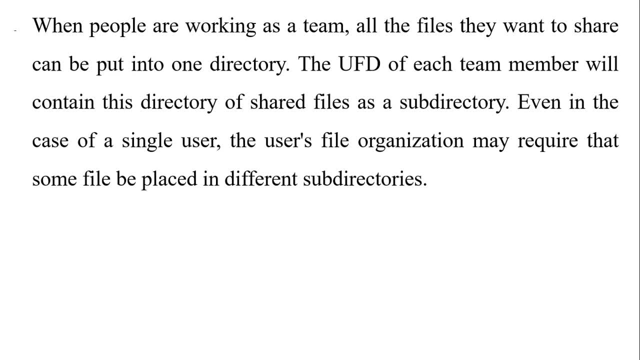 can be put into one directory. The user file directory, or UFD, of each team member will contain this directory of shared files as a subdirectory. Even in the case of a single user, the user's files organization may require that some files be placed. 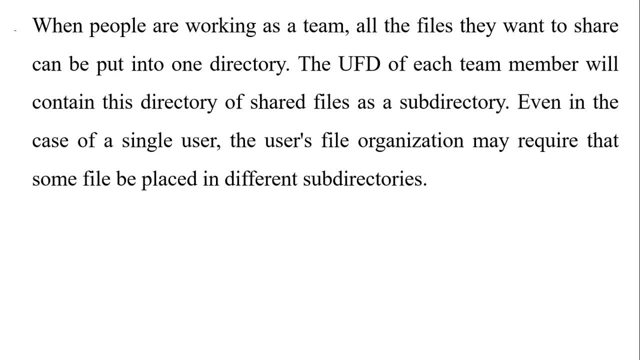 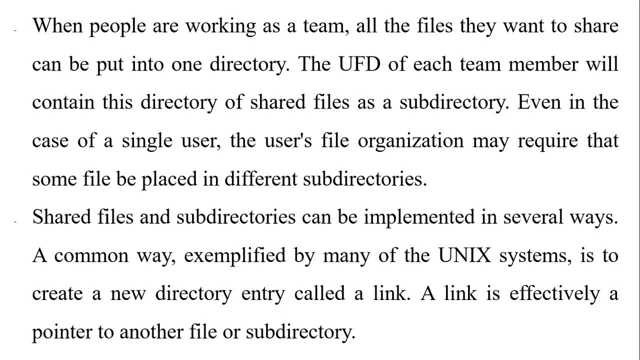 in different subdirectories. Shared files and subdirectories can be implemented in several ways. For example, if you want to share a file with another user, you can use the shared file E2- B1 in your directory- A common way exemplified by many 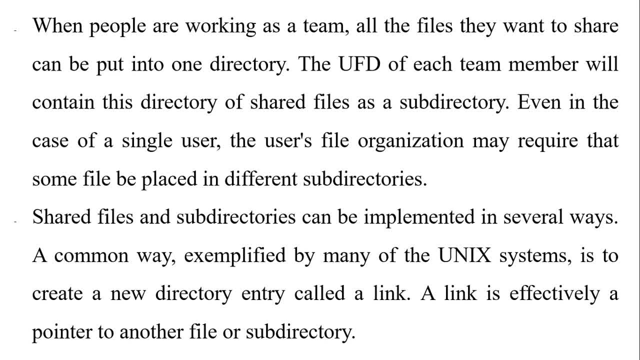 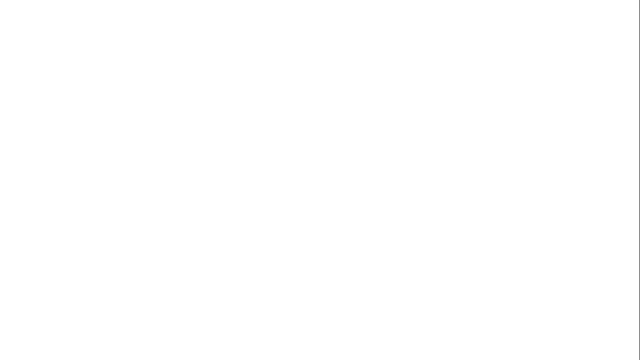 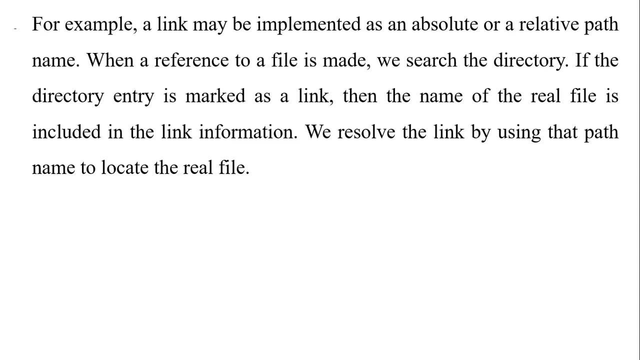 of the UNIX systems is to create a new directory entry. that is called a link. A link is effectively a pointer to another file or subdirectory. For example, a link may be implemented in a relative path When a referenced a file is meant. 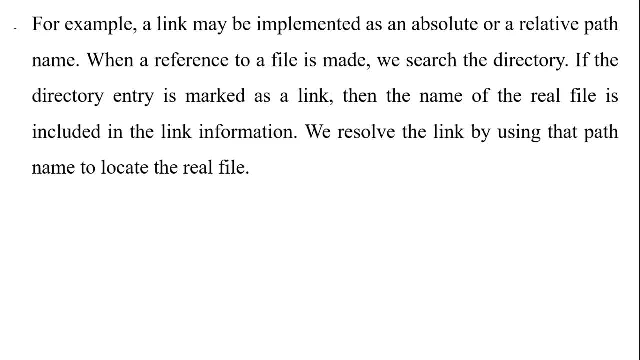 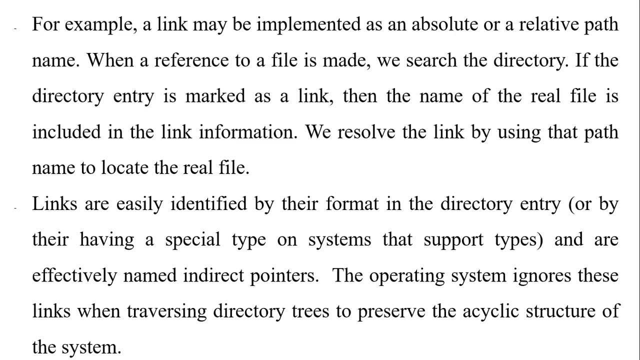 we search the directory. If the directory entry is marked as a link, then the name of the real file is included in the link information. We resolve the link by using that method. The links are easily identified by their format in the directory entry or by 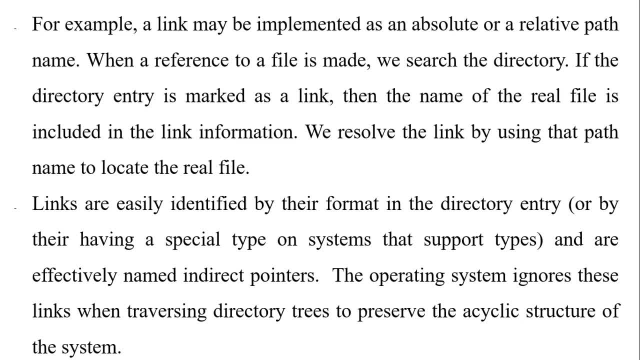 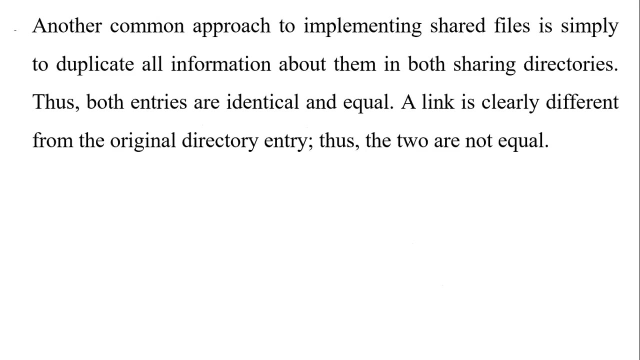 their having a special type on systems that support types and are effectively named in direct pointers, The operating system ignores these links. Another common approach to implementing shared files is simply to duplicate all information about them in both sharing directories. Thus most entries are identical. 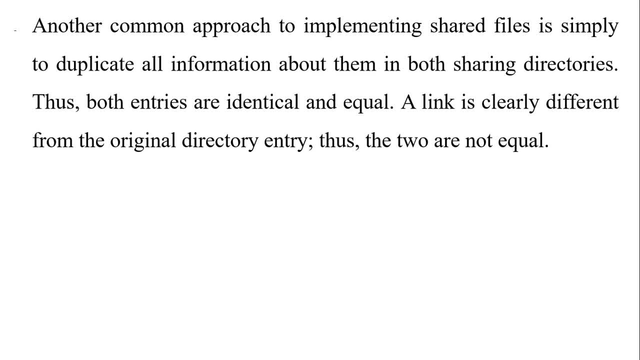 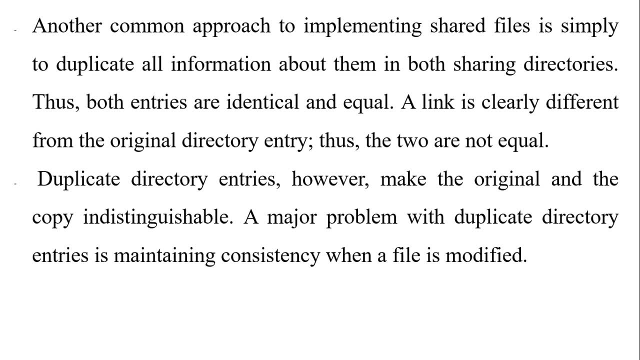 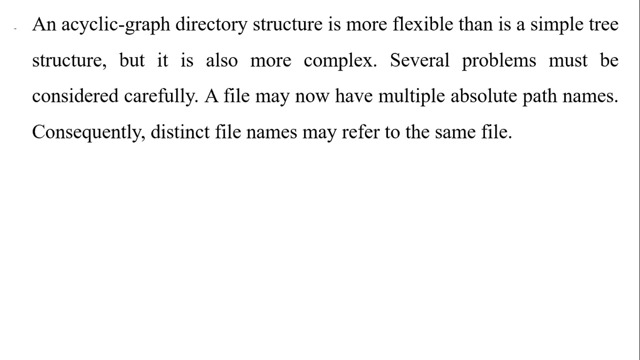 and equal. A duplicate directory entries, however, make the original and the copy indistinguishable. A major problem with duplicate directory entries is maintaining consistency when a file is modified. An acyclic graph directory structure is more complex. Several problems must be considered carefully. 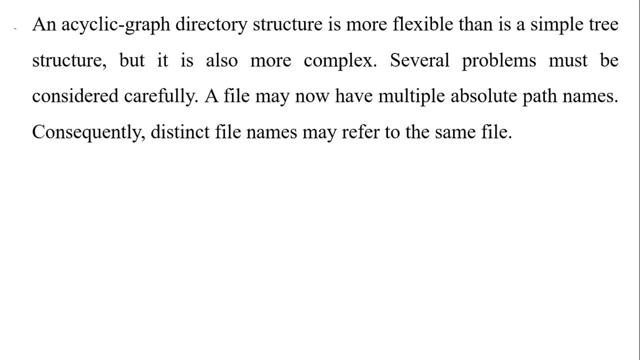 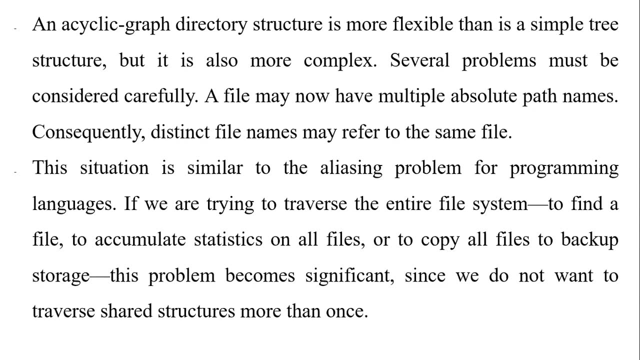 A file may now have multiple absolute party names. Consequently, distinct file names may refer to the same file. This situation is similar to the case with the most common programming languages. If we are trying to traverse the entire file system to find a file, 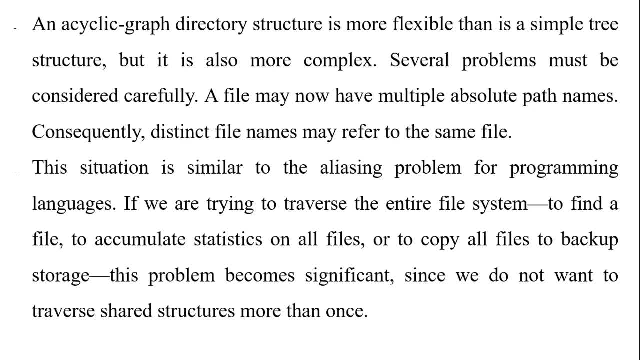 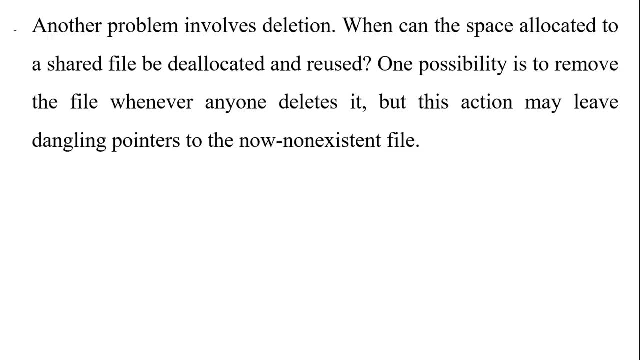 to accumulate statistics on all files or to copy all files to backup storage. this problem becomes significant since we do not want to traverse the entire file. Another problem involves deletion. When can the space allocated to a shared file be deallocated and reused? One 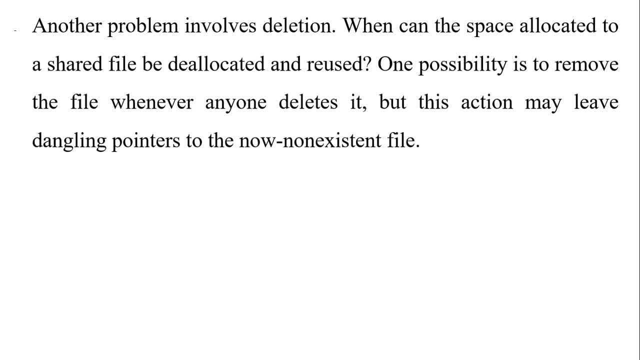 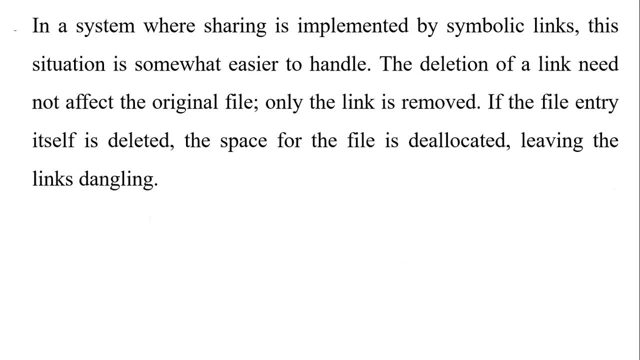 possibility is to remove the file whenever anyone deletes it, but this action is not necessary If the remaining file pointers contain actual disk addresses and the space is subsequently reused for other files. these dangling pointers may point into the middle of other files In a 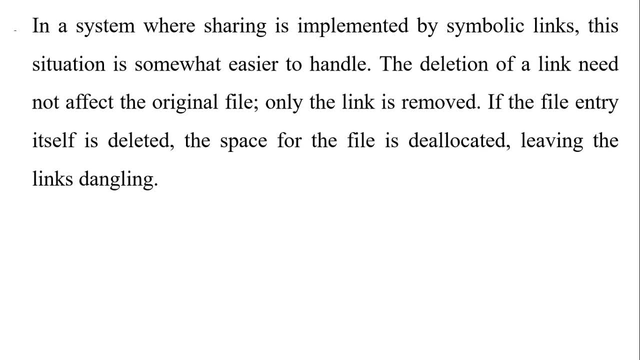 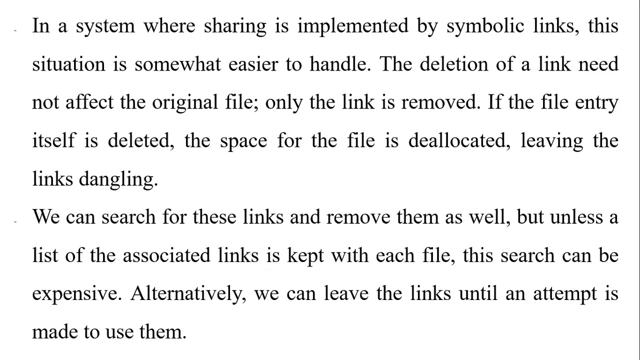 system where sharing is a must. the deletion of a link need not affect the original file, only the link is removed If the file entry itself is deleted, the space for the file is limited. this search can be expensive. Alternatively, we can: 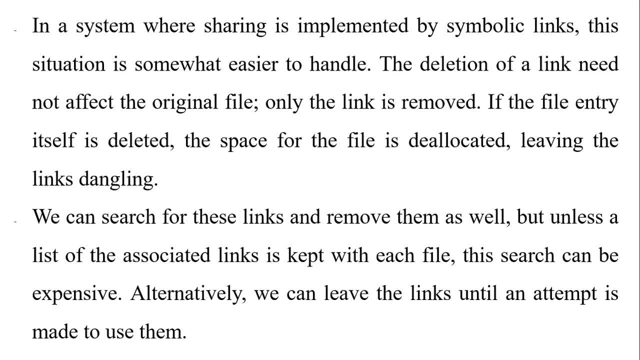 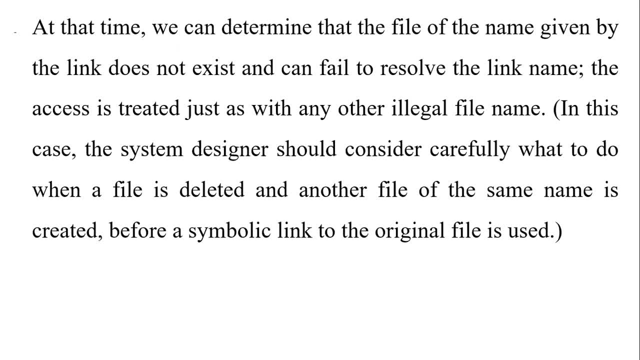 leave the links until an attempt is made to use them. At that time, we can determine that the access is treated just as with any other illegal file name. In this case, the system designer should consider carefully what to do when a file is deleted. 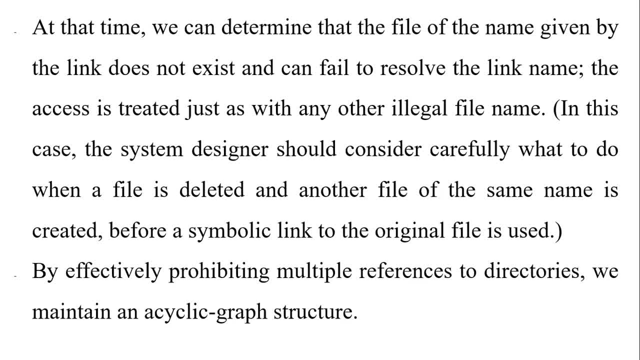 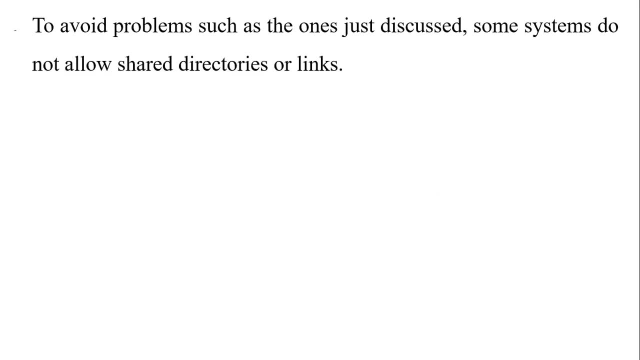 and another file of the file is deleted. To avoid the problems such as the ones just discussed, some systems do not allow shared directories or links. For example, in Microsoft Disk Operating System, a directory structure is a tree structure rather than an acyclic. 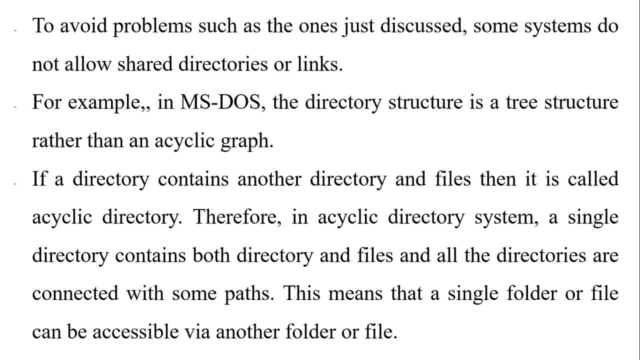 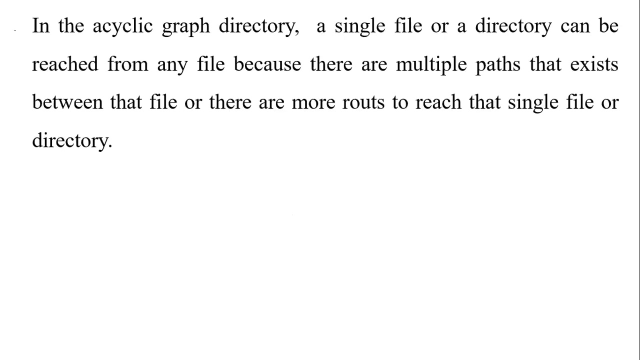 graph. If a directory contains another directory and files, then it is called an acyclic directory. Therefore, in an acyclic directory a single folder or a file can be accessible via another folder or a file In the acyclic graph directory. 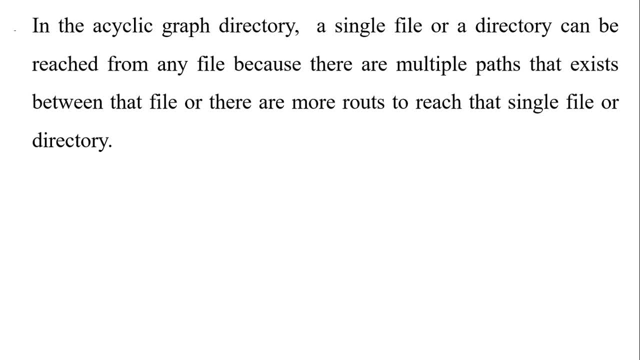 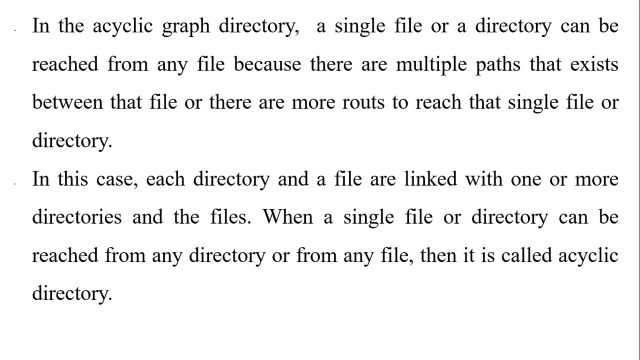 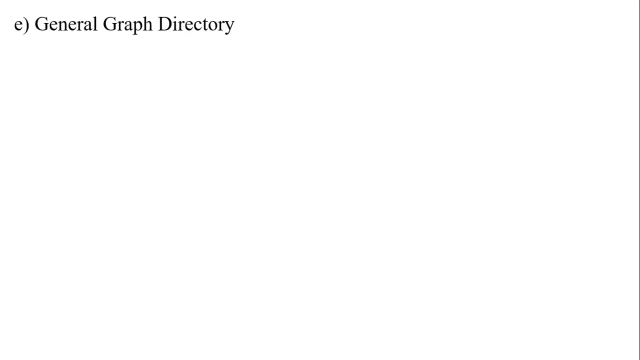 a single file or a directory can be reached from any directory or from any file. In this case, each directory and a file are linked with one or more directories in the files. When a single file is linked with another file, the file is linked. 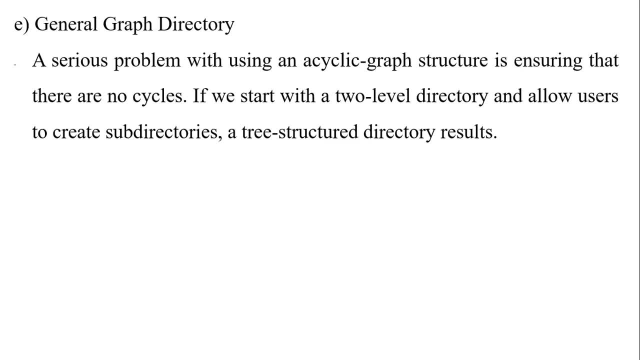 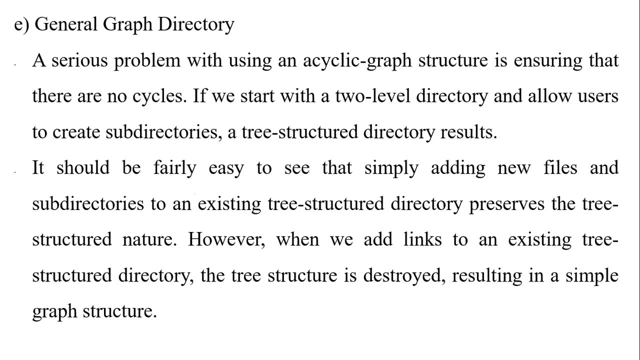 with another file. Let us now look at the general graph directory. A serious problem with using an acyclic graph is that simply adding new files and subdirectories to an existing tree structure directory preserves the tree structure in nature. However, when we add links, 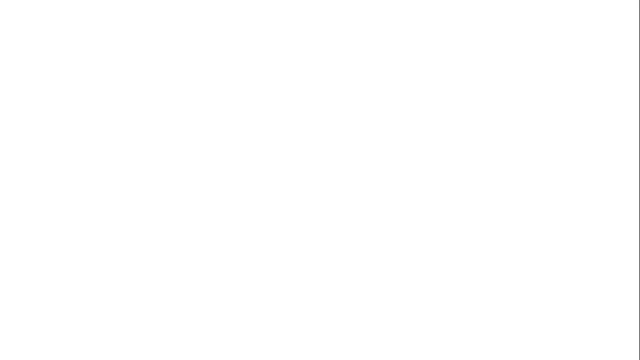 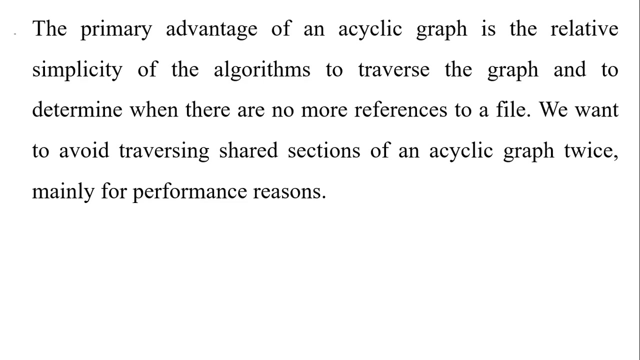 to an existing tree structure directory. the resultant is that the relative simplicity of the algorithms to traverse the graph and to determine when there are no more references to a file. We wanted to avoid traversing shared sections of an acyclic graph twice, mainly because we 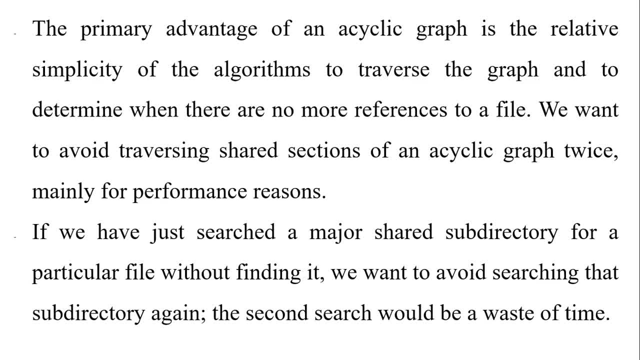 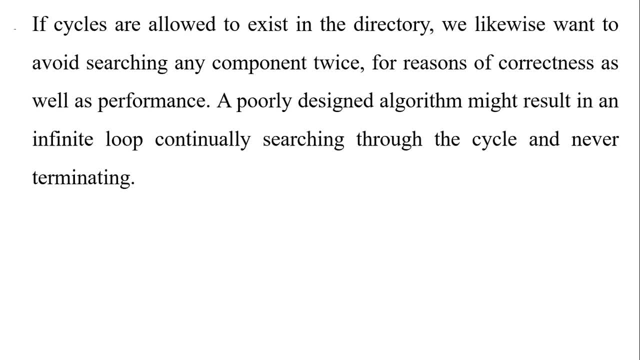 wanted to avoid searching that directory again. The second search would be a waste of time If cycles are allowed to exist in the directory. we likewise wanted to avoid searching any component twice or three times in an infinite loop, continually searching through the cycle and never. 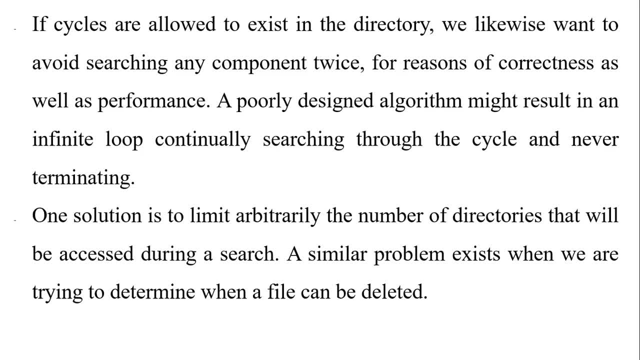 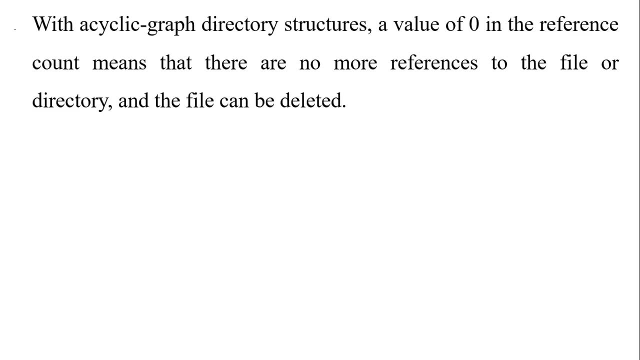 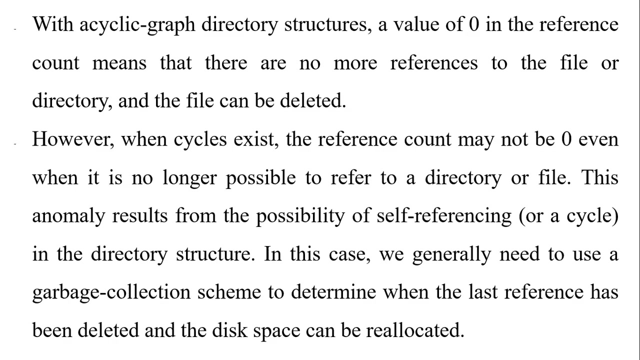 terminating. One solution is to limit arbitrarily the number of directories that will be accessed during the cycle. With acyclic graph directory structures, a value of zero in the reference count means that there are no more references to the file or directory, and the file can be. 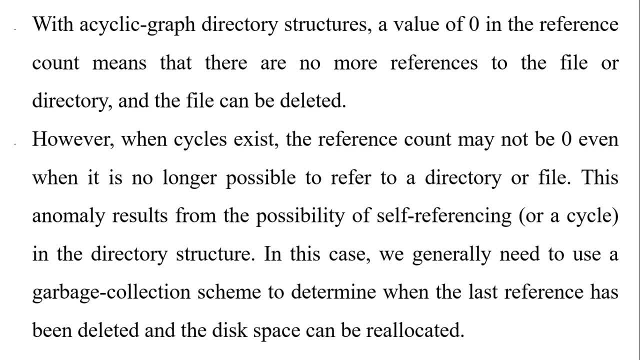 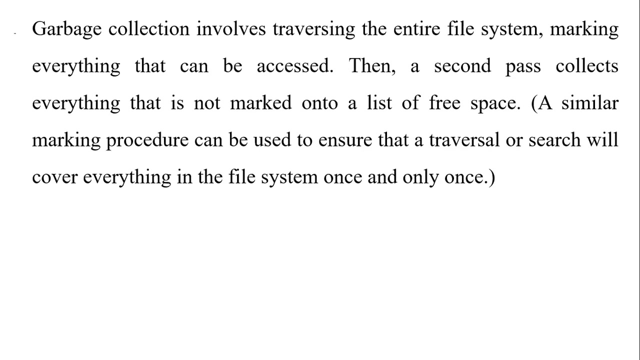 deleted. However, when cycles exist, the file can refer to a directory or file. This anomaly results from the possibility of self-referencing or a cycle in the directory structure. In this case, we generally need to use a single reference to the. 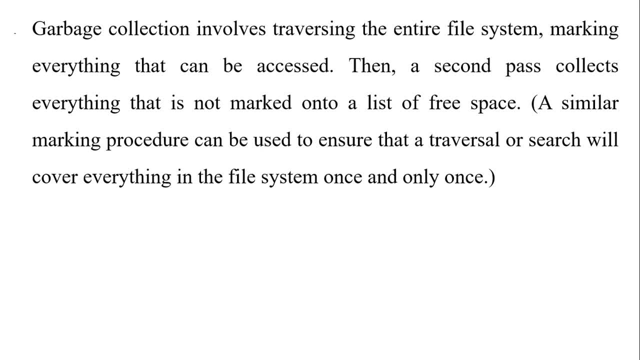 file in the file system. The second pass collects everything that is not marked into a list of free space. A similar marking procedure can be applied to a system once and only once. Garbage collection for a disk-based file system, however, is extremely. 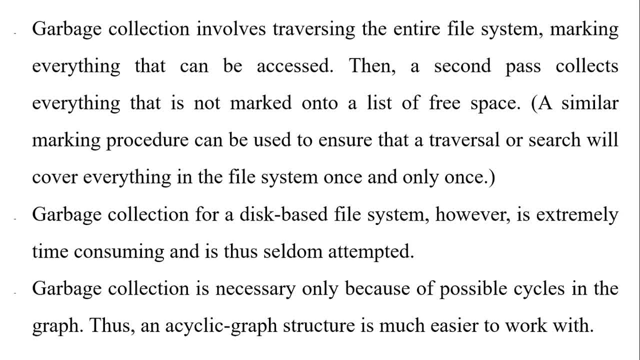 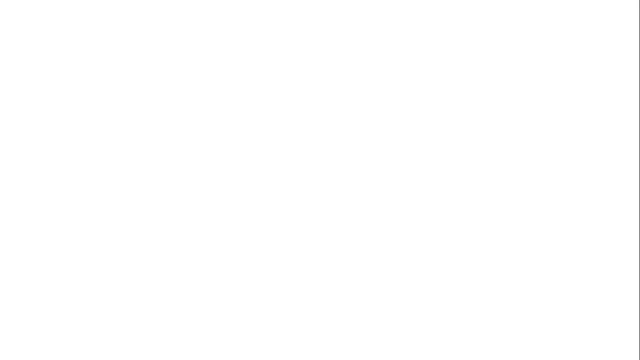 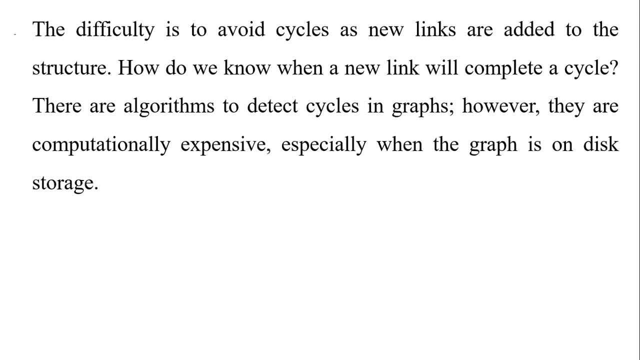 time-consuming and is thus serodrome. attempted Garbage collection is necessary only because it is much easier to work with. The difficulty is to avoid cycles as new links are added to the structure. How do we know when a new link will complete a? 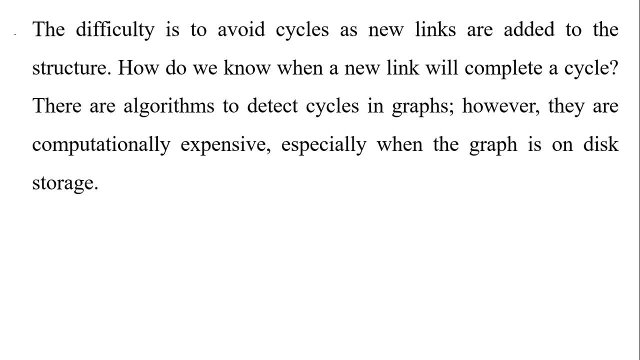 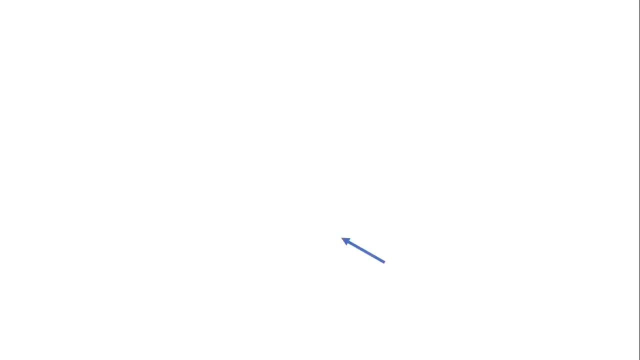 cycle. There are several ways to do this, especially when the graph is on a disk storage. A simple algorithm is the special case of directories and links is to bypass links during directory traversal. The following diagram illustrates a general graph directory: Just as it. 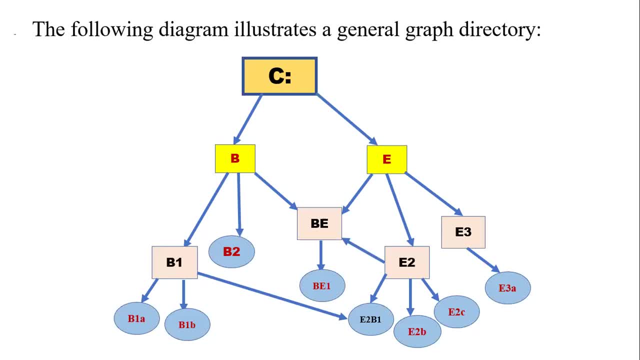 was the case in the other directory systems that have already explained. this graph directory, or this graph system, indicates that the user file directory E is able to access three other user subdirectories. These are B2, E2, and E3.. However, 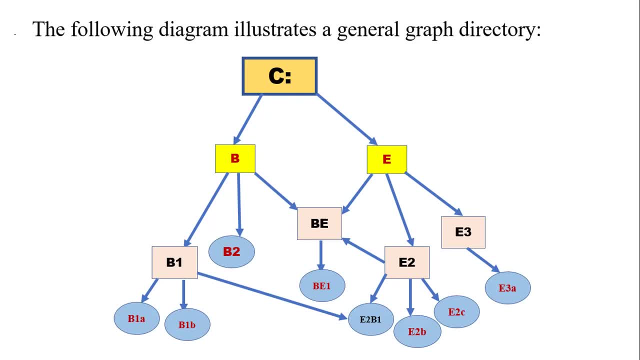 once we are in the user subdirectory E2, we can access BE. Therefore, in this case, whereas BE is a subdirectory for user B and is accessible as a subdirectory for user B at the same time for user E, 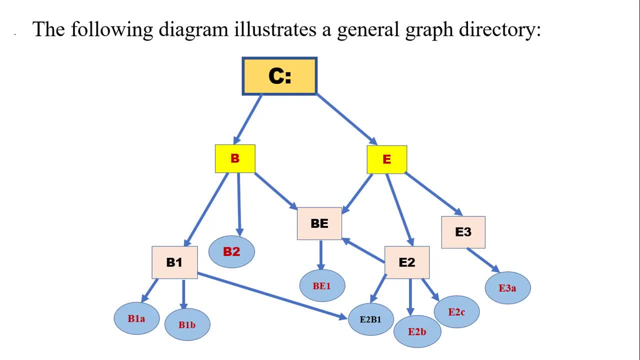 it is able to indicate BE as if it is its subdirectory And therefore BE is accessible through E, while at the same time, E2, which is a subdirectory, is able to access BE as its subdirectory And therefore that 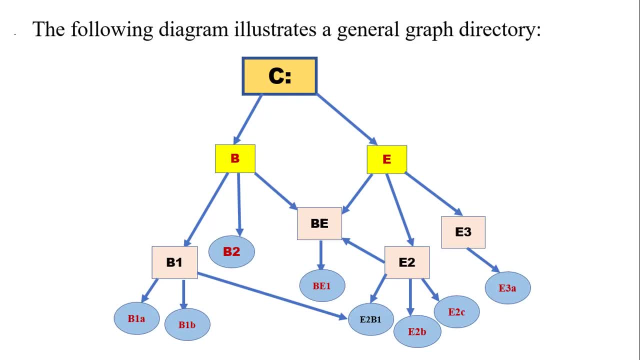 forms what we are calling a general graph directory, and that is what differentiates it from the other type that we have just looked at here. So it means that the file BE1, that is accessed through the user subdirectory BE, can also be accessed. 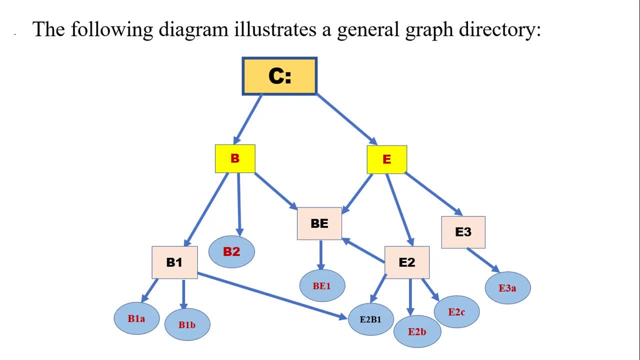 from user file subdirectory E2 through BE. And therefore that means that from the user subdirectory E2, we can be able to access BE1.. And therefore that also means that the file BE1 is accessible from user directory B through. 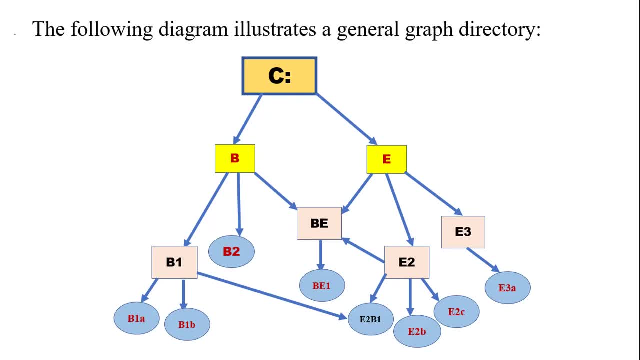 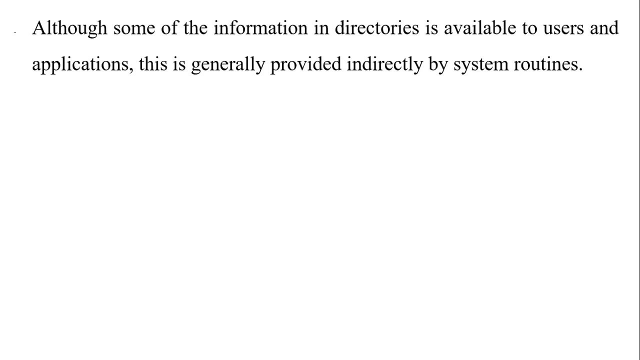 user subdirectory E through BE And, at the same time, it is accessible through user subdirectory E2 through BE And, of course, E2 is able to access or through E2, E2, and B1.. Although some of the 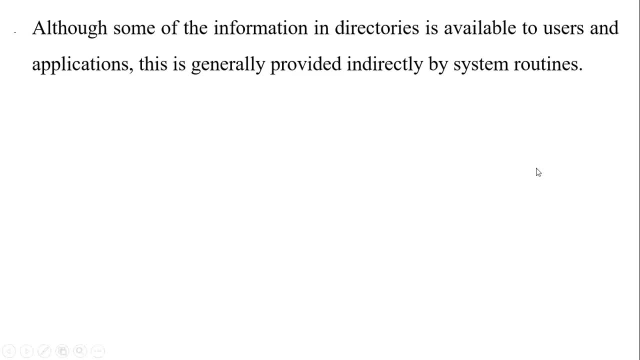 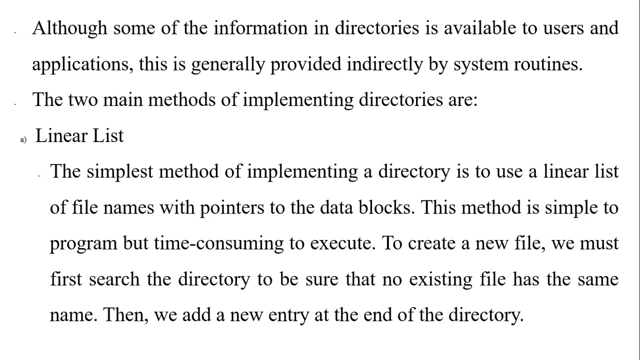 information in directories is available to users and applications. this is generally provided indirectly by system routines. The two main methods of using linear lists is the simplest method of implementing a directory such that we are able to use a linear list of filenames with pointers to the 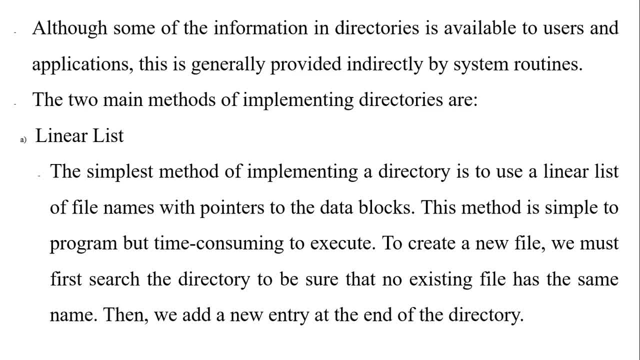 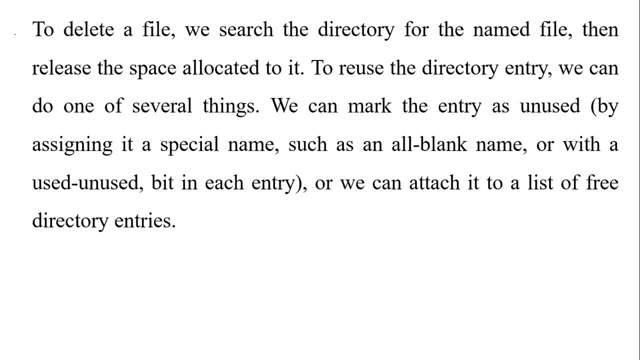 data blocks To be sure that no existing files have the same name. then we add a new entry at the end of the directory To delete a file. we search the directory for the named file. We can mark the entry as unused by assigning: 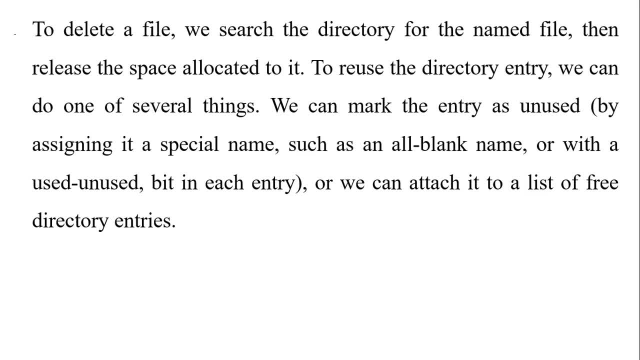 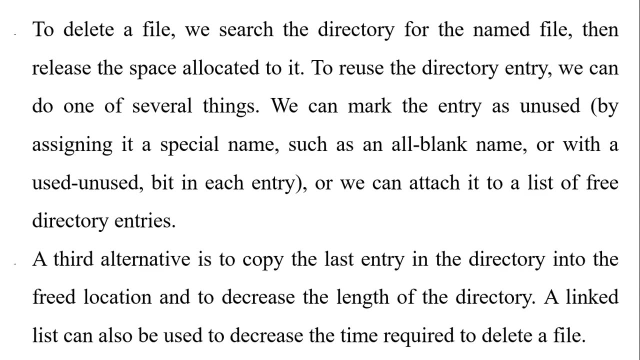 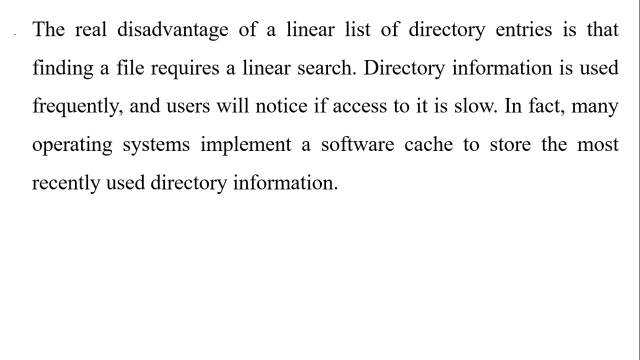 it a special name, such as an all-blank name or with an unused bit in each entry, Or we can attach it to the directory to decrease the length of the directory. A linked list can also be used to decrease the time required to delete a. 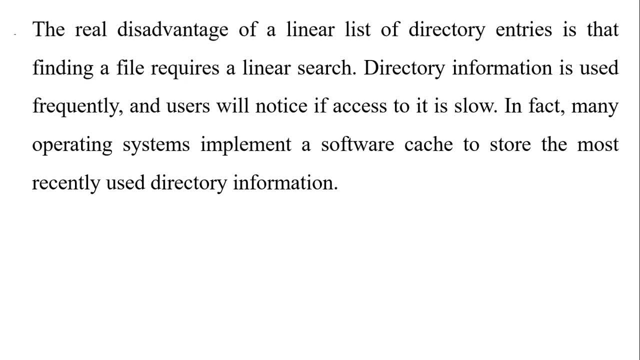 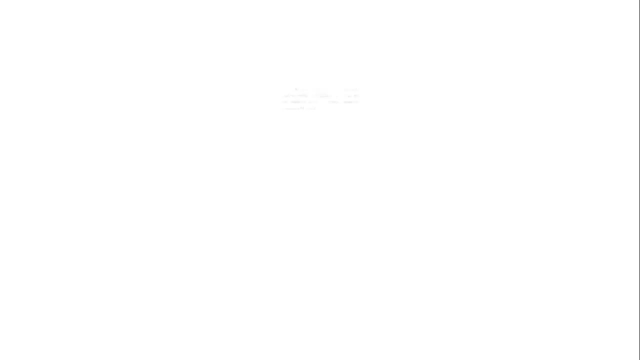 file. The real disadvantage is that it is slow. In fact, many operating systems implement a software cache to store the most recently used directory information. A cache hit avoids the need to constantly re-read the list at any time. However, the requirement that the 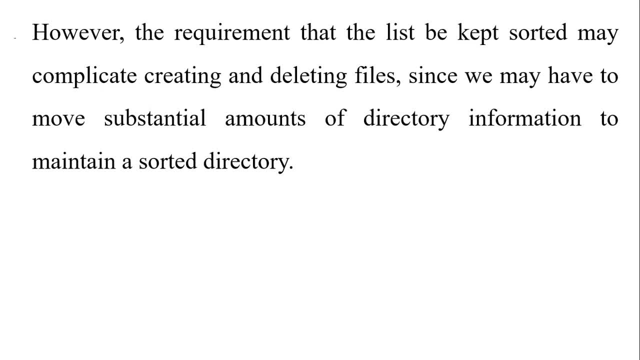 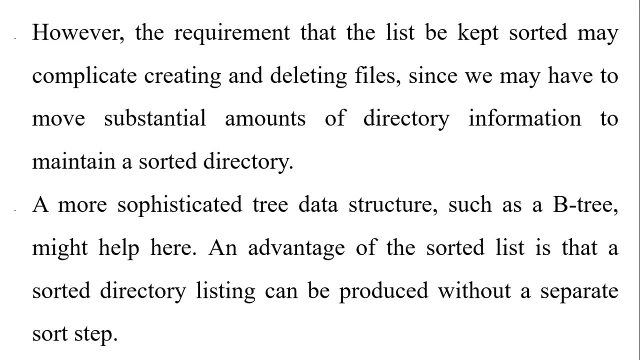 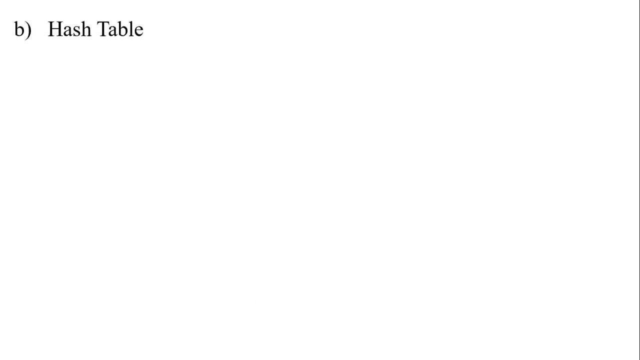 list must be kept. sorted may complicate creating and deleting files, since we may have to move substantial amounts of directory information to the list. The advantage of the sorted list is that a sorted directory listing can be produced without a separate sort step. The other type. 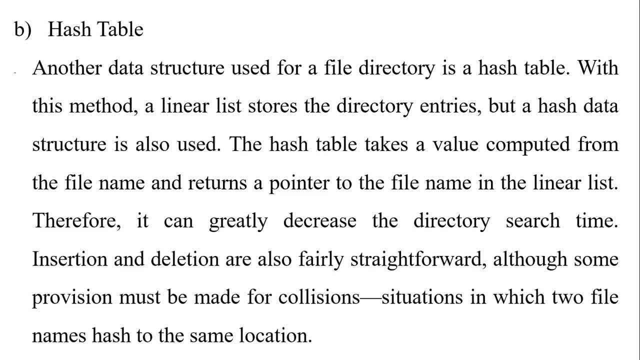 is what we call the hash table. Another data structure is the hash table. With this method, a linear list stores the directory entries, but a hash data structure is also used. The hash table takes a value computed from the hash table, The hash. 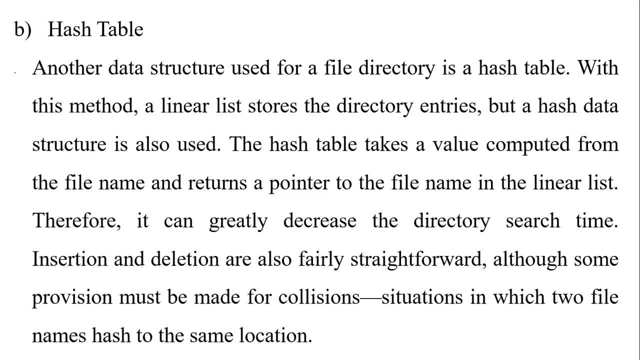 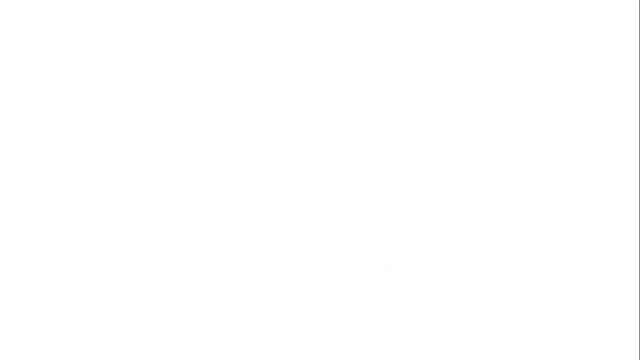 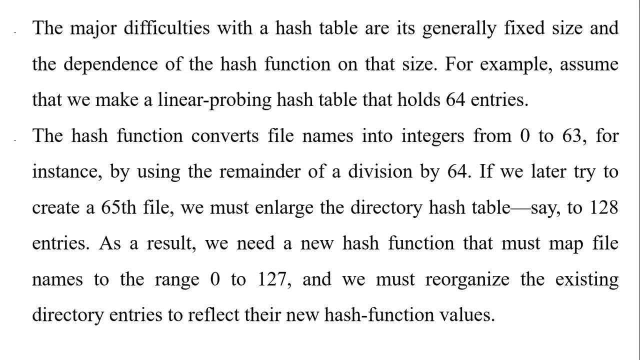 table has two file names hashed to the same location. The major difficulties with a hash table are its generally fixed size and the dependence of the hash table. The hash function converts file names into integers from 0 to 63, for instance by using: 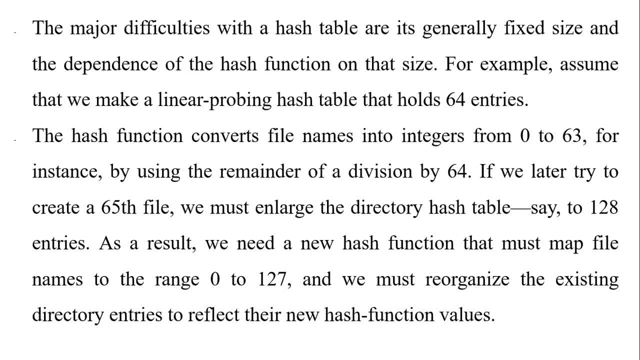 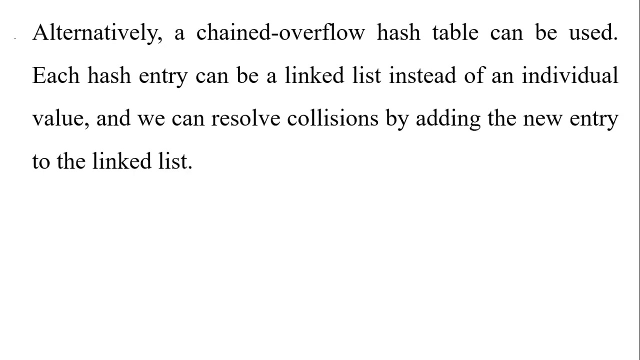 the remainder of n division by 64.. If we never try to create a new hash function, we need a new hash function that must map file names to the range of 0 to 127, and we must reorganize the existing directory entries. 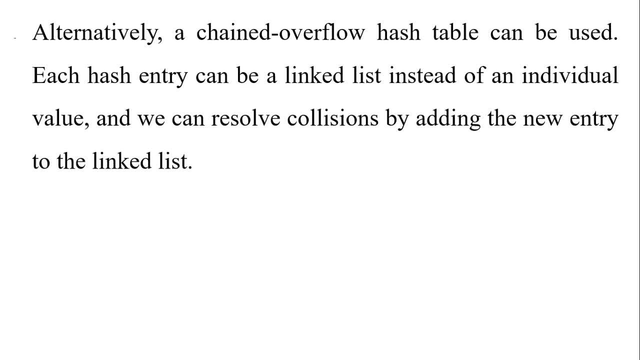 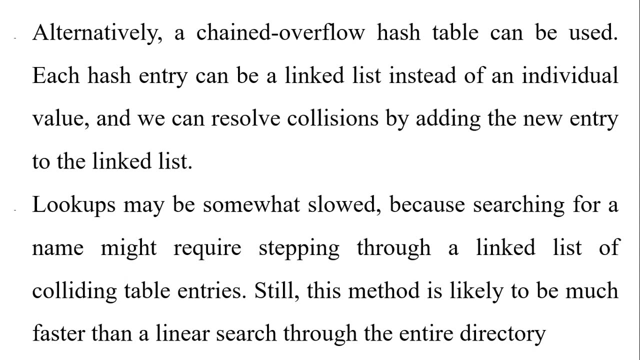 so that each hash entry can be a linked list instead of an individual value and we can resolve collisions by adding the new entry to the linked list. Lookups may be somewhat slowed because searching for a name is likely to be much faster than a linear. 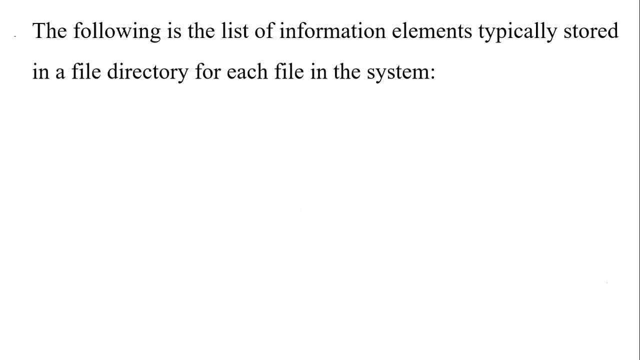 search through the entire directory. The following is the list of information elements that are typically stored in a file directory. for each file in the system, The name as chosen by the creator, that is, user or program. this name must be unique within a specific directory. 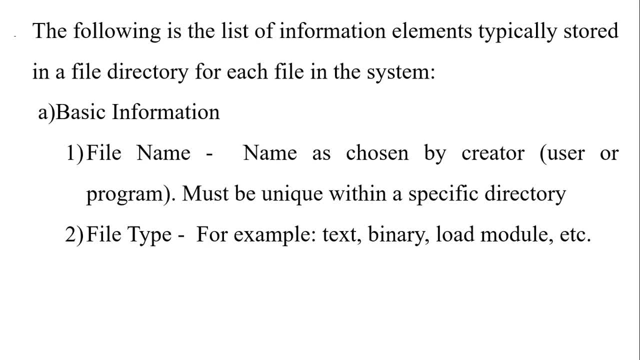 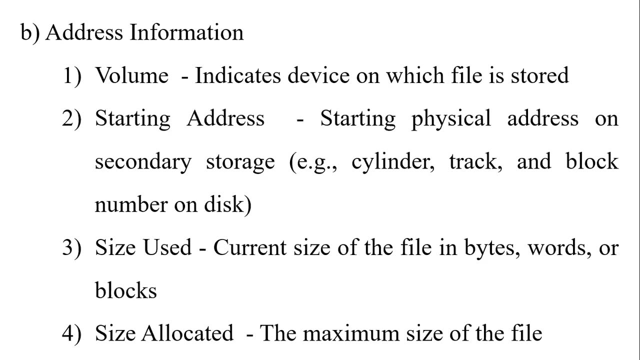 Number two is the file type, for example, text, binary, load module, etc. Number two, or the secondary category of information, is what we call the address information. This includes the volume, which indicates device on which the file is stored. Number two is: 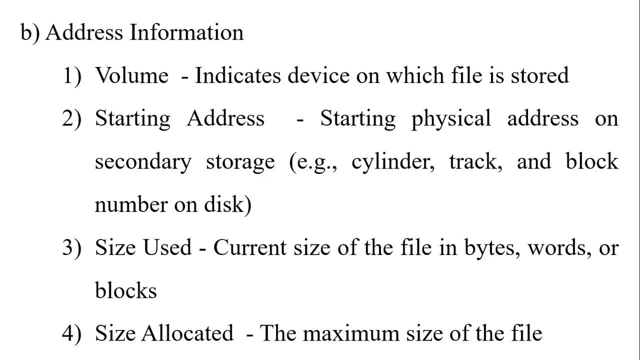 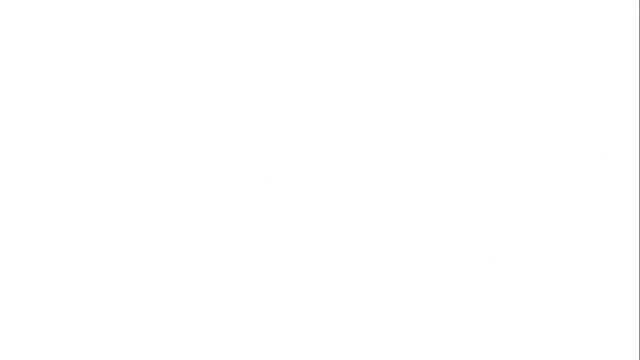 the cylinder, a track and block number on the disk. Number three is the size used. It indicates the current size of the file in bytes once on it. Number four is the access control information. This includes number one, the owner. This is: 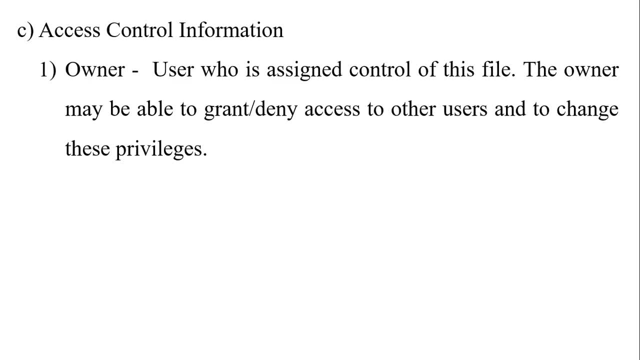 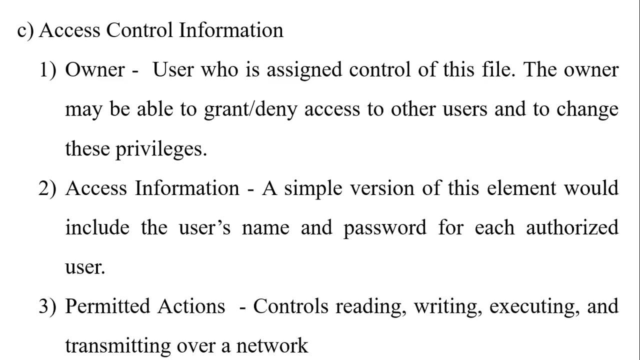 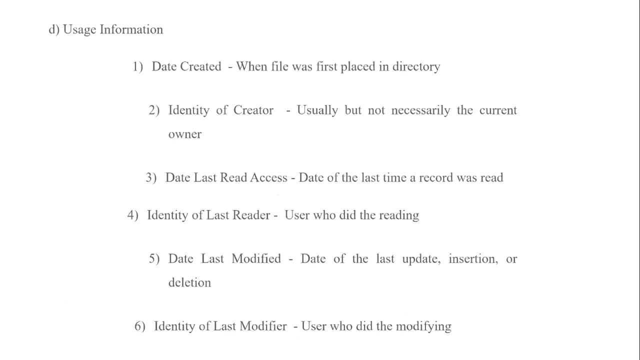 the user who is assigned control of this file. The owner may be able to access the user's name and password for each authorized user. Number three is the permitted actions. This controls the reading, the writing, executing and transmitting over a network. The. 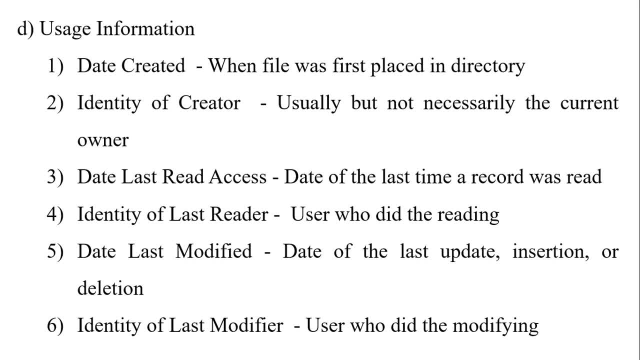 user has access to the user's data. The user has access to the user's data. This includes the date created, the identity of the creator, the date last read access, the date of the last time the red access was done, the date of. 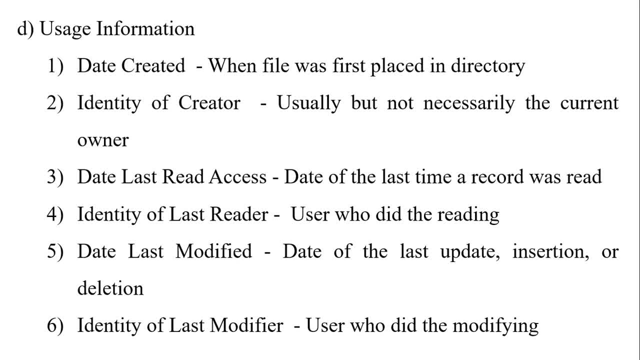 the last time the red access was done and the date of the last time the red access was run. The identity of the last reader indicates the user who did the reading. The date last modified indicates the date of the last update, insertion or deletion, while. 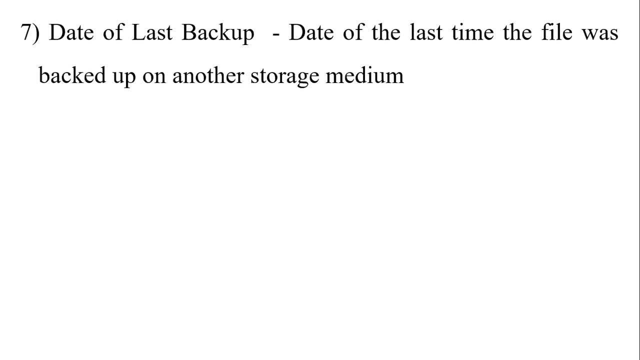 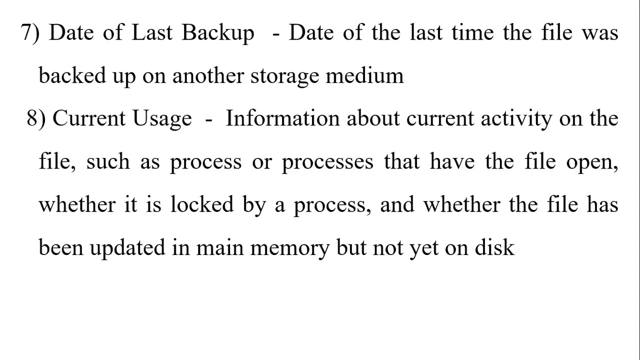 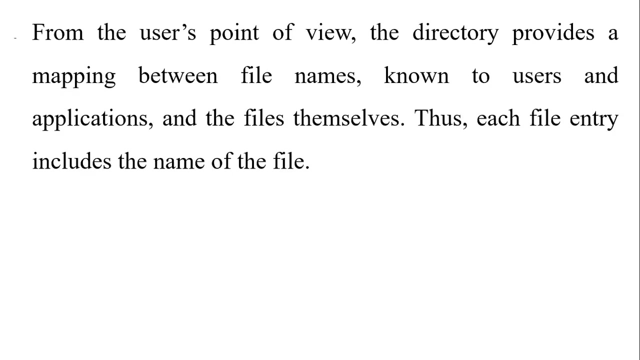 identity of last backup is the date of last backup. This is the date of the last time the file was backed up on another storage medium. Number eight is current usage. This is the date when the file was updated in the main directory, but not yet. 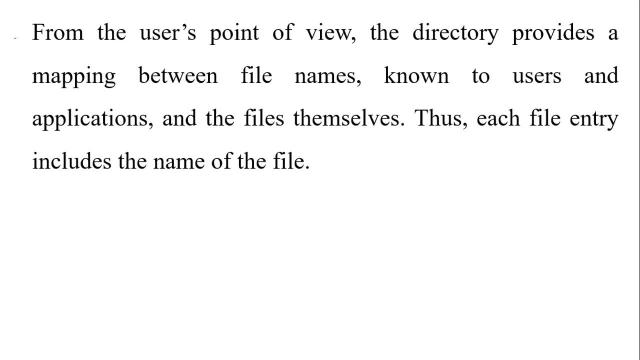 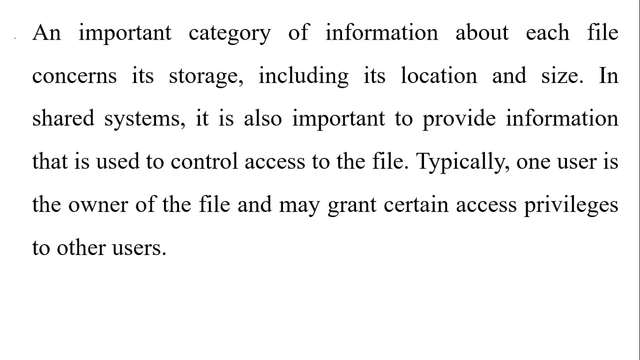 on disk. From the user's point of view, the directory provides a mapping between file storage and file storage. This is the date of the last update. Number nine is the date of the last update. This is the date of the last update. 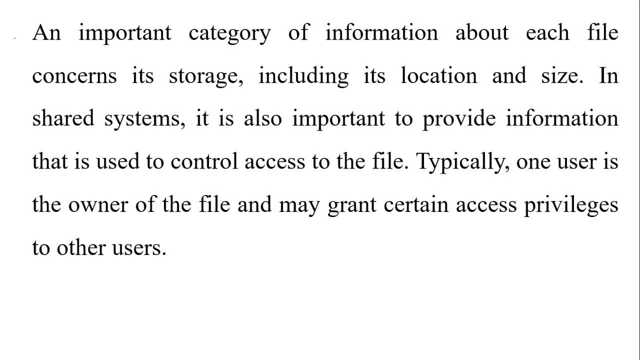 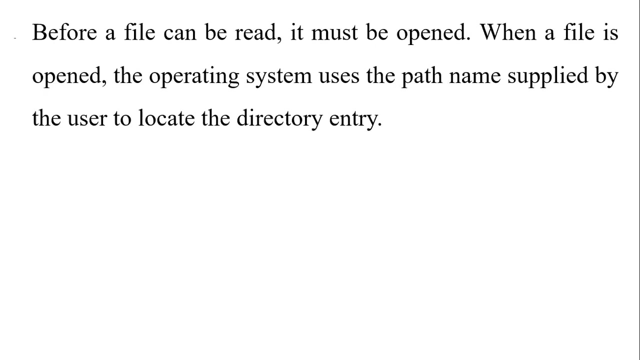 Number 10 shows the most common storage data in any directory. This is one of the most common storage data in the current storage of this domain Number. When a file can be read, it must be opened. When a file is opened, the operating system uses the path name supplied by the user to 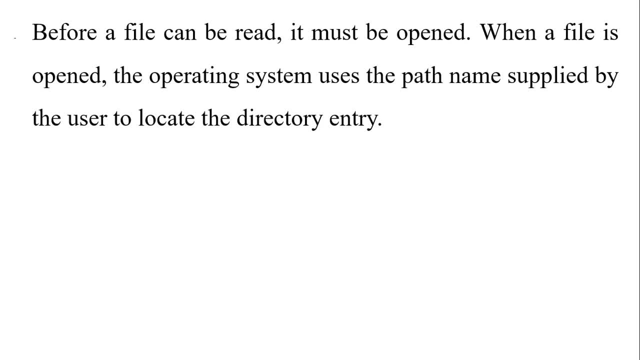 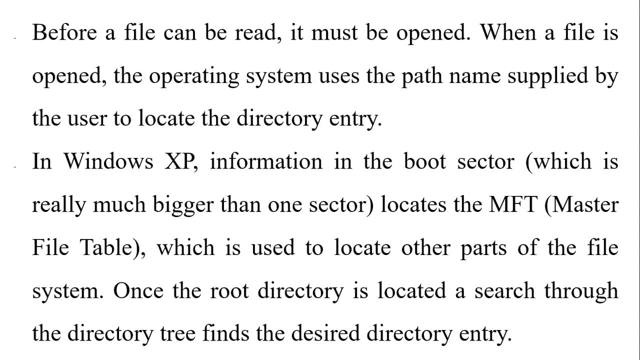 locate the directory entry. In Windows XP, for example, information in the boot sector, which is really much bigger than one sector, locates the MFT, that is, the master file table, which is used to locate other parts of the file system. 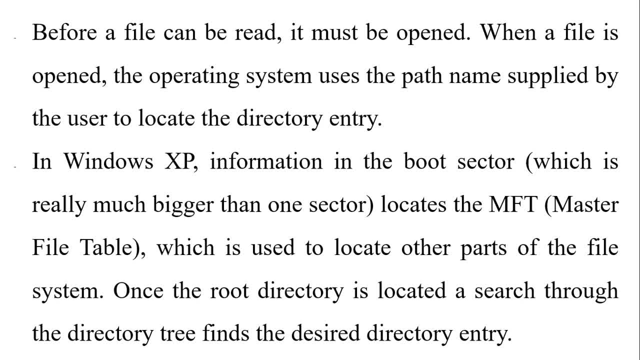 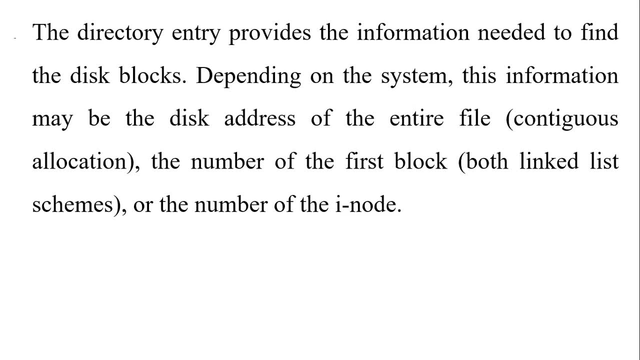 Once the root directory is located, a search through the directory tree finds the desired directory entry. The directory entry provides the information needed to find the disk blocks. Depending on the file system, this information may be in disk address of the entire file that is, contiguous allocation, the number of the first block, both the linked list schemes. 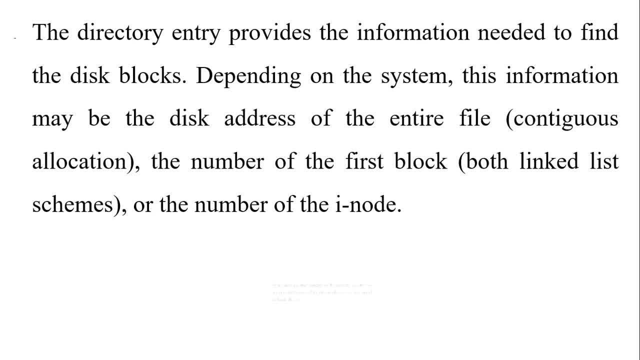 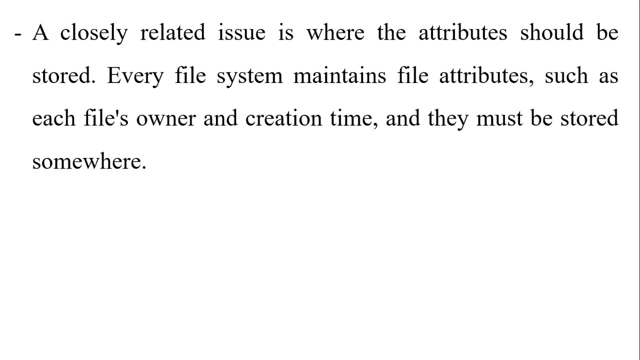 or the number of the inodes. In all cases, the main function of the directory system is to map the ASCII name of the file into or onto the information needed. A closely related issue is where the attributes should be stored. Every file system maintains file attributes, such as each file's owner and creation time. 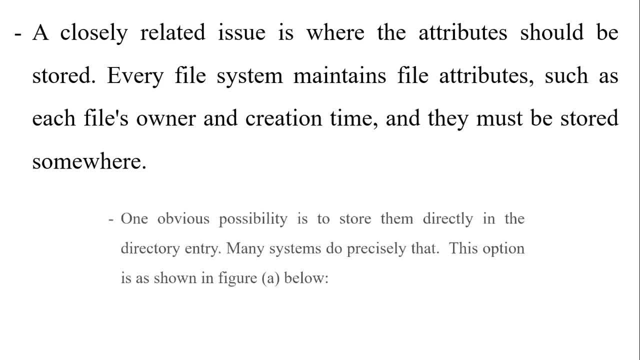 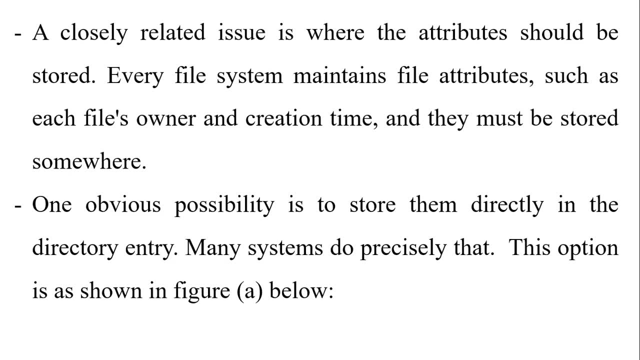 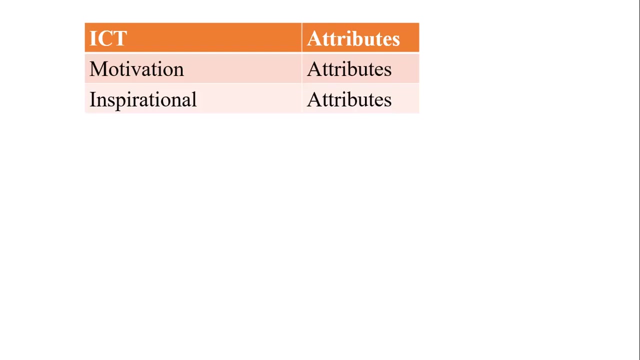 and they must be stored somewhere. One obvious possibility is to store them directly in the directory entry, Where, by many systems precisely do that. This option is as shown in this figure. In this method, we have each folder being stored together with its attributes. 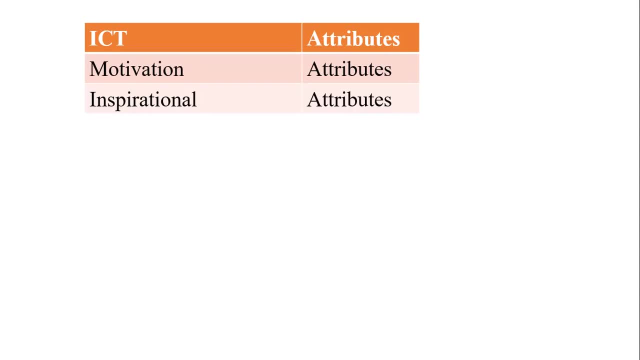 For example, in this case we have ICT and its attributes. The motivation and its attributes are stored. This is due to the fact that the L Woofer for that particular folder is stored on the inodeítulo. In other words, it is stored on the inodeítulo and it is stored on the inodeítulo. 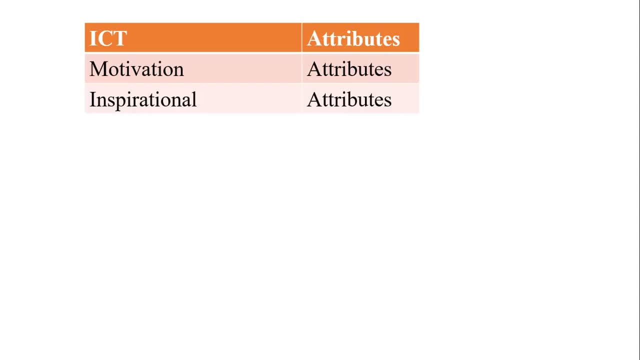 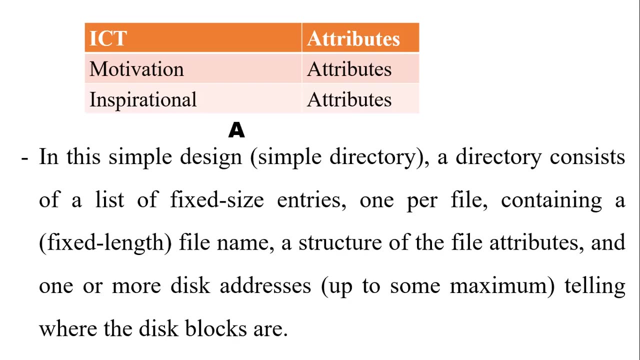 Therefore it is stored on the inodeítulo attributes, as well as inspirational and its attributes in this simple design or simple directory. a directory consists of a list of fixed size entries, one per file, containing a fixed length, file name, a structure of the file attributes and one or more disk addresses, up to some maximum telling where the disk blocks are. 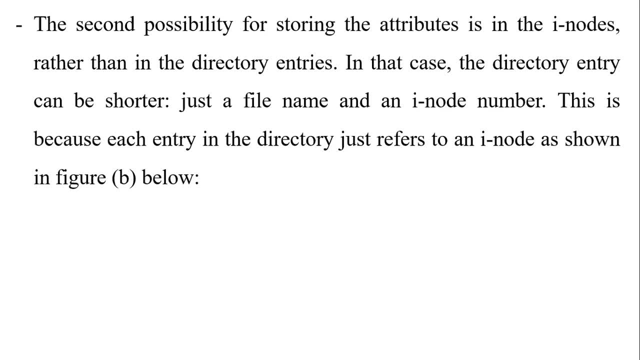 the second possibility for storing the attributes is in the idos rather than in the directory entries. in that case the directory entry can be shorter, just a file name and an id number. this is because it's not the same as the directory entry. entry in the directory just refers to an inode, as shown in the following figure. 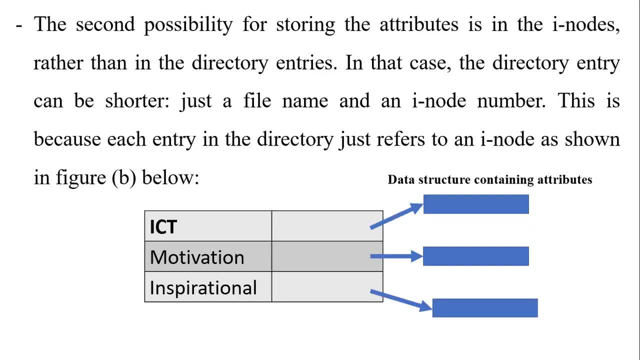 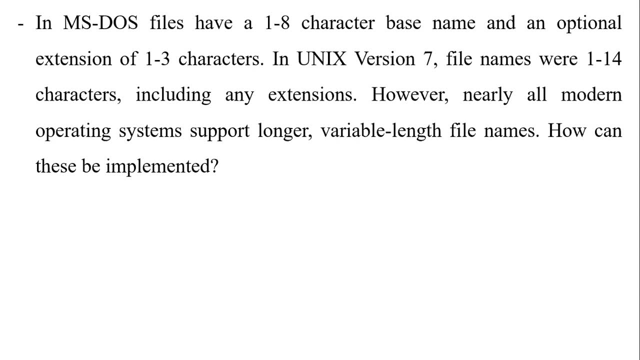 so in this case we have the attributes stored separately from the directory entries. in ms-dos, for example, files have a 1 to 8 name and an optional extension of 1 to 3 characters. in unix version 7, file names were 1 to 14 characters, including in extensions. however, nearly all the modern operating systems 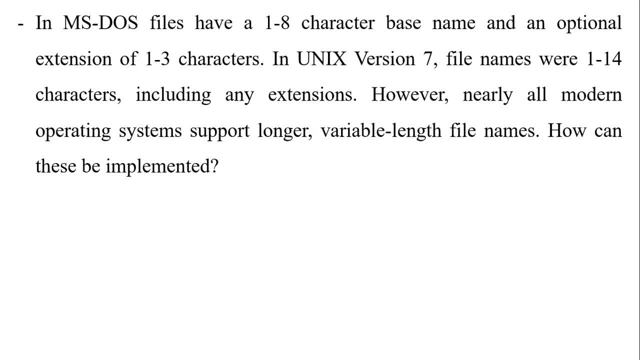 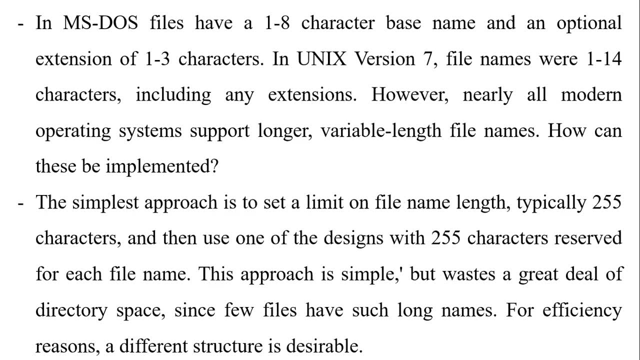 support longer variable length file names. so how can this be implemented? the simplest approach is to set a limit on file name length, which is typically 255 characters, and then use one of the designs with 255 characters reserved for each file name. this approach is simple, but with a great deal of directory space, since few files. 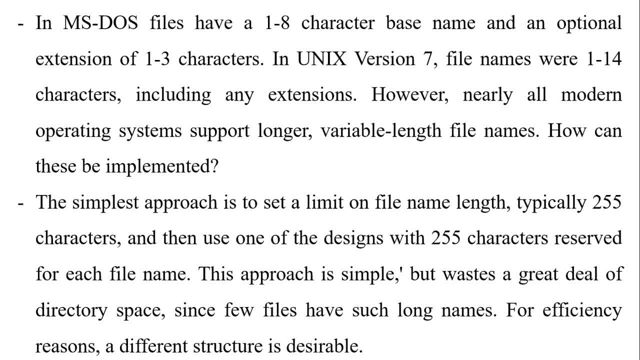 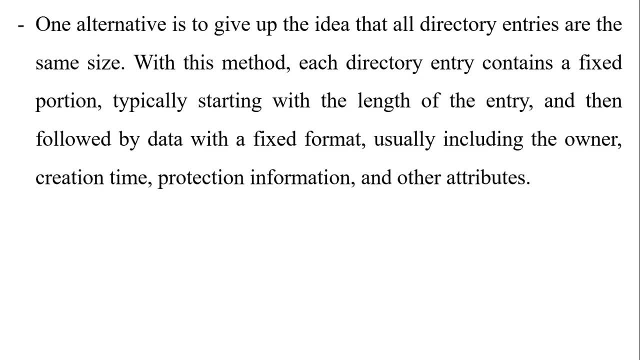 have such long names. for efficiency reasons, a different structure is desirable. one alternative is to give up the idea that all directory entries are the same size. with this method, each directory entry contains a fixed portion, typically starting with the length of the entry, and then followed by data with a fixed format, usually including the owner. 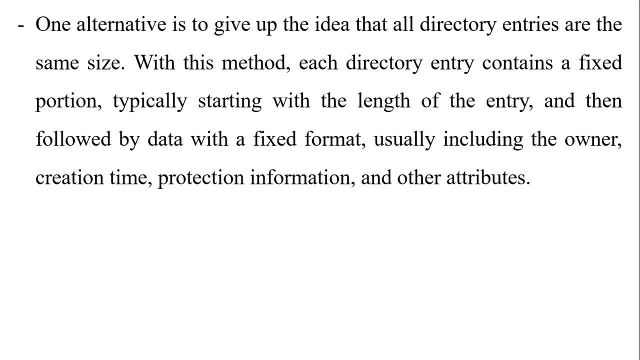 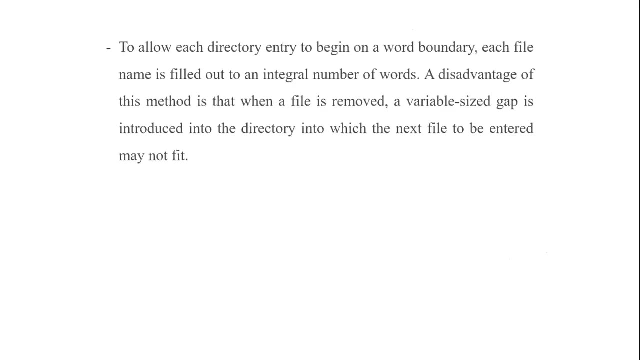 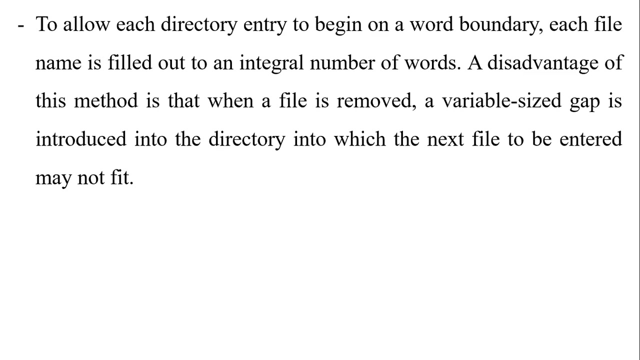 creation, time protection information and engine time name and other attributes. This fixed-length handler is followed by the actual filename, however long it may be. Each filename is determined by a special character, which is usually a zero, To allow each directory entry to begin on a one boundary. each filename is filled out. 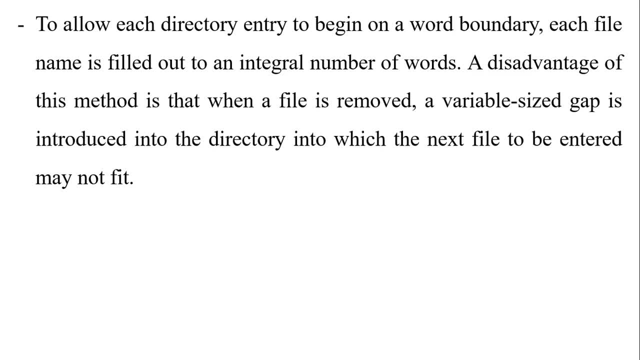 to an integral number of ones. A disadvantage of this method is that when a file is removed, a variable-sized gap is introduced into the directory into which the next file to be entered may not fit. Another problem is that a single directory entry may span multiple pages, so a page fault. 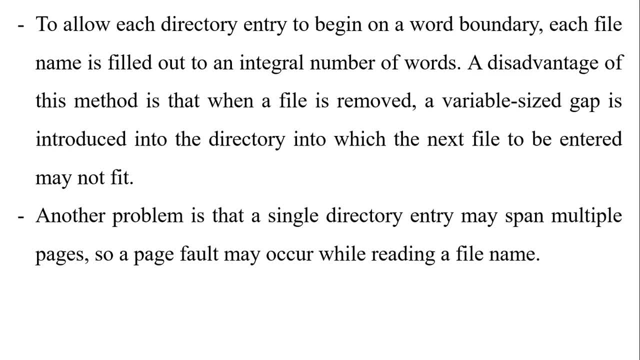 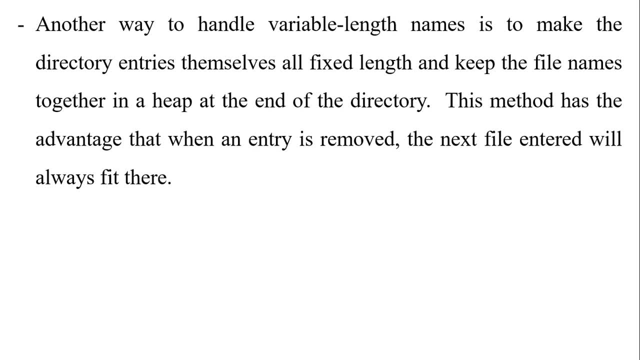 may occur. Another way to handle variable-length names is to make the directory entries themselves all fixed-length and keep the filenames together in a heap at the end of the directory. This method has the advantage that when an entry is removed, the next file entered will. 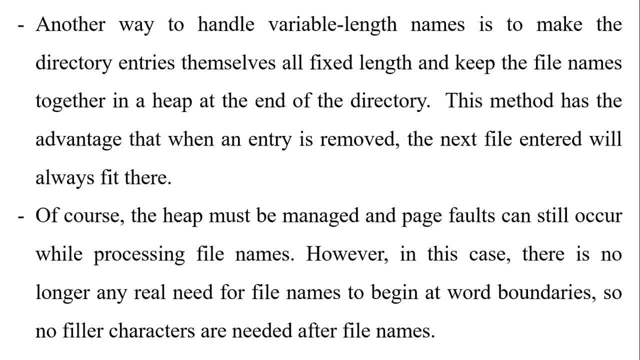 always fit there. Of course, the heap must be managed and page faults can still occur while processing filenames. However, in this case, there is no longer any real need for filenames to begin at one boundary, so no filler characters are needed after filenames. In all of these designs so far. directories are as follows: The first is the file name. The second is the file name. The third is the file name. The fourth is the file name. The fifth is the file name. The sixth is the file name. 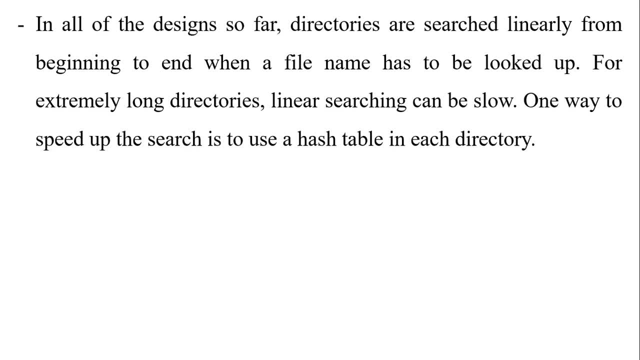 The sixth is the file name. The fifth is the file name. The sixth is the file name. The ninth isweis the value behind thewhich kinds of page faults and the length of the entries requires Any trace value will be most of them. 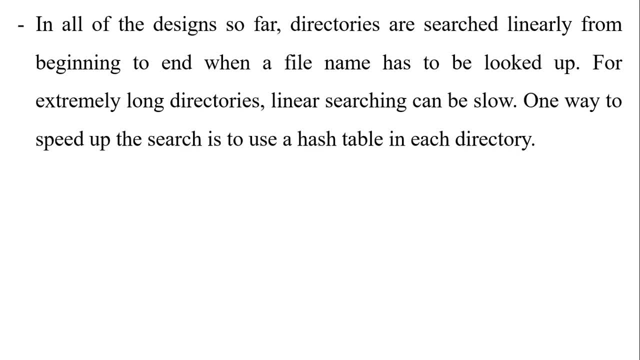 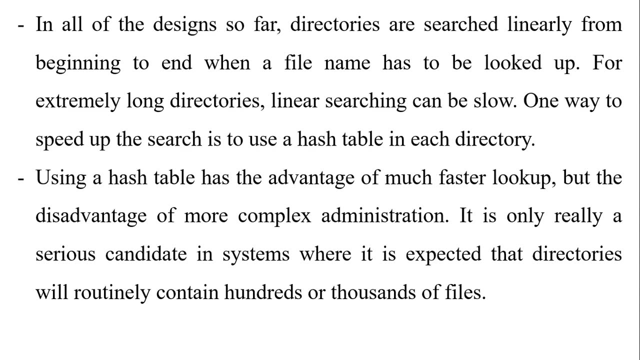 The output can be searched linearly from beginning to end. when a file name has to be looked up For extremely long directories, linear searching can be slow. One way to speed up the search is to use a hash table in each directory. Using a hash table has the following advantage of much faster look up, but the disadvantage 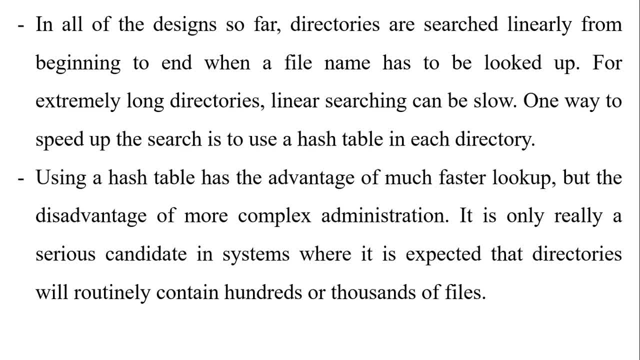 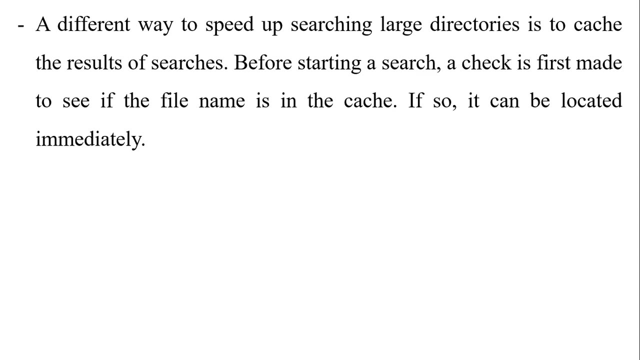 administration. It is usually, or it is only really, a serious candidate in systems where it is expected that directories will routinely contain hundreds or thousands of files. A different way to speed up searching large directories is to cache the results of searches. I repeat: a different way to speed up searching large directories is to cache the results of 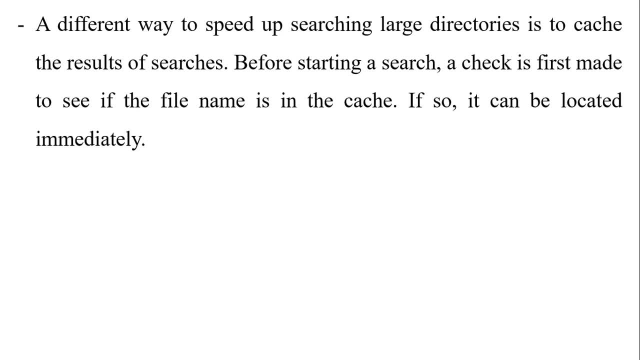 searches. Before starting a search, a check is first made to see if the file name is in the cache. If so, it can be located immediately. Of course, caching only works if a relatively small number of files comprise the majority of the lookups. The following are brief explanations of how. 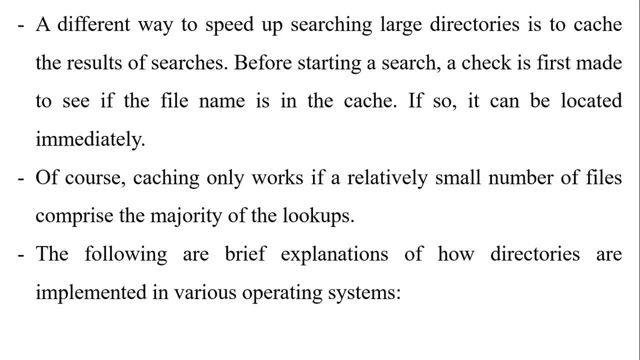 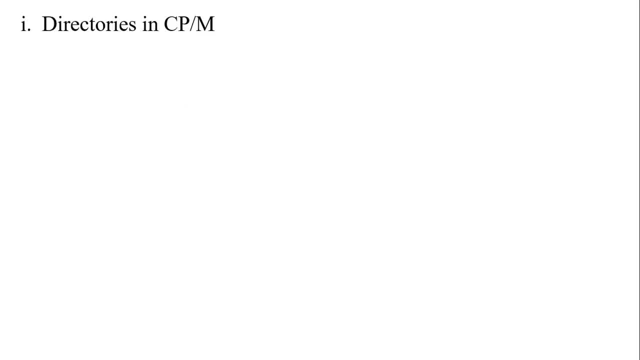 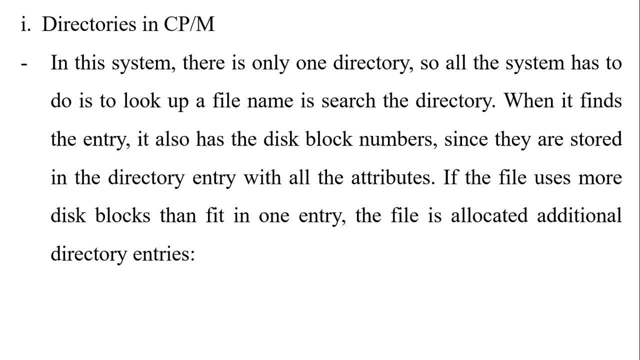 directories are implemented in various operating systems. We start with looking at directories in CP, stroke M. In this system there is only one directory. so all the system has to do is to look up a file name in the search directory. Or, in this system, there is only one directory. 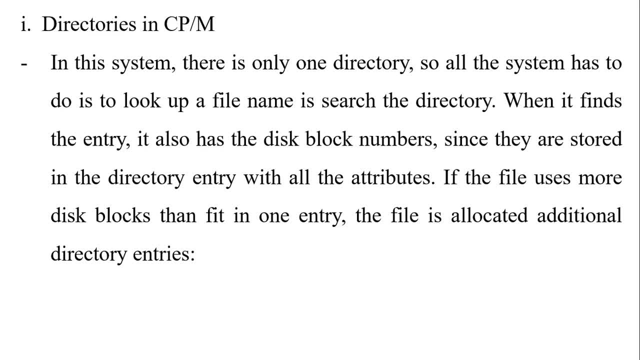 and therefore all the system has to do is to look up a file name in the search directory. When it It defines the entry, it also has the disk block numbers, since they are stored in the directory entry with all the attributes. If the file uses more disk blocks than can fit in one entry, the file is allocated additional directory entries. This is how. 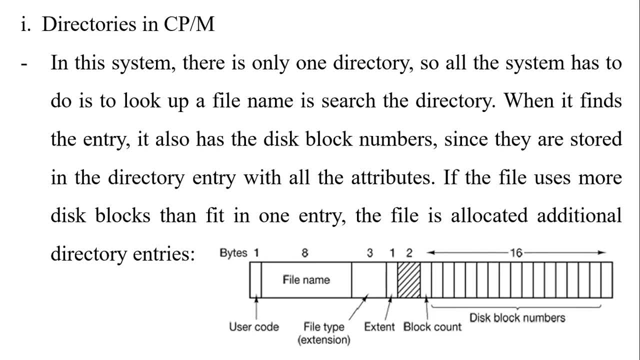 the directories in CPM are allocated. From this diagram, my dear students and the rest of the learners, you can see that we have one byte reserved for the user code, eight bytes reserved for the file name, 3 reserved for the file type or extension. 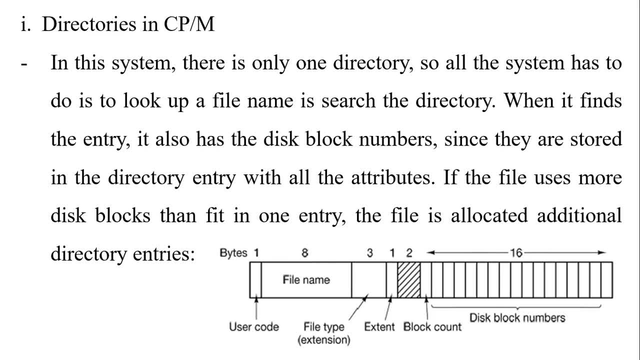 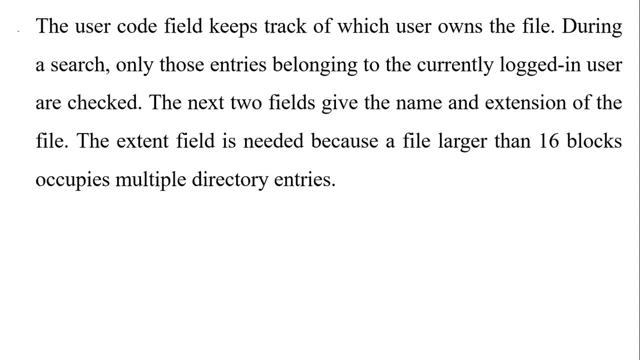 1 reserved for extent, 2 bleibt reserved for trademarks and so on are left as the gap. Then we have the block count and these blocks span across several blocks, Like in this case, we have 16 disk blocks. The user code field keeps track of which user owns the file During a search. 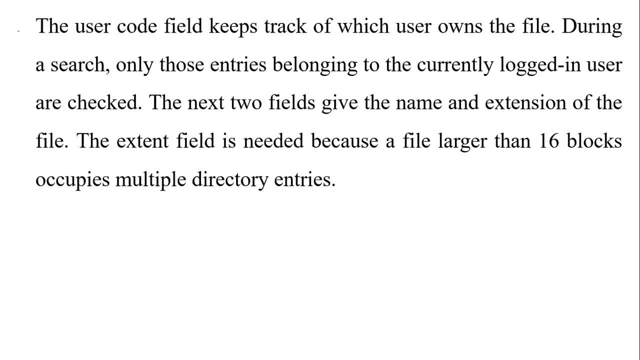 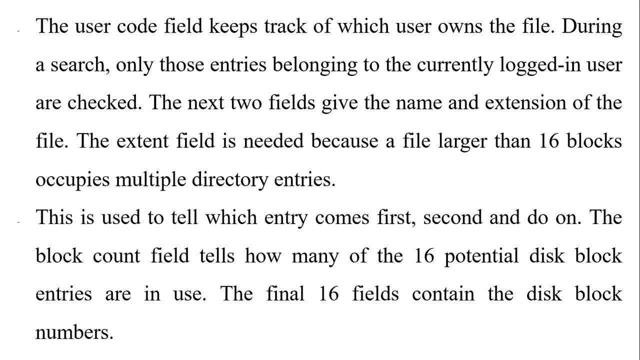 only those entries belonging to the currently logged in user are checked. The next two fields give the name and extension of the file, while the extend field is needed because a file larger than 16 blocks occupies multiple directory entries. This is used to tell which entry comes first. 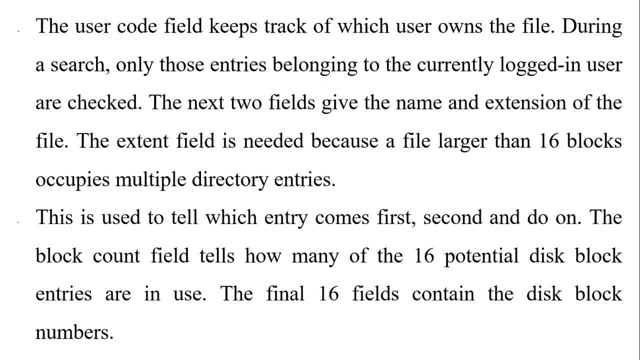 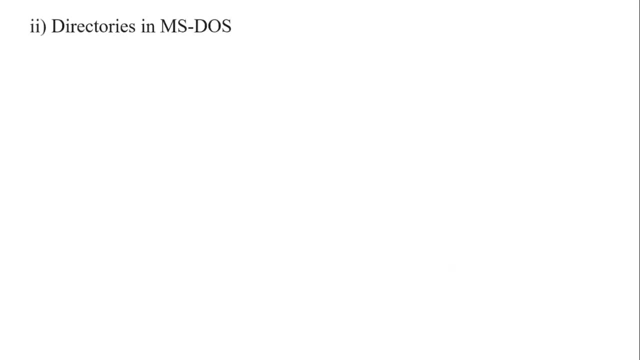 second and do and so on. The block count field tells how many of the 16 potential disk block entries are in use. The final 16 fields contain the disk block numbers, just as I have already mentioned. The other is directories in ms-dos. 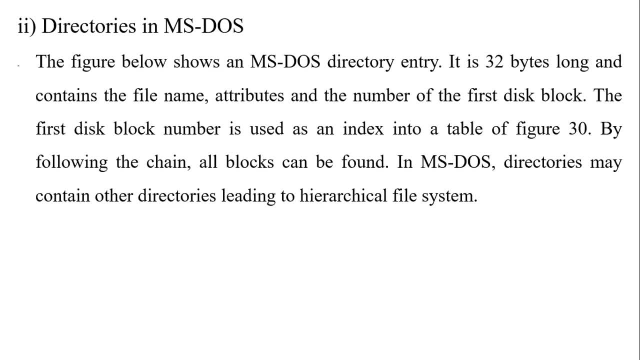 The figure below shows an MS-DOS directory entry. It is 32 bytes long and contains the file name, in this case, whose length is 8 bytes, the attributes and the number of the first disk block. The first disk block number is used as an index into a table of figure 30.. 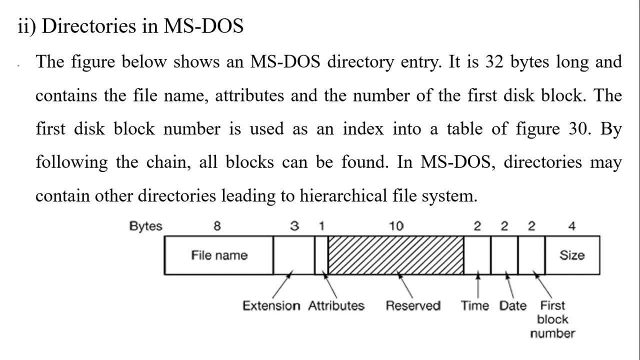 By following the chain, all blocks can be found In MS-DOS. directories may contain other directories leading to a hierarchical file system And therefore this is illustrated as follows. And therefore, my dear students and the rest of the learners, you can see that when information 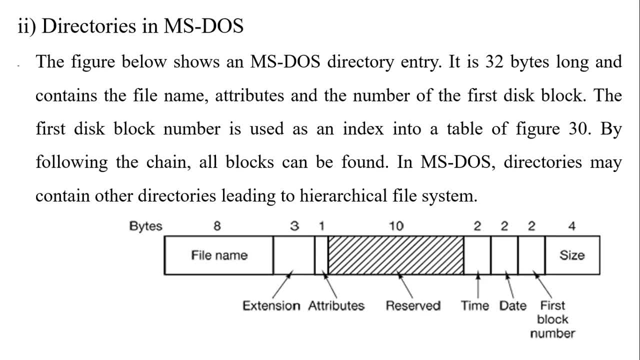 or a directory is created in MS-DOS, a number of information is kept or is stored. This information includes a file name whose number of bytes are normally eight. in maximum. Three is used for extension, One For attributes, Ten are reserved. 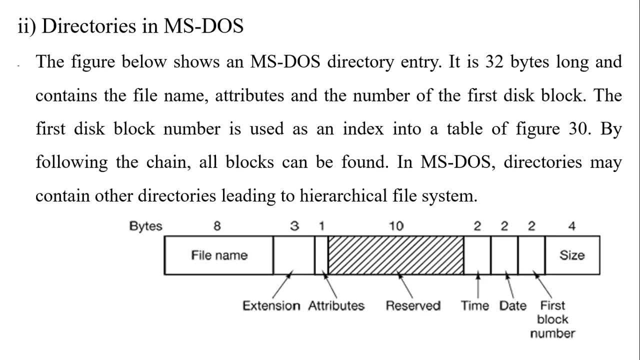 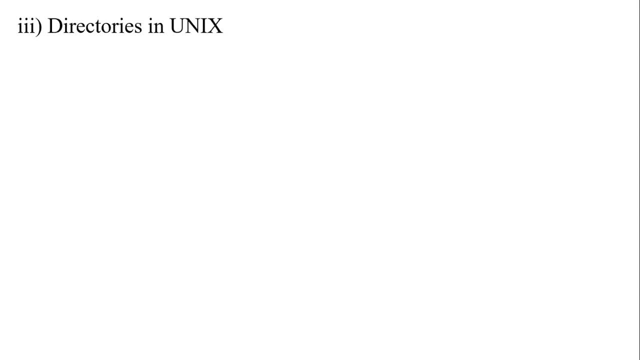 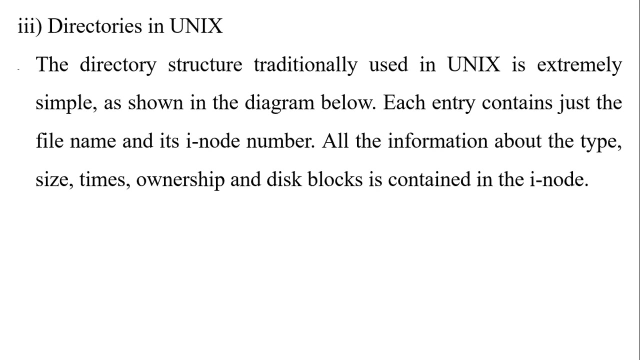 While two are for time, Two are for date, Two are for the first block number And four is for the size. Number three is directories in Unix, The directory structure traditionally used in Unix. The diagram is extremely simple, as shown in the diagram below. 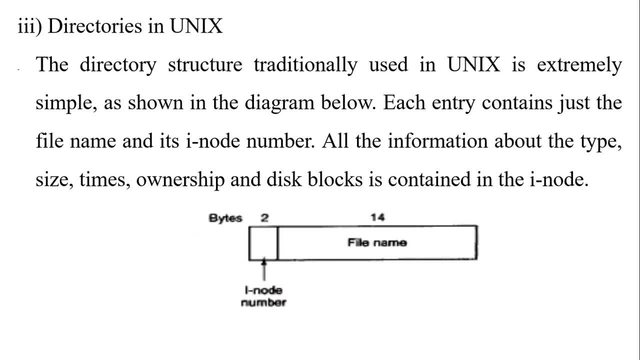 Each entry contains just the file name and its I-node number. All the information about the type, the size, the times, the ownership and disk blocks is contained in the I-node And therefore from this diagram you will see that the directory structure is very simple. 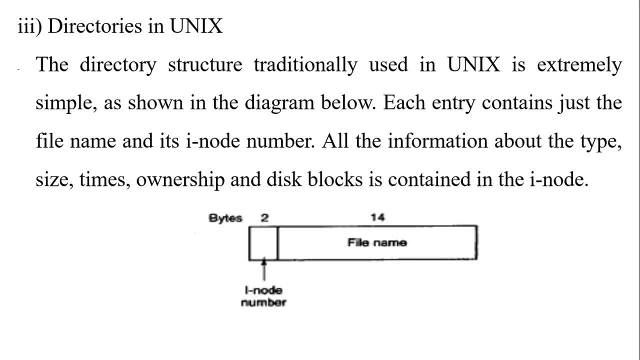 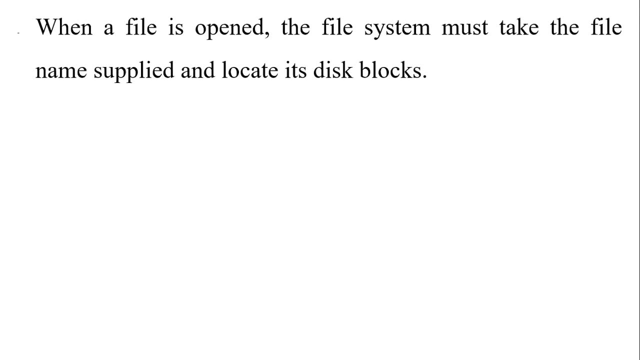 In this diagram you can see that we have two bytes that are normally reserved for the inode number and 14 bytes are reserved for the file name. When a file is opened, the file system must take the file name supplied and locate its disk blocks. 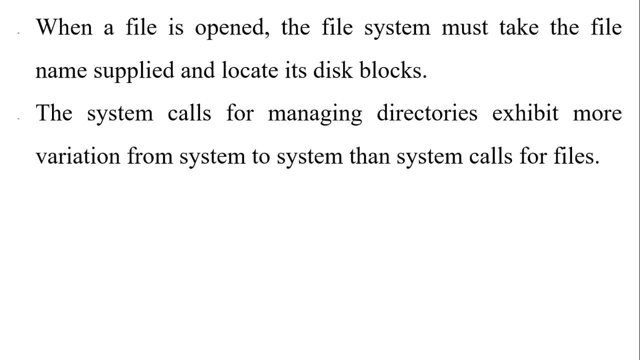 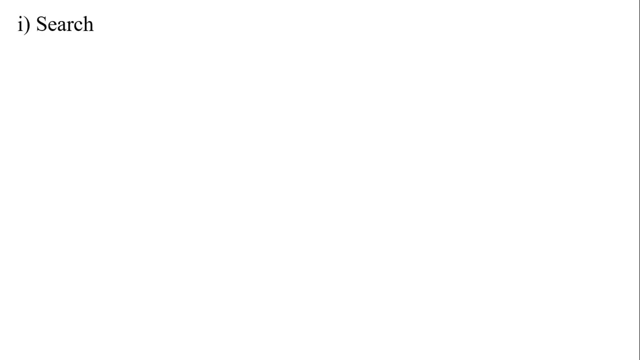 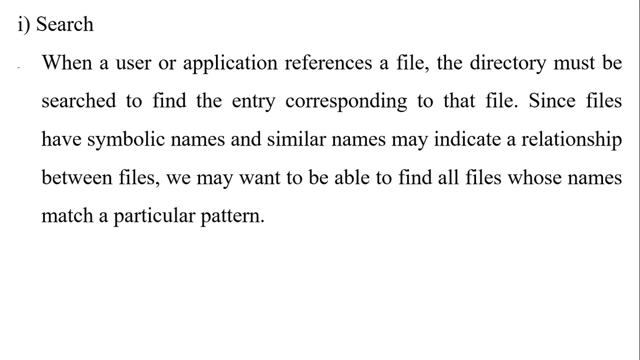 The system calls for managing directories exhibit more variation from system to system than system calls for files. The following are the main types of operations or system calls that may be performed on a directory. Number one is a search operation. When a user or application references a file, the directory must be searched to find the entry corresponding to that file. 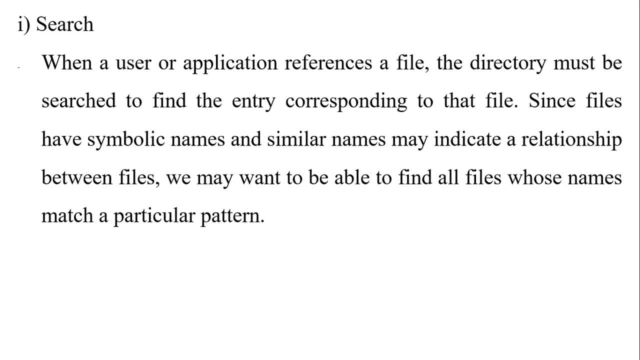 Since files have symbolic names and similar names may indicate a relationship between files, we may want to be able to find all the files whose names match a particular pattern. Number two: a search is create. Number two: A search is create. It is used to create a new directory. 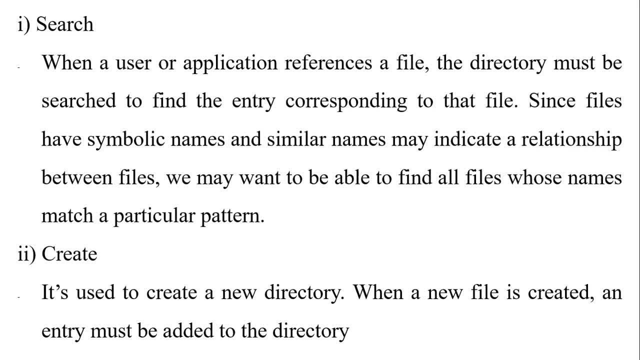 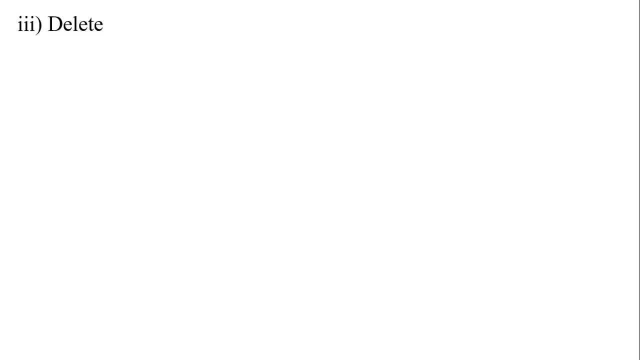 When a new file is created, an entry must be added to the directory. Number three is delete. It is used to remove a directory from a large storage medium. Only an empty directory can be deleted. When a file is deleted, an entry must be removed from the directory. 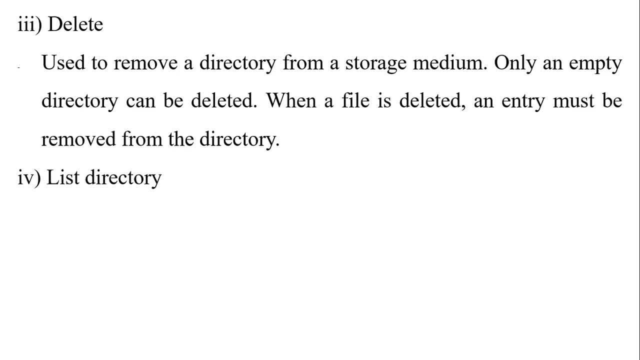 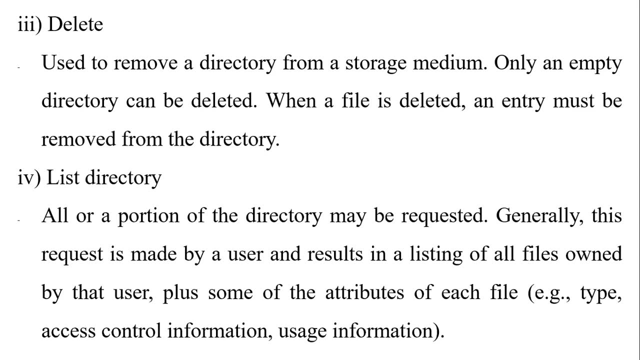 Number four is list directory. All or a portion of the directory may be requested. Generally, this request is made by a user and results in a listing of all the files, In a listing of all the files owned by that user, plus some of the attributes of each file. 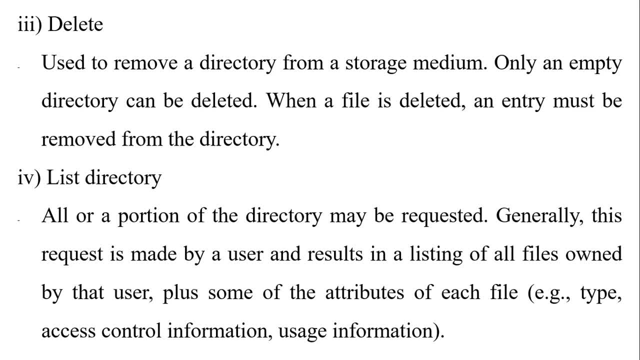 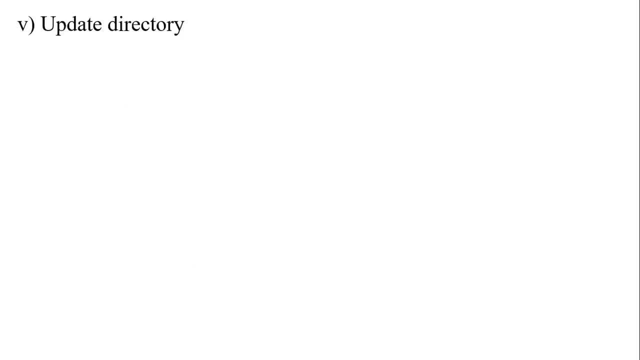 For example, the type, access, control information and usage information. Number five is update directory or update directory, Because some file attributes are stored in the directory. a change in one of these attributes requires a change in the corresponding directory entry. Number six is open directory. 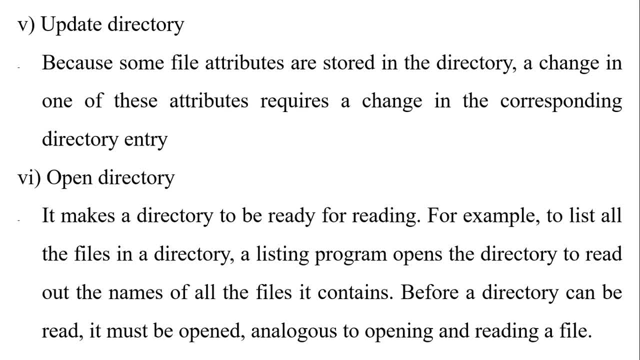 It makes a directory to be ready for reading. For example, to list all the files in a directory, a listing program opens the directory In order to read out the names of all the files that it contains. Before a directory can be read, it must be opened, analogous to opening and reading a file. 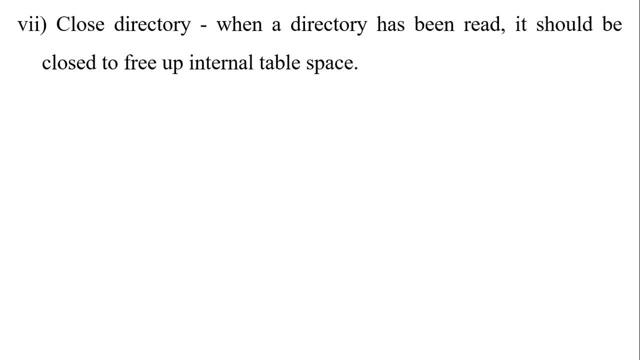 Number seven is close directory. When a directory has been read, it should be closed in order to free up the directory. When a directory has been read, it should be closed in order to free up the directory. When a directory has been read, it should be closed in order to free up the internal table space. 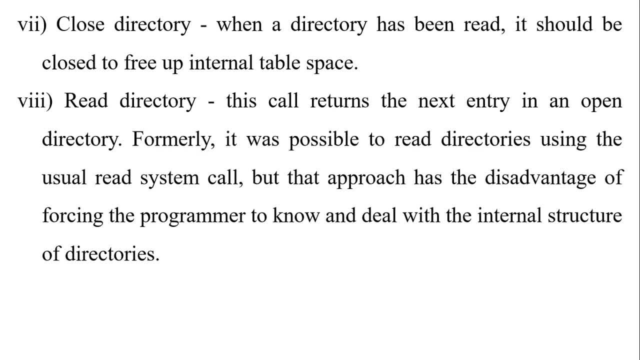 Number eight is read, or what we just call or refer to as read directory. This call returns the next entry in an open directory. Formerly it was possible to read directories using the usual read system call, But that approach has the disadvantage of forcing the program to read the directory. 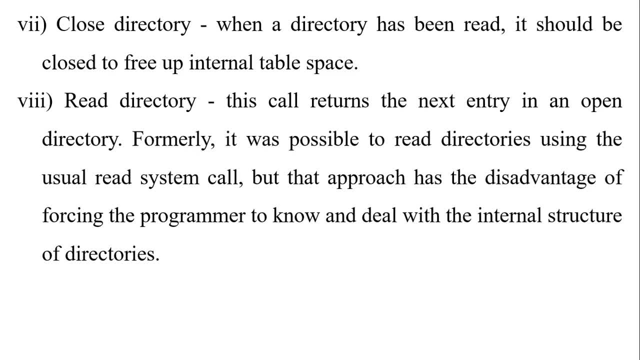 But that approach has the disadvantage of forcing the program to read the directory And forcing the programmer to know and deal with the internal structure of directories. Number nine is rename. In many respects directories are just like files and can be renamed the same way files can be. 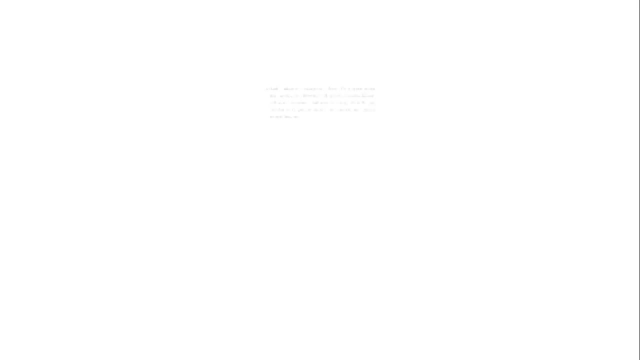 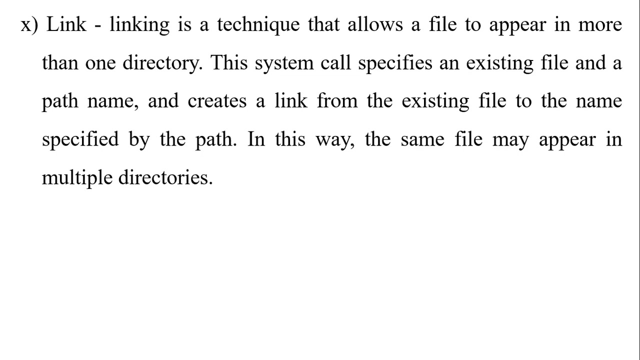 Number ten is link. link Linking is a technique that allows a file to appear in more than one directory. This system call specifies an existing file and a path name and creates a link from the existing file to the name specified by the path. In this way, the same file may appear in multiple directories. 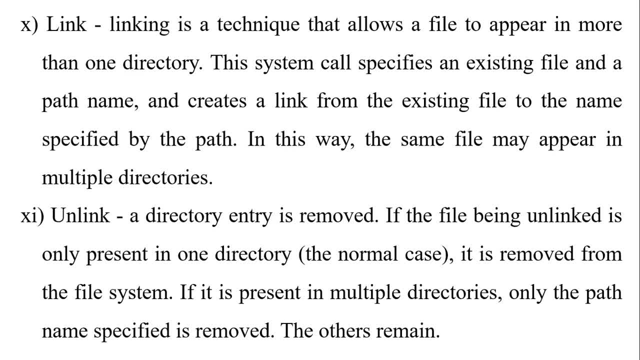 Number 11 is Unlink. A directory entry is removed If the file being unlinked is only present in one directory- the normal case, or which is usually the normal case- it is removed from the file system. If it is present in multiple directories, only the path name specified is removed. 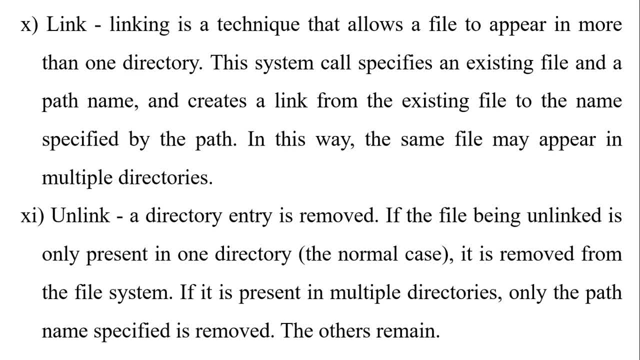 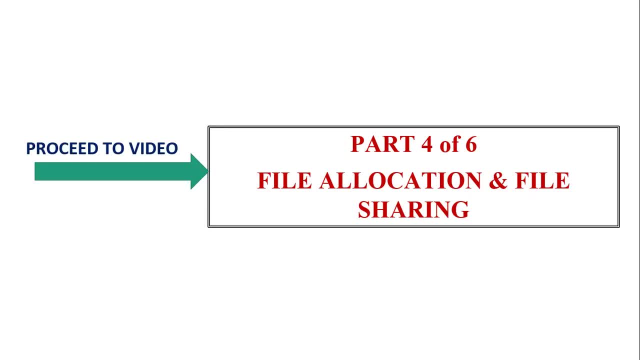 The others remain. We have come to the end of part 3 of the series of videos in this topic on file management. You can now proceed and listen to and watch part 4 of the 6 part series of videos in this topic by the title: File Allocation and File Sharing. 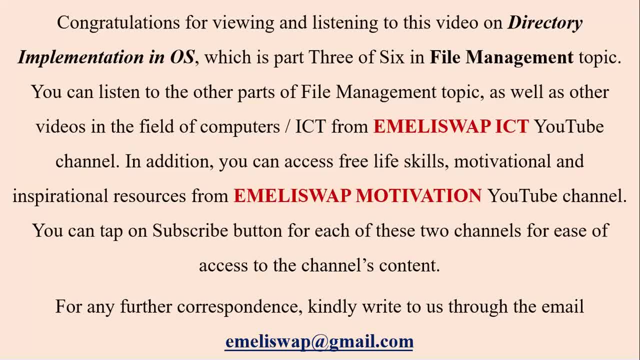 Congratulations for viewing and listening to today's video on Directory Implementation in Operating Systems, which is part 3 of the 6 part series of presentations in file management topic. Please subscribe to the channel and press the bell icon to get notified of future videos. You can listen to the other parts of file management in the rest of the series of videos. and you canlog in to the bottom of the screen. You can also listen to the style topics in the video description. I hope this video was useful. Thank you, Bye bye, Bye, bye. Share file management topic. by the title: file allocation and file sharing. Congratulations for viewing and listen to this video on directory implementation in operating systems, which is part 3 of the 6 part series of file management topic. You can listen to the other parts of file management topic. 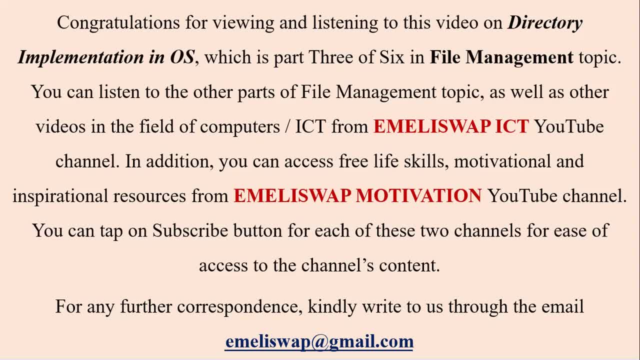 the topic, as well as other videos in the field of computers or ict from ml swap ict youtube channel. in addition, you can access free life skills, motivational and inspirational resources from ml swap motivation youtube channel. you can tap on subscribe button for each of these two.